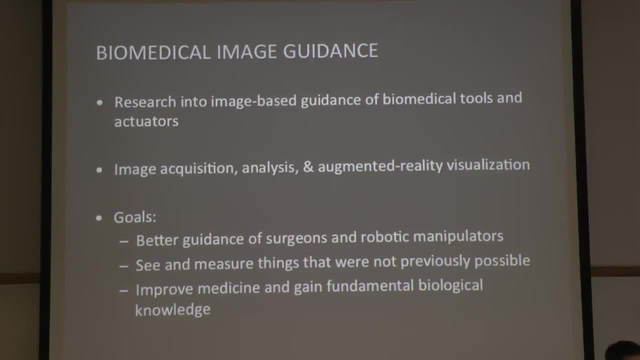 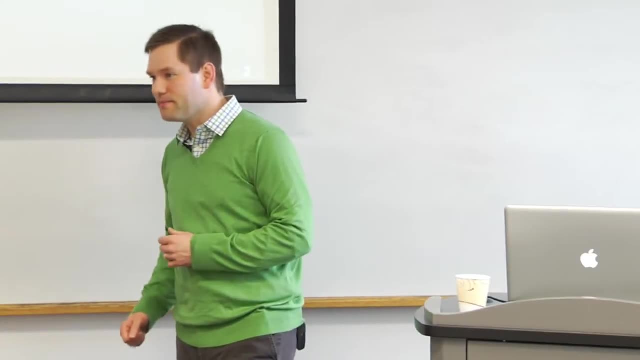 And this covers everything from image acquisition to biomechanical research. And this covers everything from image acquisition to biomechanical research. This covers everything from software acquisition and improvement, new developments in those technologies, Image analysis, computer vision kinds of things, And also augmented reality visualization. 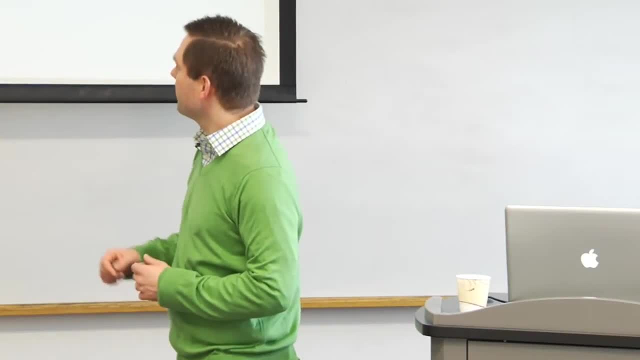 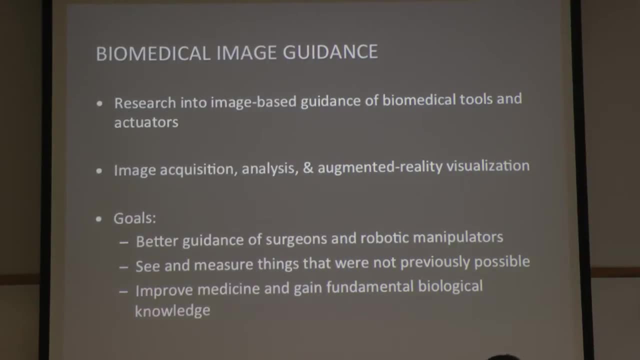 The goals of this are certainly first and foremost, in many ways, To give better guidance to surgeons and better guidance to robotic manipulators. But, going beyond that, I'd like to see and measure things that were not previously possible Working in the core imaging technologies themselves. 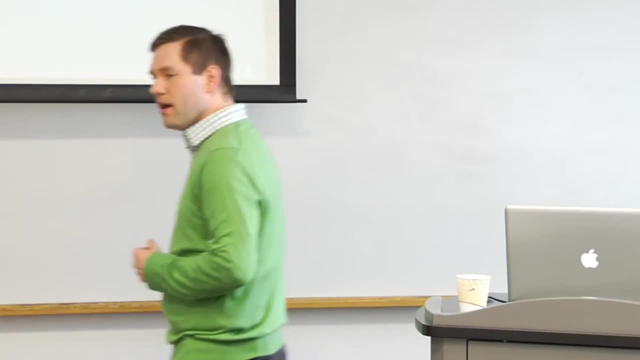 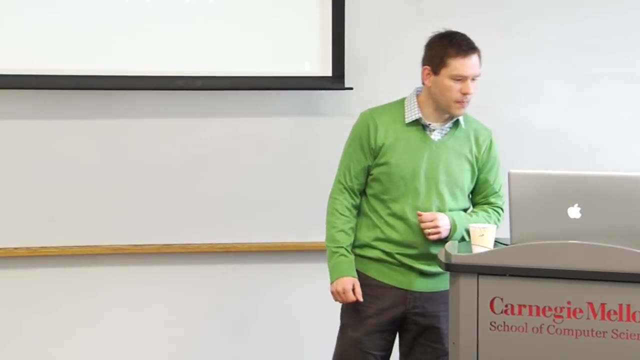 And to go with that, to then be able to improve technologies in the complex, throughout robotics and others, to improve medicine and gain fundamentally new biomedical knowledge. So that's where I'm going with this. Doing image guidance does pose some unique requirements. Real-time operation is one of those. 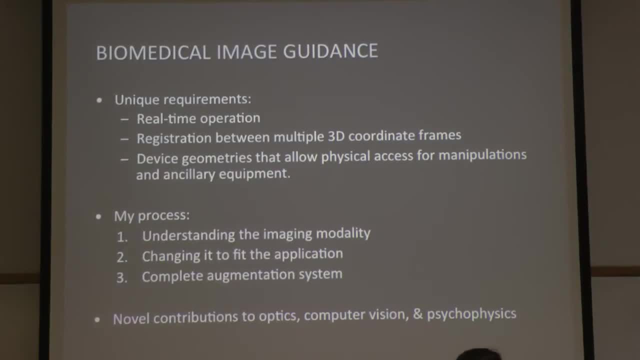 There's lots of things we do in computer vision and medical image analysis that work really well. if you have a cluster of computers and two hours for them to operate, Lots of things that work reasonably well. if you have five minutes on a desktop, Most of those don't work so well. 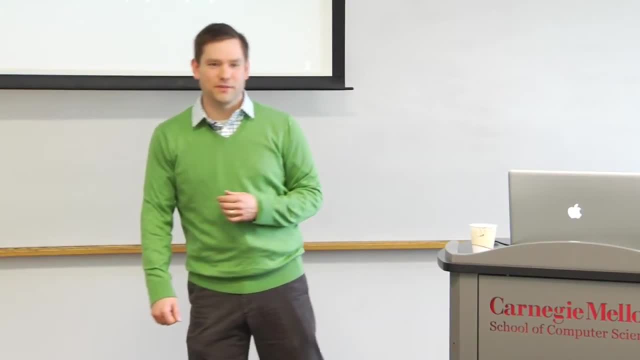 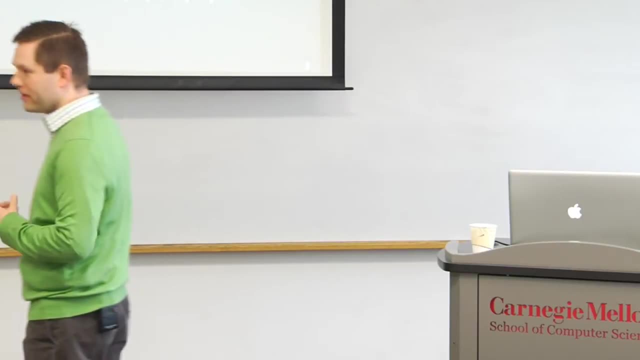 if you want them to run at 15, 30 frames a second. on real-time data stream, There is a much tighter requirement for registration between multiple 3D coordinate frames And unfortunately, patients are soft and squishy. Most things we want to do. 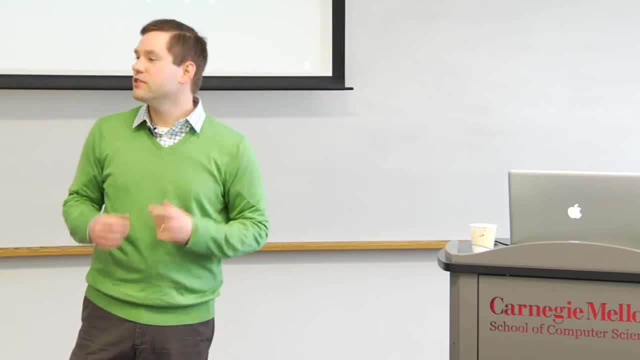 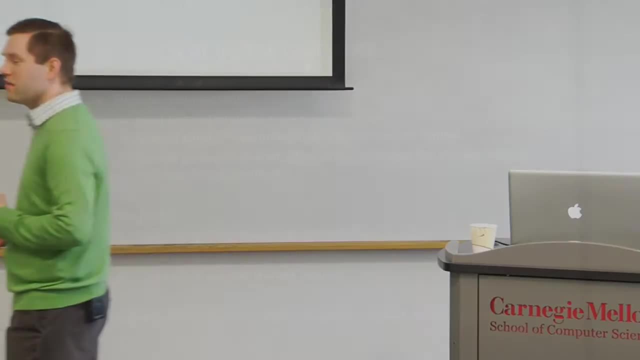 especially if we're not talking about orthopedic surgery- involve soft tissues that are deformable, And so what registration means in that context itself is complicated. Deformable registration is usually not something we think of as real-time, And there are complicated issues here. 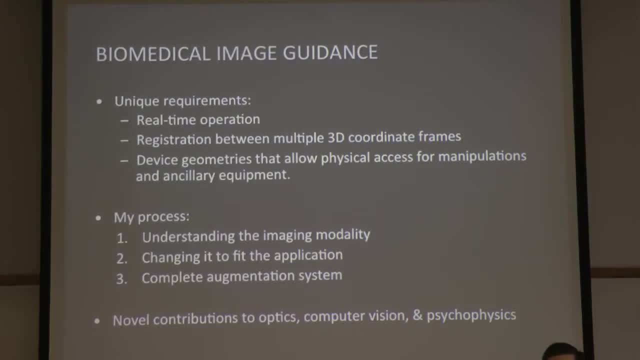 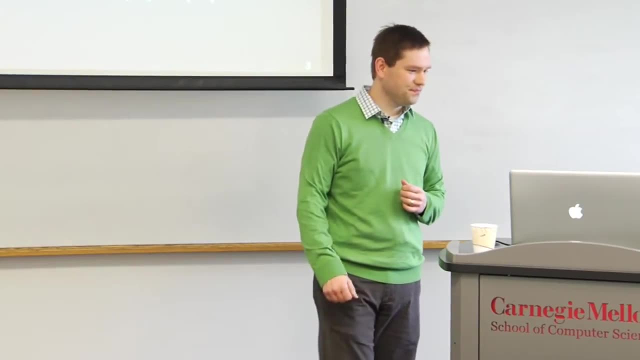 to deal with as we try to maintain the level of registration and alignment needed to safely guide tools to small targets, with dangerous things sitting right beside them that we don't want to injure. Finally, in all of this, we have to develop devices that have geometries that are actually usable. 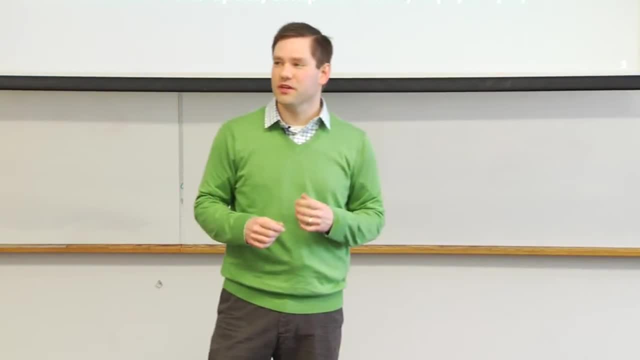 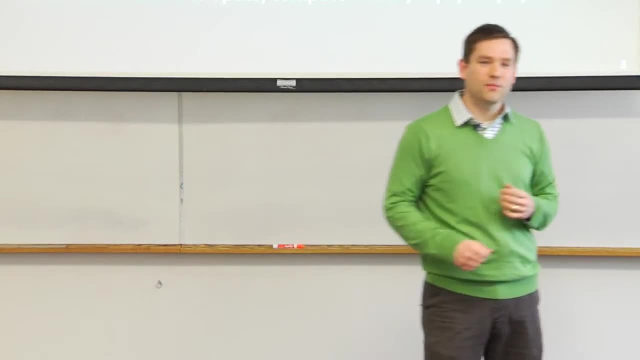 We can't have our tools sitting right in the way of the patient, for the surgeon can no longer get to where they need to get, And often this results in forcing us to do compromises. We have to work to make those compromises acceptable. 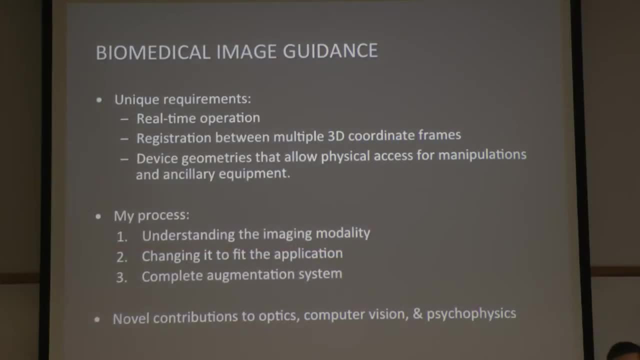 And see what we need to see, guide what we need to guide and still stay out of the way so that things can proceed. My core process in a lot of the work that I do is to begin with understanding the imaging modality at a sufficiently fundamental level. 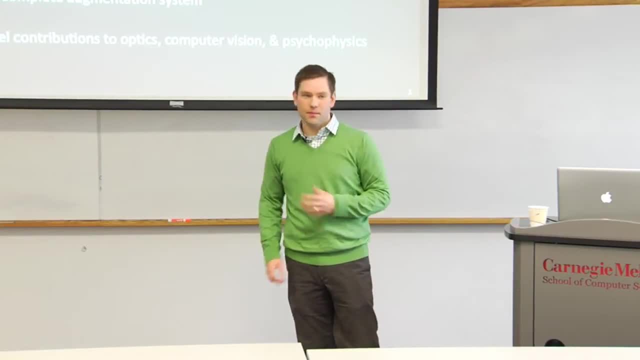 that I can change it and modify it as appropriate to be able to make the system work as a whole. I then change as I said, changing it to fit the application, and then I proceed from that to develop the entire system, an augmented reality system in many cases. 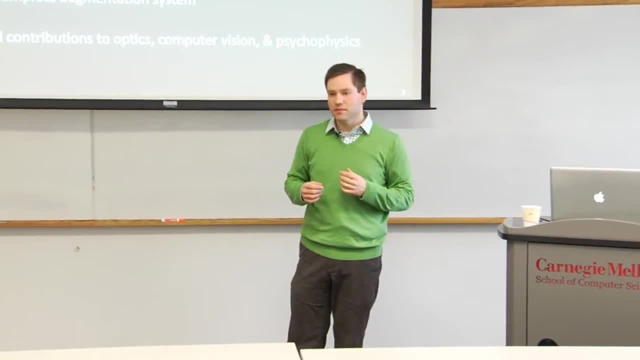 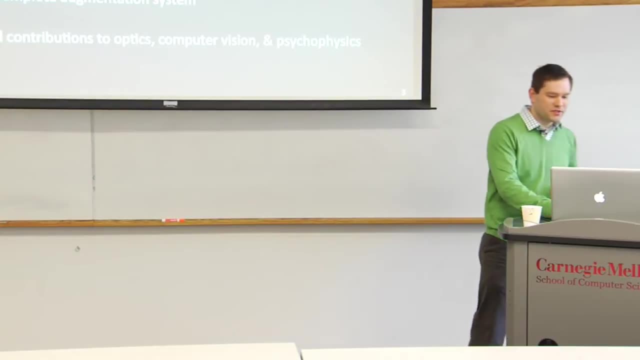 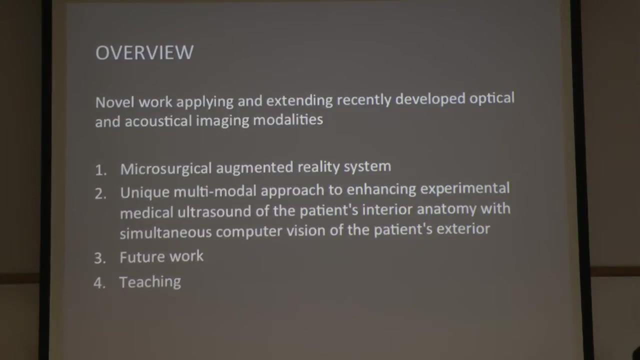 or some kind of another perceptual and guidance system, but ultimately giving new forms of vision to humans and computers. And this work entails novel contributions to optics, computer vision and psychophysics. So I'm going to, in this talk, begin by presenting two different systems that I'm working on. 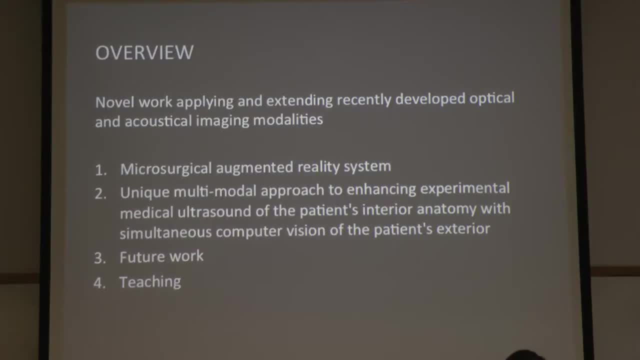 The first that'll be the imaging modality, The second that'll be the imaging modality And the third that'll spend the majority of the time on is work for the R01 that Howie mentioned, And this is in progress: developing a microsurgical augmented reality guidance system. 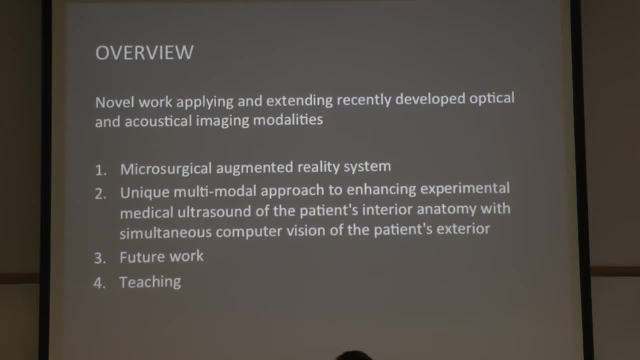 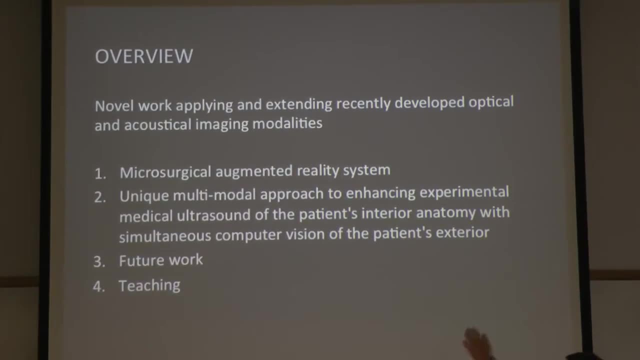 I will then talk next about the system that's just starting, And this is a system for which we're grading the DOD award, And this is for a multimodal approach to enhance clinical ultrasound with computer vision, so that the ultrasound probe will know where it is located relative to the patient themselves. 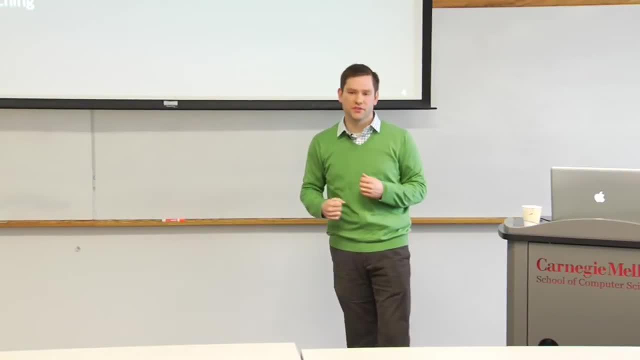 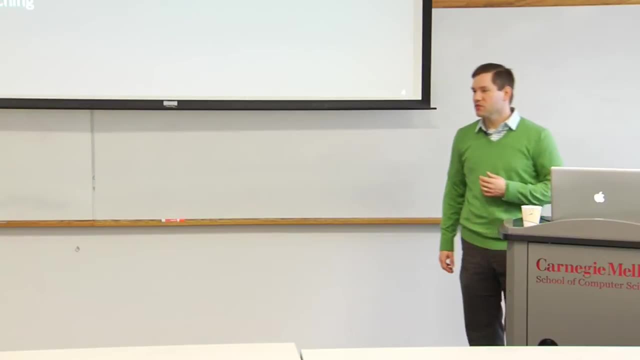 without need for a clinical ultrasound, And this is for third-party tracking able to hand deformation of the patient, and so on. I'll then discuss a little bit about my future research directions and finally have a couple of slides about the teaching that I do as well, before wrapping up. 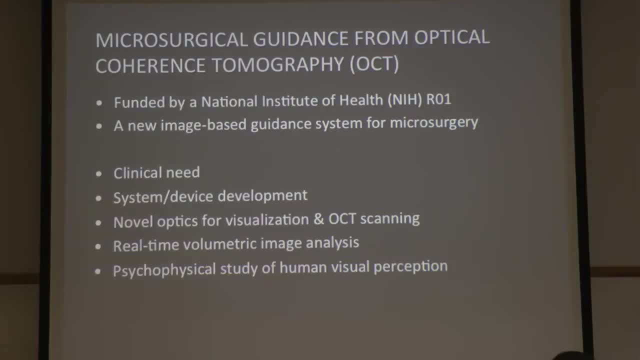 Our microsurgical guidance work uses optical coherence tomography, OCT, to guide microsurgery, And this was funded by the National Institute of Health's Eye Center with the application of guiding optimization of optical hojeology in the lens of the patient's eye. 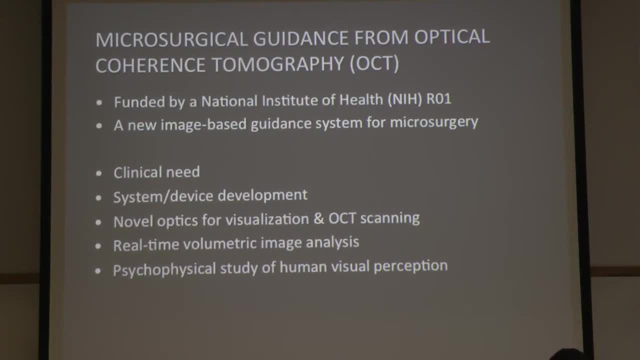 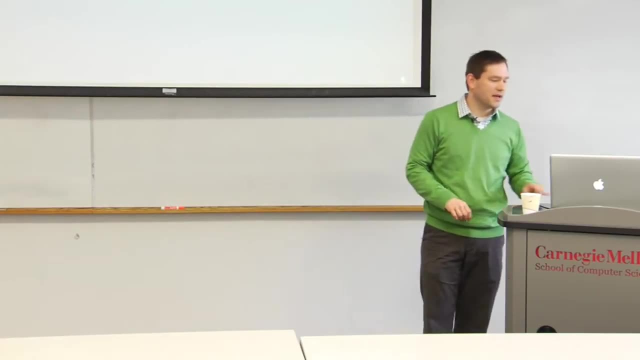 And for clinical treatment. we're doing ophthalmology surgery and in particular on the anterior segment of the eye, which is the front portion of it, So cornea, lens, that kind of stuff. This is not for retinal surgery yet. 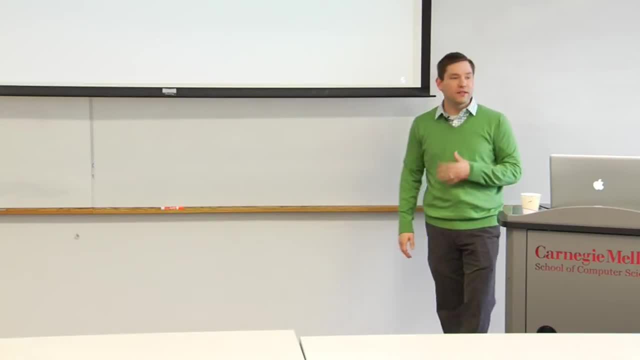 That's future work yet to happen. In describing this, I'm going to talk some about the clinical needs and what we're trying to do here. I'll talk about the general development of the system. Proceed to describing the novel optics work that was done. 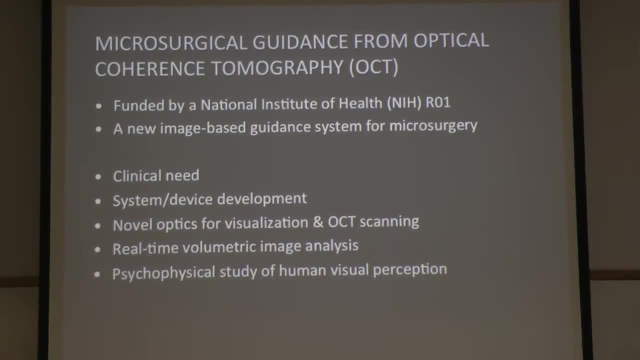 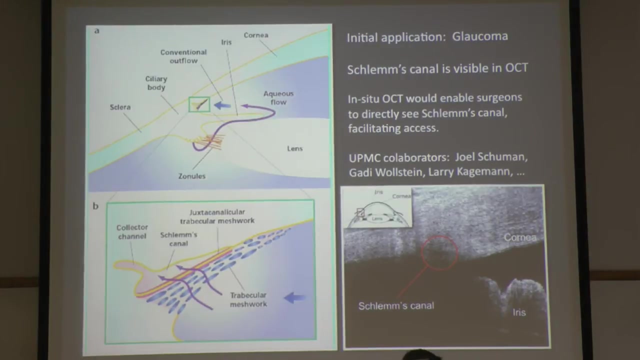 in terms of the scanner and in terms of the visualization aspects, talk a little bit about real-time image analysis and, finally, talk about psychophysics and understanding how humans perceive these images under a microscope, which, it turns out, is complicated. Our initial application for this work is treating glaucoma. 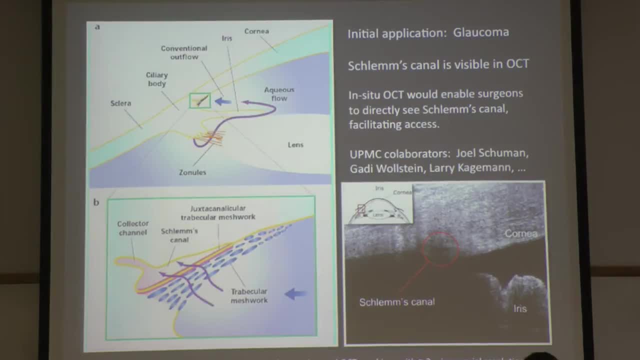 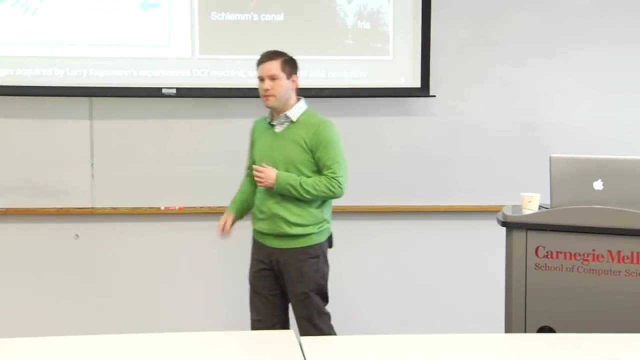 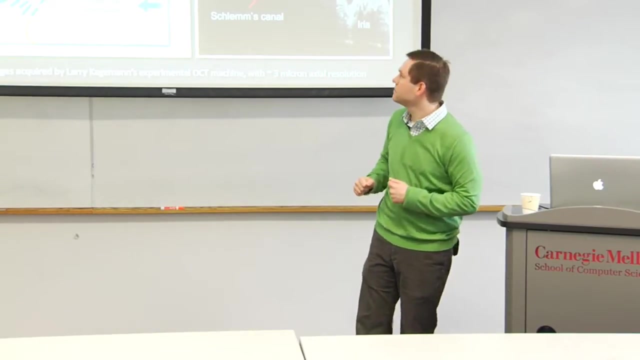 which is the second leading cause of irreversible blindness worldwide. Glaucoma is believed to be, with strong but not conclusive evidence, caused by increased intraocular pressure, And we do know that reducing pressure in the eye does correlate with positive outcomes in glaucoma patients. 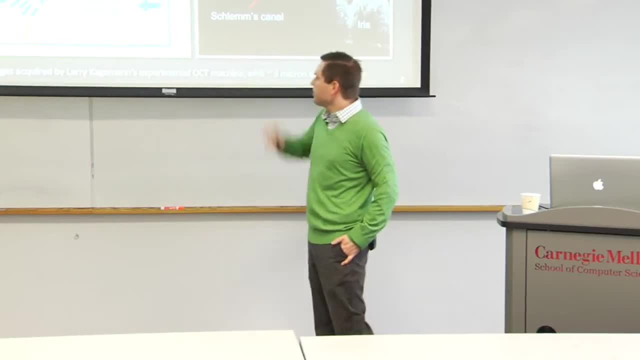 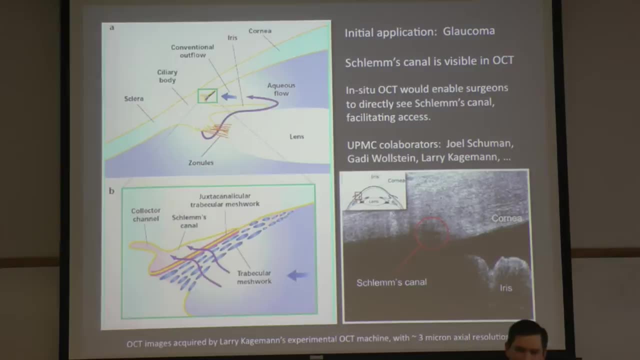 One of the ways we can treat this is by treating the collector channels that drain intraocular fluids from the eye, And all of this happens in what we call the limbus, which is the region between your clear cornea and the white sclera of your eye. 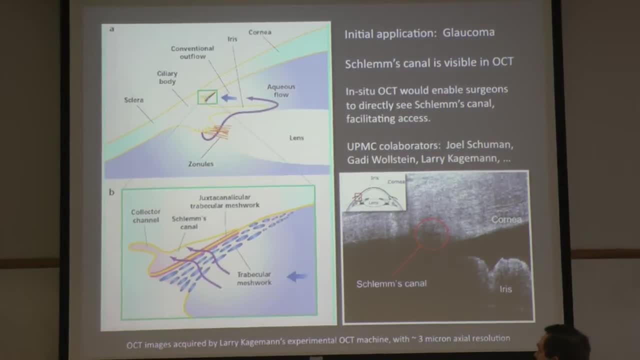 So you can imagine, right around the ring of your iris, everything interesting all comes together And you can see I'm right up here. you have a cross-section of the eye, The cornea comes down and suddenly we switch to the white of your eye. 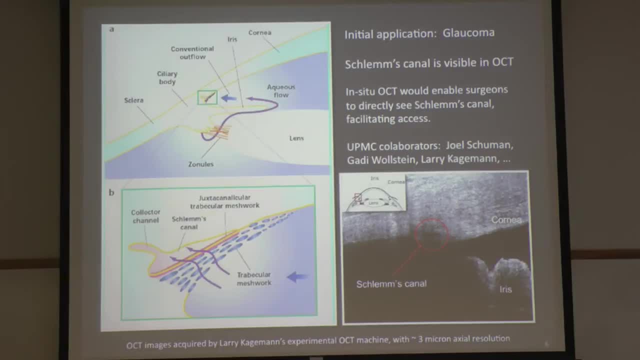 And here's the lens floating inside it, And this little part right here is where everything interesting happens from our perspective. in this regard, OCT can image this and this little piece right here blown up is what you're seeing here with an actual, real OCT scan. 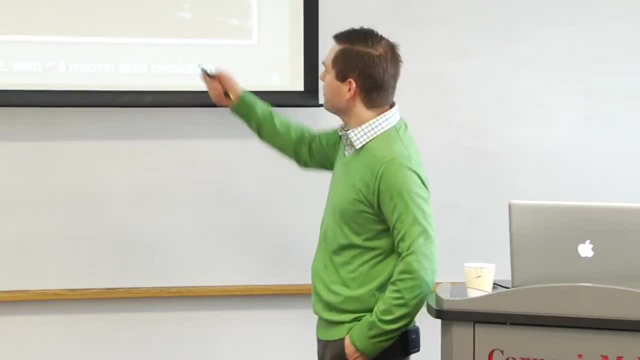 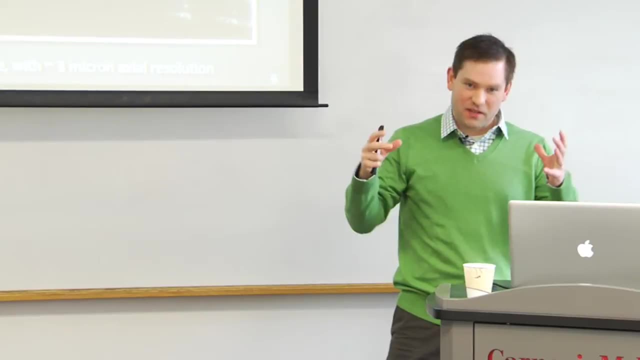 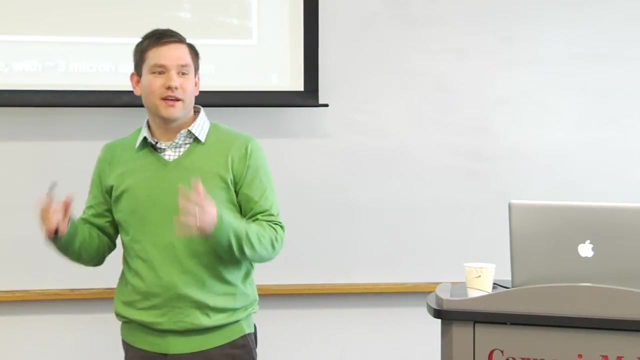 And this image was the first image in the world to conclusively visualize Schlemm's Canal, this tiny dark region right here, Which is basically a collapsed, flattened inner tube that circumscribes your iris, And it functions kind of like a ring network, if you will. 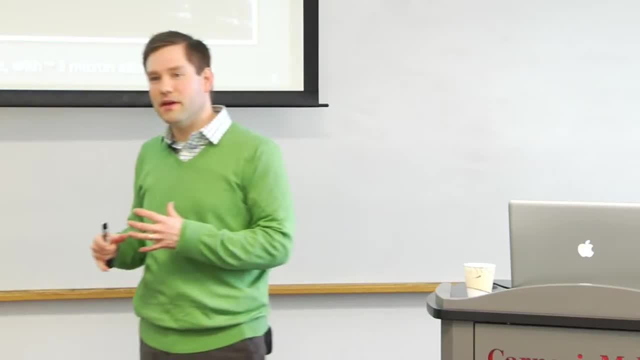 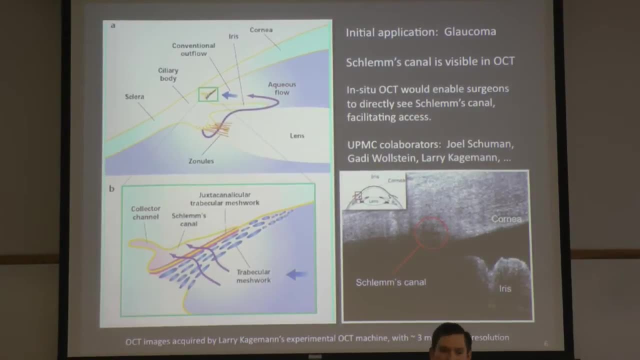 but for fluids. that makes the interface between all the collector channels that gather the fluid from your eye and then lead into the channels that feed these fluids into your actual venous system, so that you can have the exchange of nutrients and waste between your bloodstream and between the eye. 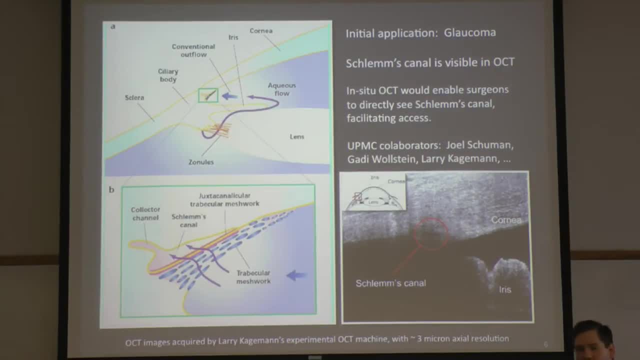 Schlemm's Canal can in fact be roto-rooted, if you will kind of like plumbing. OCT can image this and this little piece right here, this little piece right here, this little piece right here. they basically take a tiny needle. 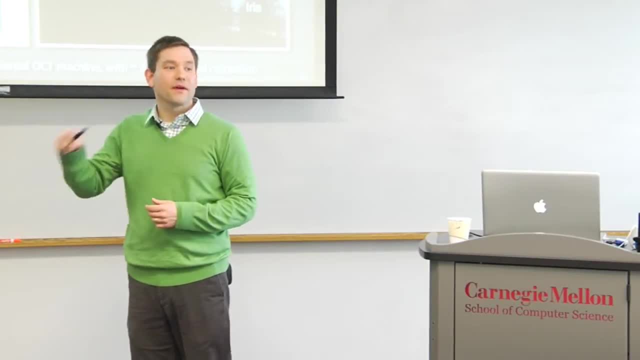 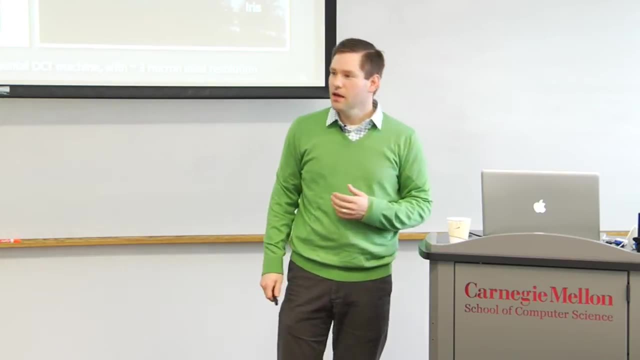 they thread it in, stick Schlemm's Canal and thread the needle all the way around the eye. This forces it open and this, generally speaking, does reduce ocular pressure and lead to improved outcomes. One of the problems with this is that you can't see Schlemm's Canal. 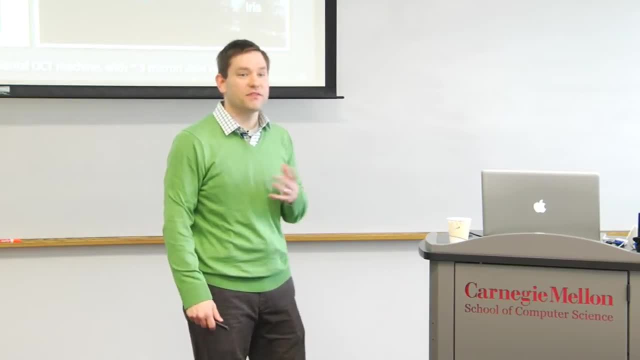 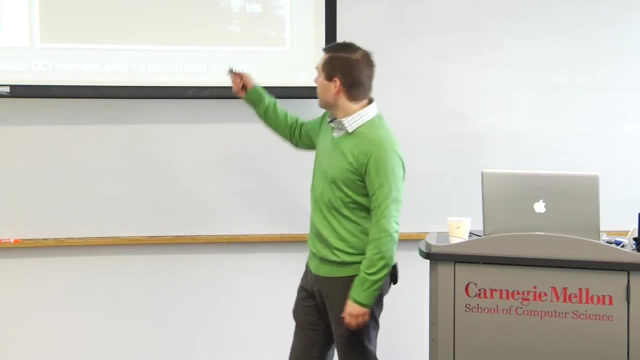 Even with the highest power surgical microscope you could use, it's not visible. Now, these structures are generally from one transparent structure inside of another transparent structure. There's no way to see them. OCT on the other hand, as you can see, 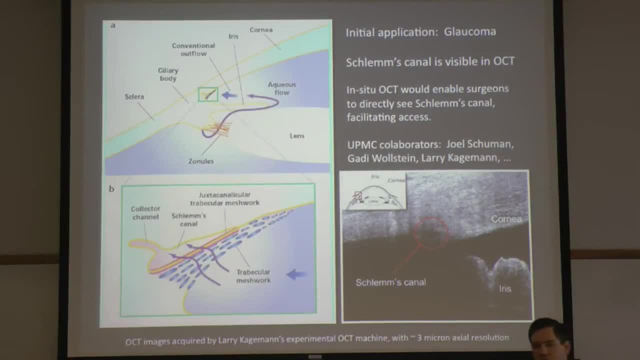 can pick up the different lengths, layer transitions here and see it. and so, instead of surgeons poking about where it's supposed to be and trying and trying again until suddenly the needle starts, following this path without too much resistance and causing lots of damage in the meantime while they try to find it, 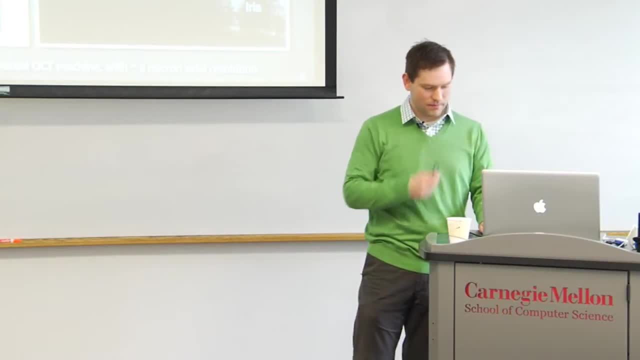 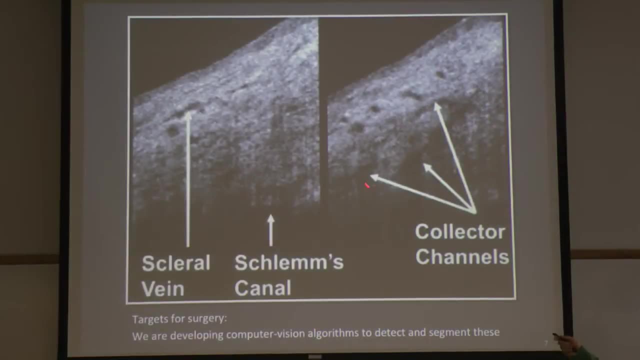 they could directly aim for it, stick it, hit it and have much less damage in this procedure. other targets of interest for various procedures: the collector channels, scleral veins and again slim's canal. you can see right here. this is image. does not look very good on the projector, unfortunately, and if i had a quality monitor? 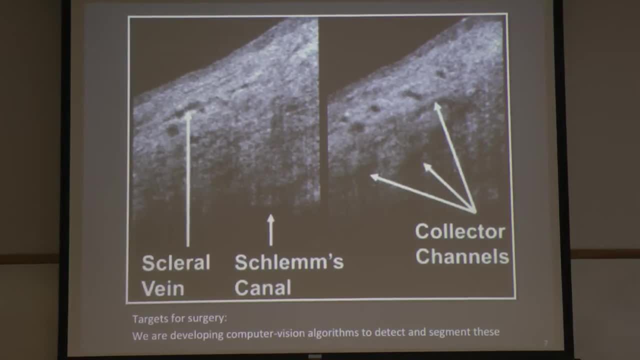 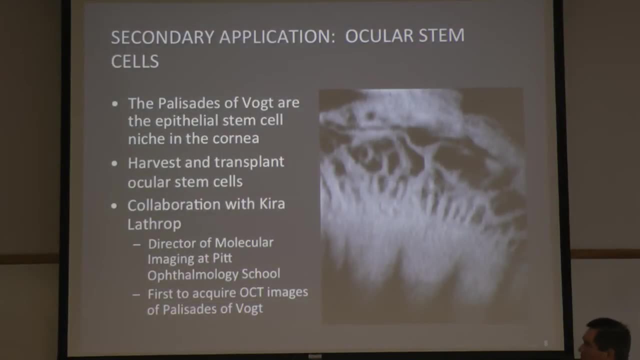 in front of you with good contrast. in the dark grays you'd be able to see that more clearly. other applications here. i do not have funding for this. this is going into future work. the palisades of watts are the epithelial stem cell niche in the cornea. these are really important. they help or they produce the stem cells that your cornea heal itself regenerate. if you do cornea, corneal transplants, you really don't want to have cornea transplants. you really want to have cornea transplants. you really don't want to have cornea transplants. you really don't want to have cornea. 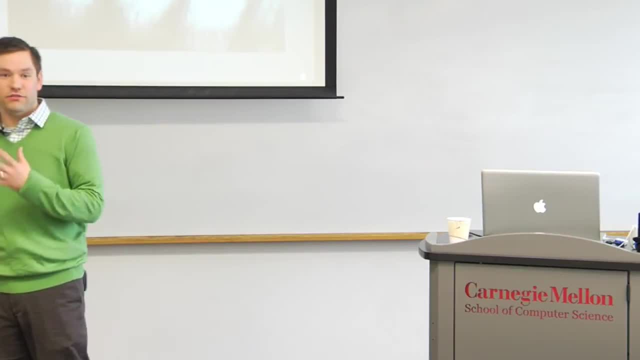 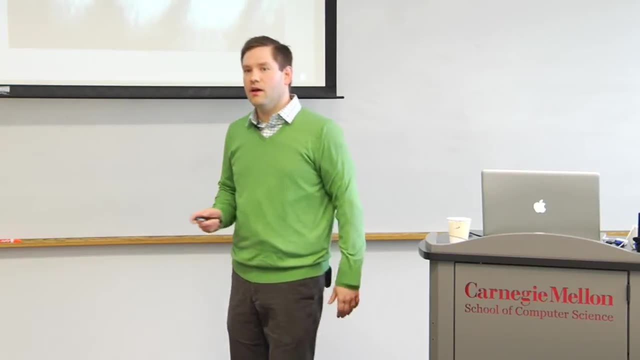 transplants. you really don't want to have cornea transplants. you really want to carry these with them. if you want to do science with ocular stem cells, these are important, but there's currently no real way to harvest these things, preserve them or do anything with them. the first person ever to see. 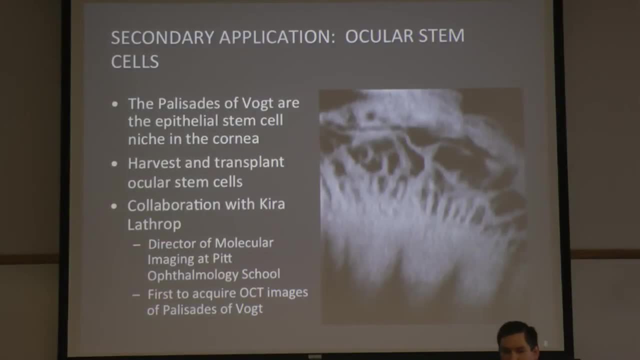 these things in oct. kira lathrop is one of my new collaborators in ophthalmology and she and i plan to take the system we're developing and then proceed to tweak it to enable harvesting of these palisades so that we can actually enable new forms of clinical 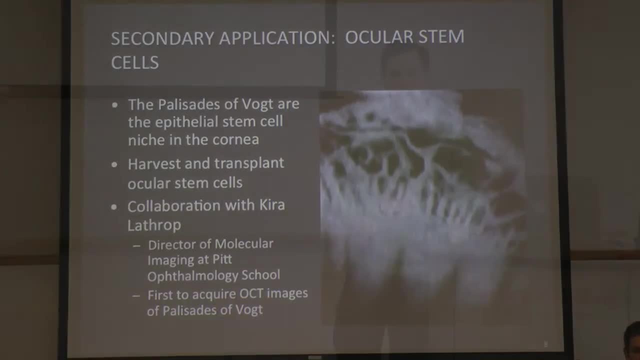 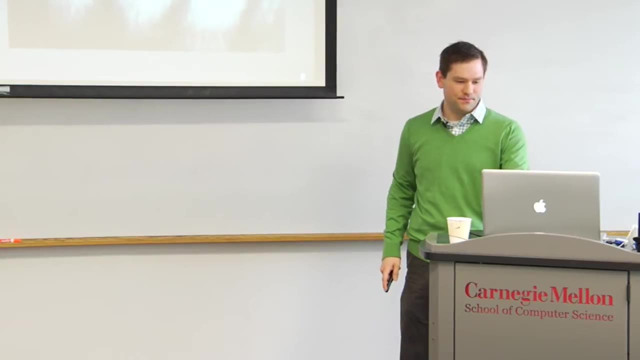 treatments, new forms of science and stem cells and a wide variety of clinical and scientific applications here, just by being able to see what we're doing with harvesting these, transplanting these, preserving these things. at this point, i'd like to talk a little bit more about what oct is. 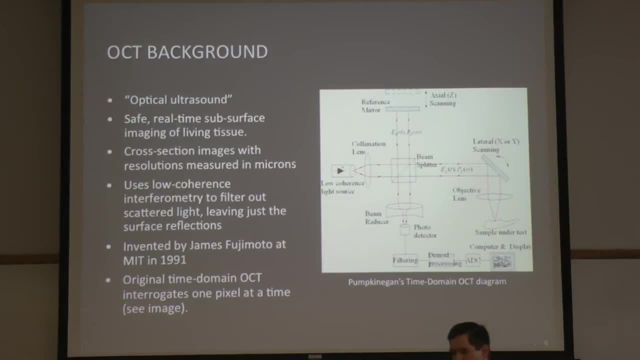 very briefly, i'm not going to go into too many details here. the basic idea of oct is that we're going to shine light into a translucent thing- skin tissue, whatever- and we want to see the structures inside and to see the structure inside and to see the structure inside and to see the structure inside. 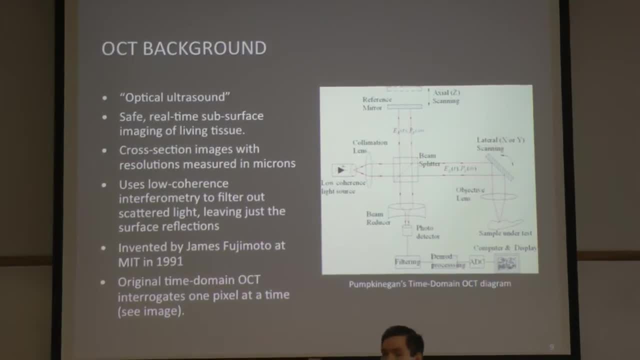 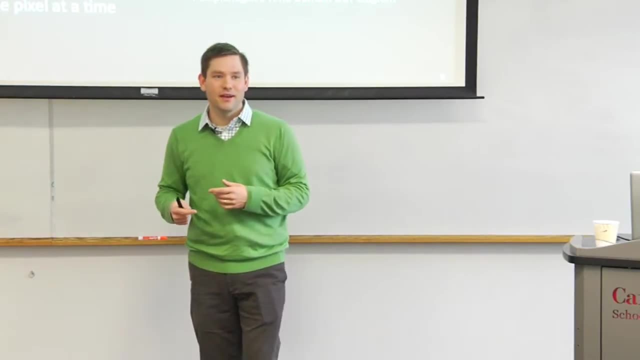 and to do that we have to filter out all of the light- scattered light. so if you shine a flashlight into your finger, you see this vague red glow as the light all bounces around inside there. we don't want that. we want crystal clear images. the way oct can do this is that oct basically uses. 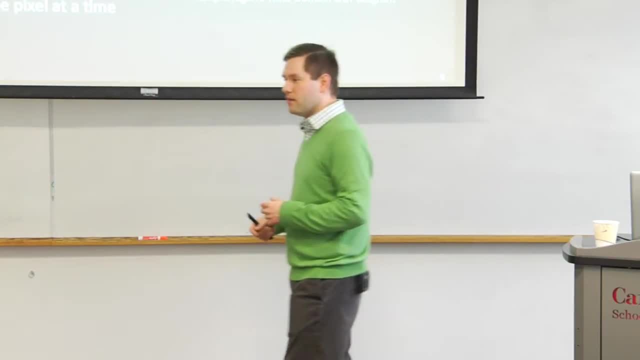 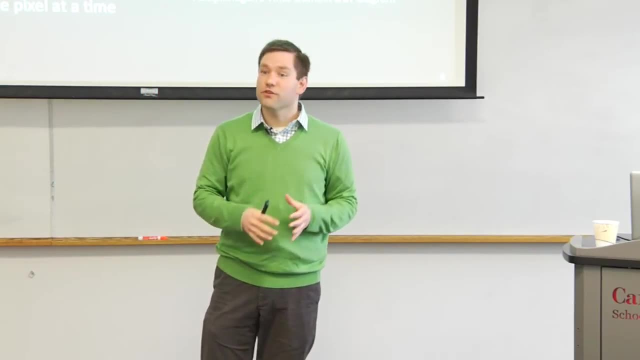 a very low coherence light source and a michelin interferometer setup so that only the light waves that follow the direct path in and the direct path back end up constructively interfering and get preserved. all the light waves that follow the direct path in and the direct path back end up constructively interfering and get preserved. 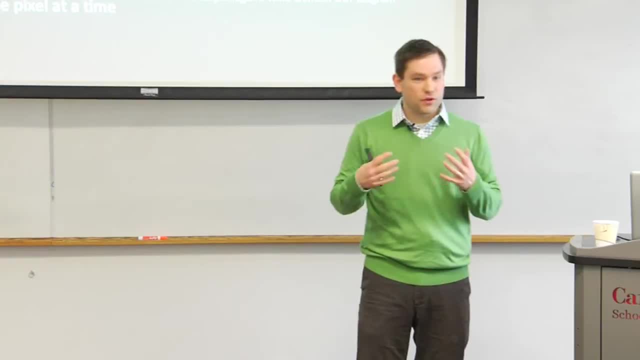 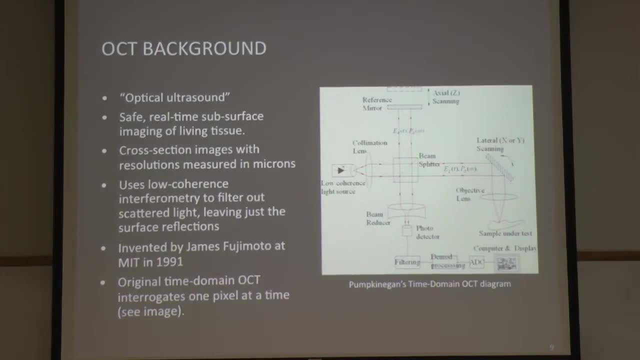 the other light that bounces around has a different path length, and so when it passes through the interferometer, we don't get constructive interference and we can filter that out. that's the very basic idea. it was invented by fujimoto at mit. my clinical collaborators were the first collaborators with him on this. co-authors. 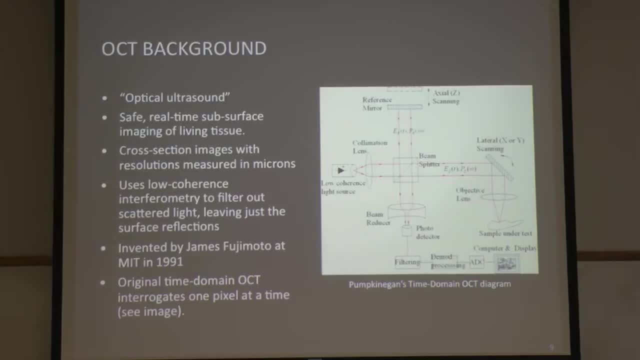 on his first science publication introducing the role to oct, and oct can image one to two millimeters deep in translucent tissue. beyond that we have so little light falling or going in and coming back out directly that we basically have no signal and signal-to-noise ratio against. 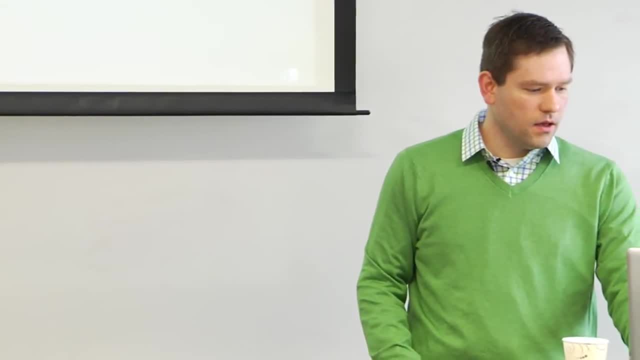 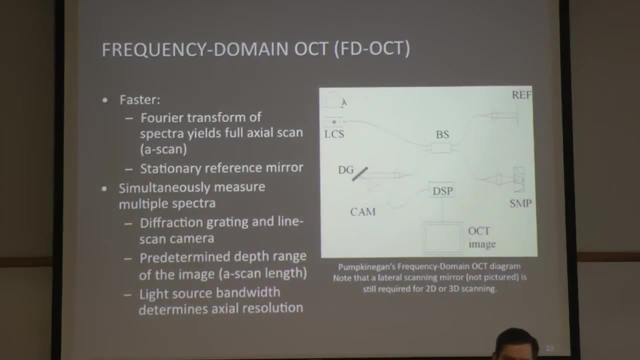 our interferometer, so that's why it gets horrible. there is an improved version of oct that uses the frequency domain to be able to image all the different depths at once instead of having to adjust our reference mirror interferometer, and this is the kind of system that we're actually using. it consists of a diffraction grading line. 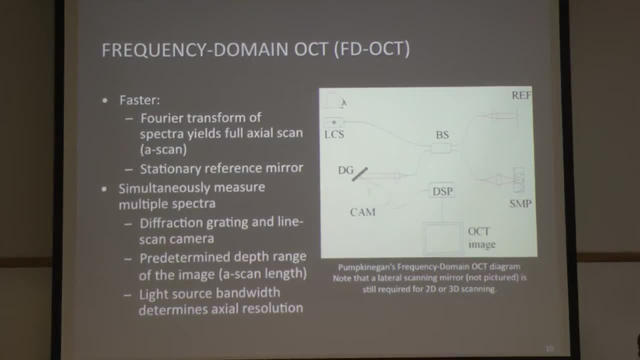 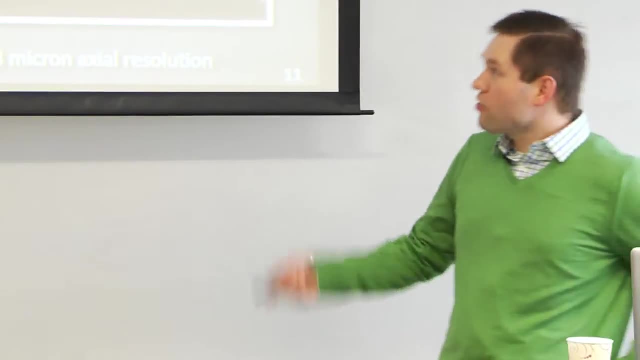 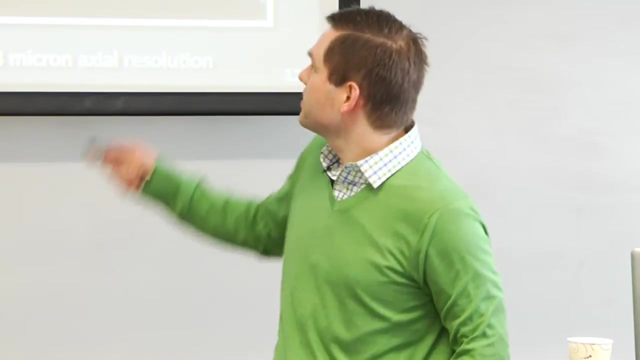 scan camera and so on, and is able to image an entire series of depths simultaneously using this trick. so our goal, as i said earlier, is basically to give x-ray vision to the surgeons, but in this case to be able to see structures that aren't at all visible in the clear cornea. for example, in oct. 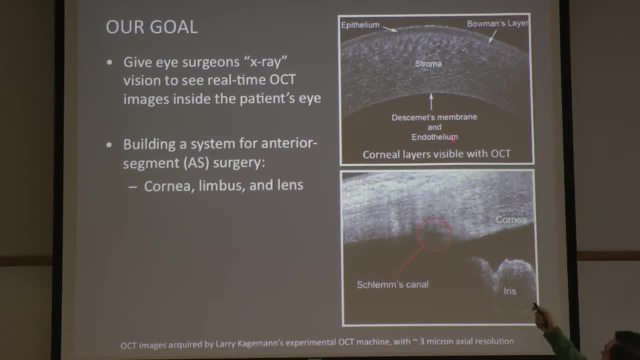 we can actually distinguish between the epithelium, bowman's layer, the majority of the cornea, which is a stroma, and even see right down here this very thin line at the bottom decimase membrane, and the thilium. there are a lot of procedures for which we want to completely remove one of these layers and 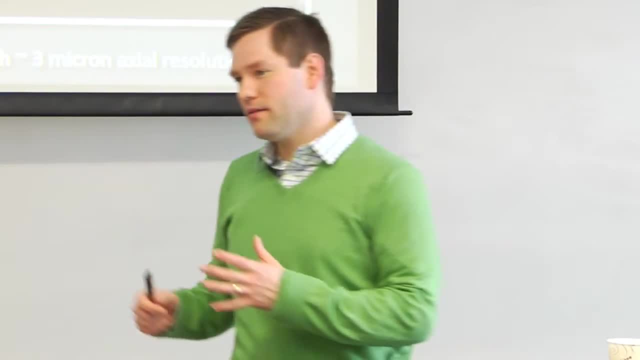 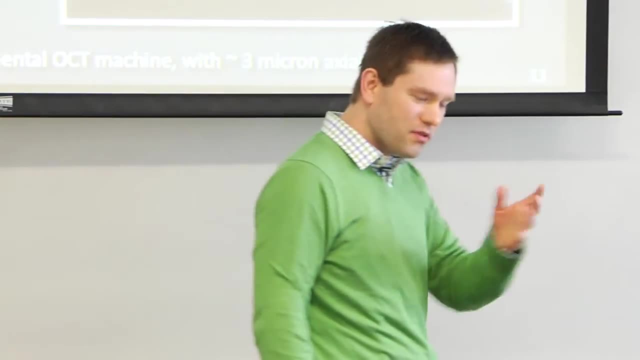 and completely preserve the layer right beneath it. And again in the clinic they try this Once in a while. they succeed if you don't have too much adhesion between the layers, but very often what would hopefully be a simple- well, simple- procedure with low risk. 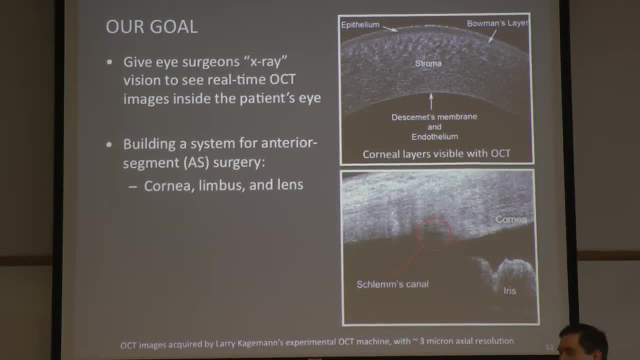 ends up having to be turned into a much more invasive procedure when, oops, by golly, we just punctured that membrane below. Now we have to remove it to transplant a lot of stuff. we didn't want to do a lot of patching. 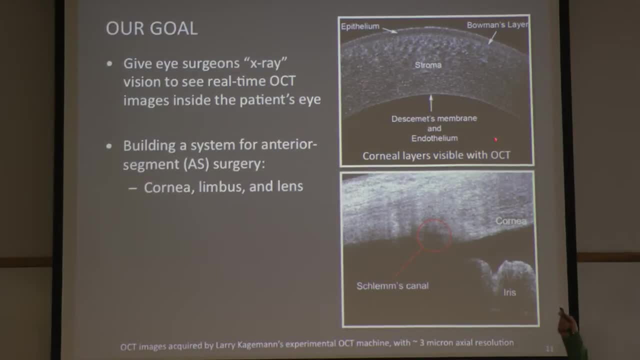 Things get complicated in a hurry frequently, and we don't want that to happen. With OCT, we could actually see what we're doing and, again, very carefully, remove one layer while preserving the other, And then, likewise, as I said, of course, 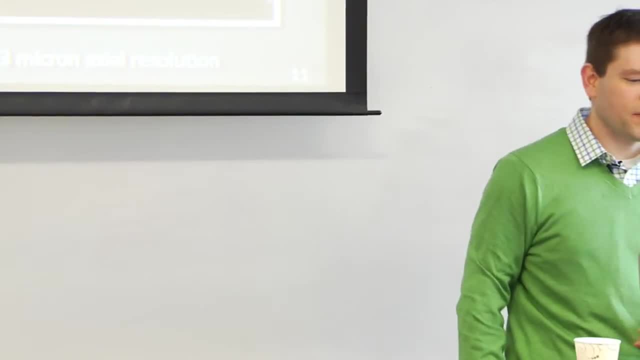 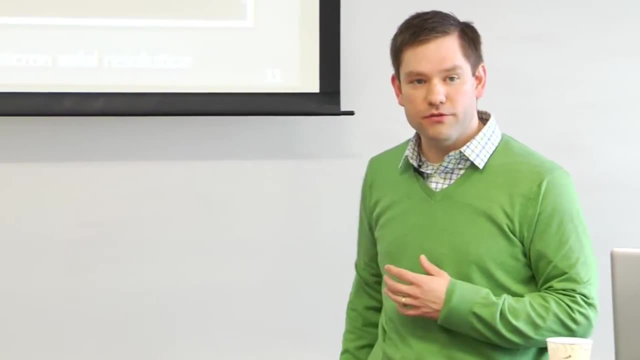 access to the canal, access, scleral veins, so on and so forth. In addition to the cornea and these things in the limbus, this could also presumably be used for various kinds of lens replacement surgery. That's not our focus, because it tends to be. 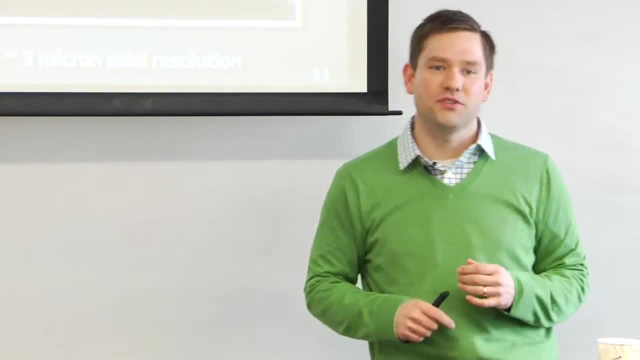 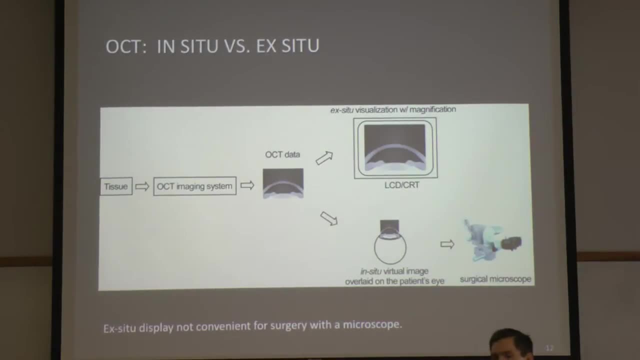 more of a replacement procedure. at the moment There's not as many fine details they're doing, but there are potential applications there as well. Using OCT to guide surgery. we need to have some kind of augmented reality system. Previously, all OCT systems to date. 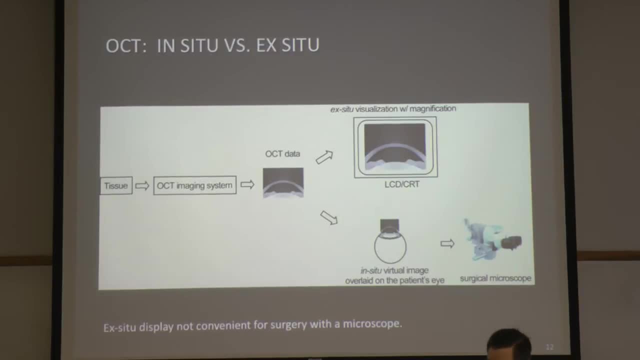 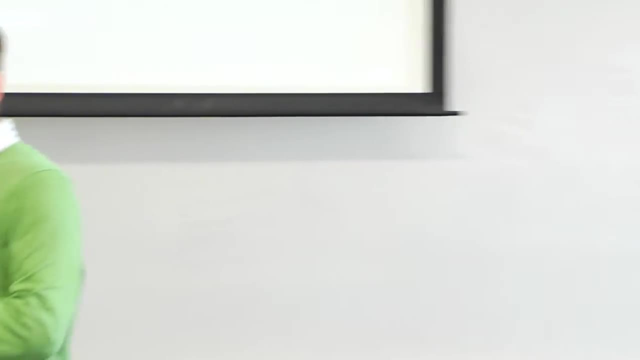 have basically been diagnostic systems. They put the OCT scanner right in front of the patient's eye, They acquire images, taking as much time as they need, and then they show them magnified as much as possible in this big, beautiful 20-inch monitor. 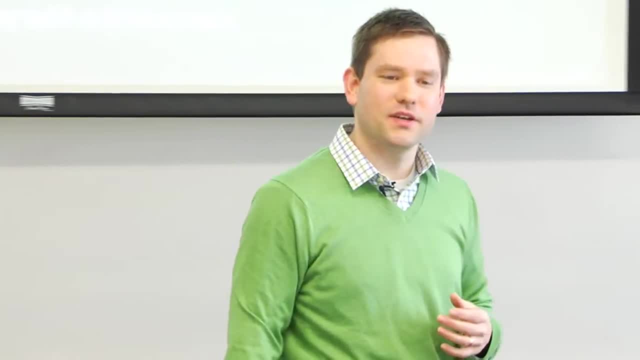 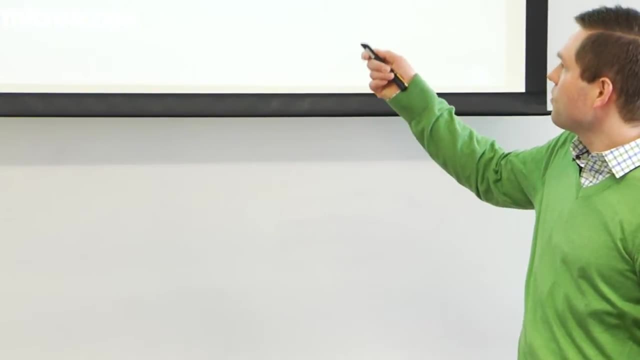 high resolution, where the surgeon can or not the surgeon, the clinician, can, fuss over small details in individual pixel nuances. In our case, however, we want to project these images at life-size scale, right inside the eye itself, perfectly registered and lined up. 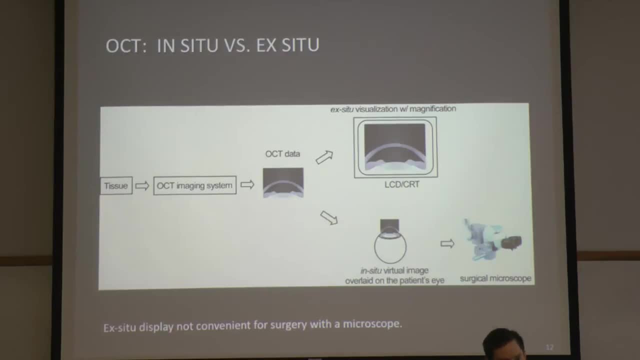 so that the magnification is happening not by putting this image on a computer monitor, but instead the magnification is happening from the microscope itself, the surgical microscope, So that the image appears in place. It's magnified exactly the way, same way that the patient's eyeball is. 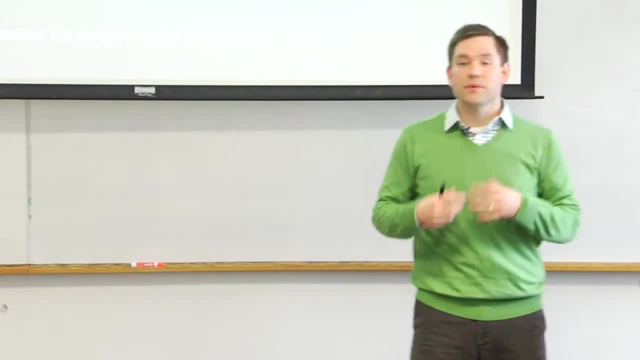 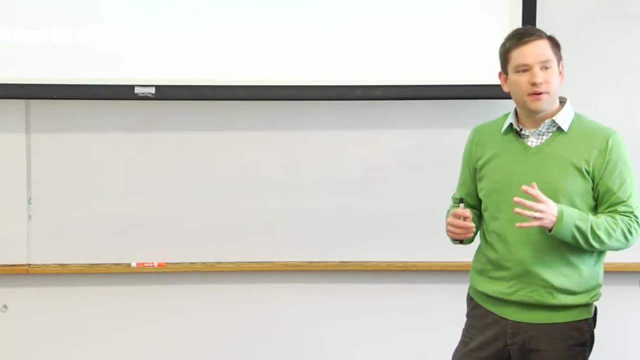 And, very importantly, the optical distortions that the microscope introduces to the patient's eyeball are equally applied, in exactly the same way, to the virtual image, And if this doesn't happen, then we lose the registration between the two. Coordination breaks down. 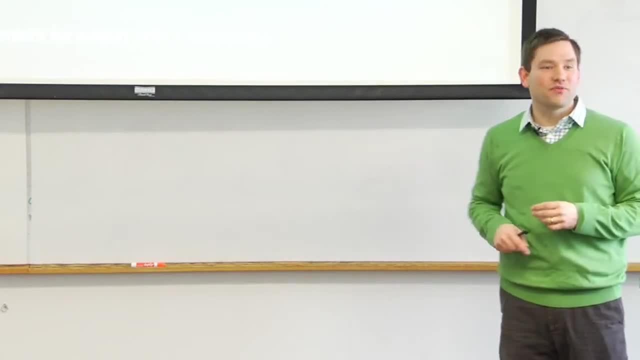 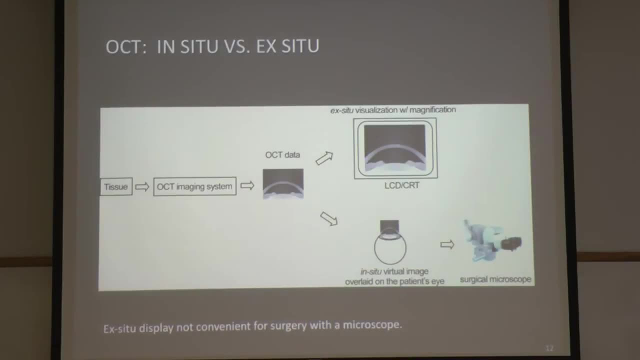 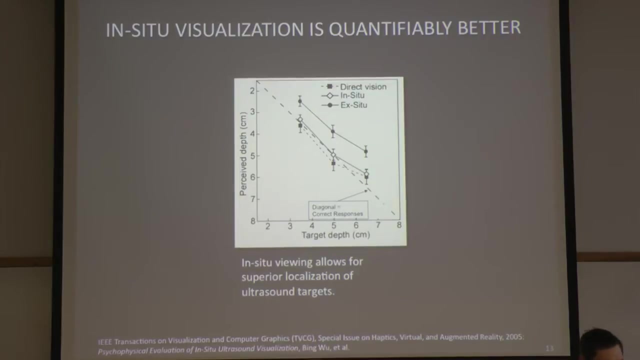 Lots of nasty things happen, So we need the bad things that happen from the microscope to happen to our virtual image just the same way they happen to the patient's eye itself. Doing in situ imaging properly has a number of benefits. It results in much more accurate aiming. 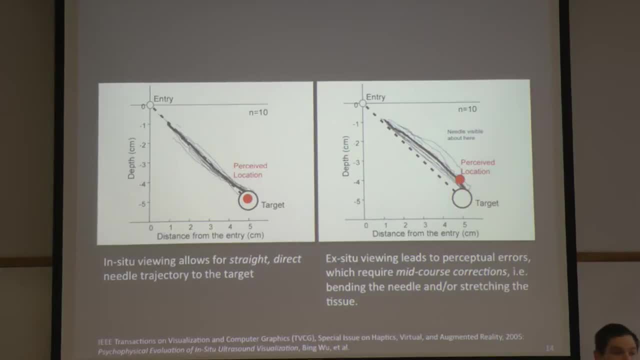 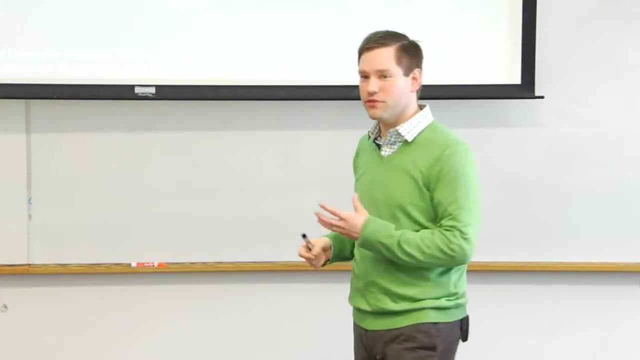 Because you have more accurate aiming, you're able to follow straight trajectories to targets, as opposed to most other systems where you aim close to right but not exactly, And as your needle tip or tool tip gets close to the target, you realize- oh wait. 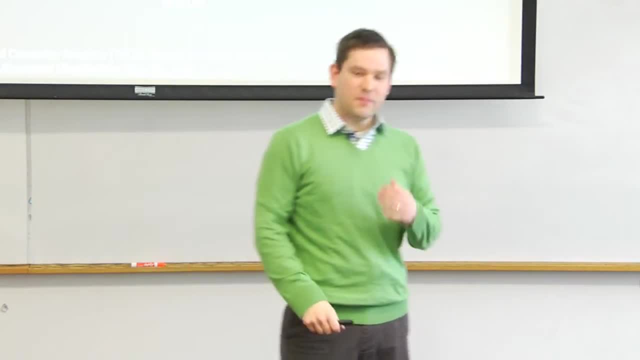 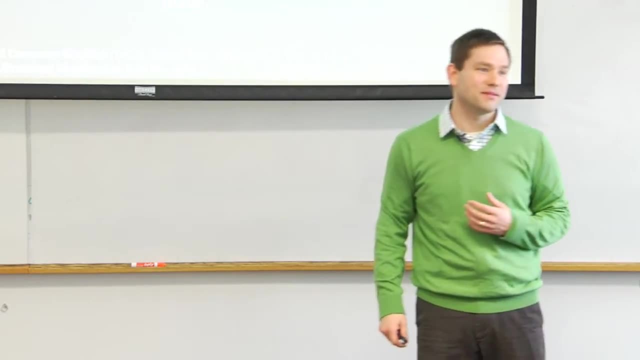 I'm off a little bit And you make a mid-course correction. Unfortunately, mid-course corrections, when your tool is partway through the patient's tissue, usually results in some undesirable tearing, stretching, nasty things. that happen And we want to avoid that. 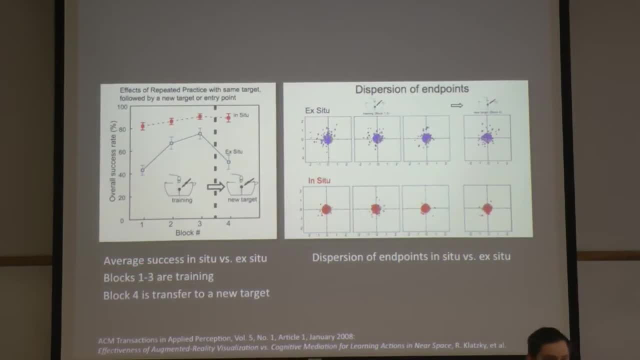 And finally, while it's certainly possible for people and clinicians to learn to aim, We want to anticipate the kinds of mistakes they'll make and work around them When they do their learning and get better as soon as you put them in a different situation, where 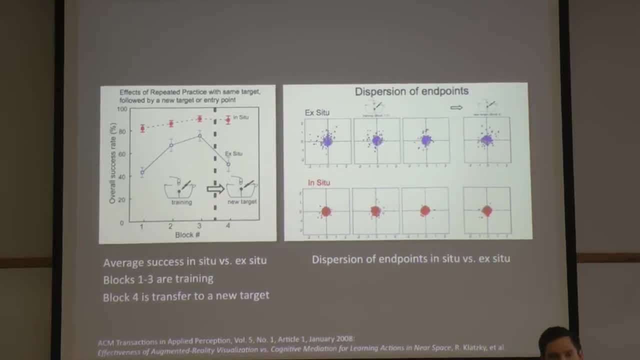 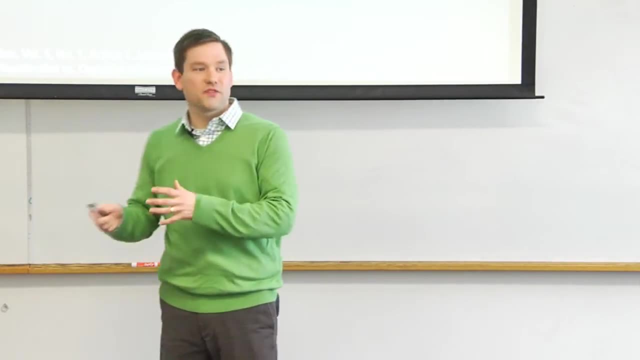 something's different. they basically have to relearn how to accommodate for the errors of the system that they're using, And when you have patients with diseases where this patient's a little bit different than everyone you saw before, this introduces problems. In fact, no two patients are the same to begin with. 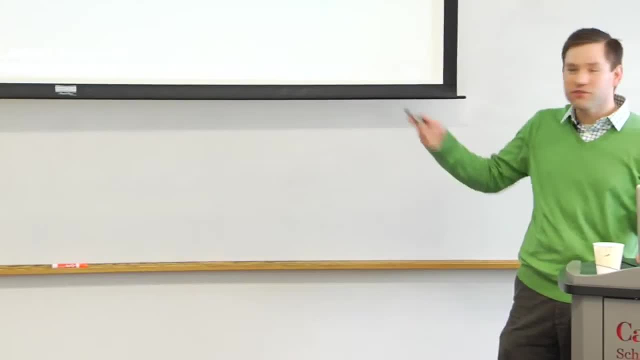 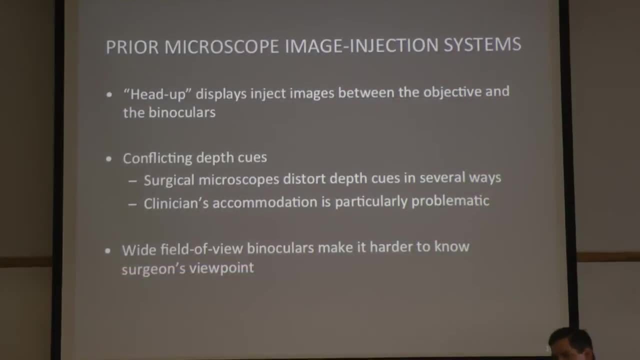 let alone in disease conditions And in pediatrics. this is particularly problematic, where we have the wide range of developments of the size of the body, the size of the bone, the size of the bone size, the size of the bone, the size of the bone size. 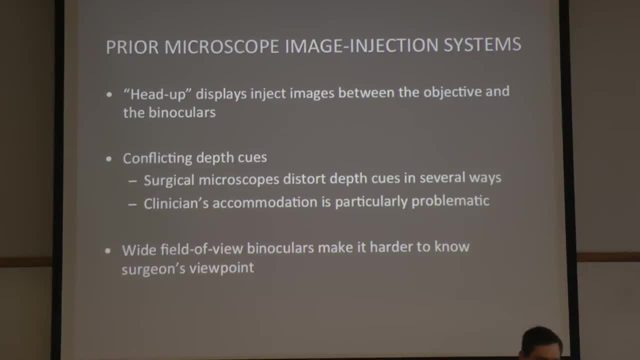 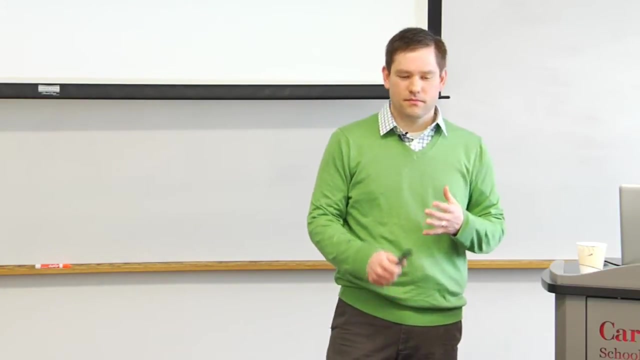 the size of the bone size, the size of the bone size and so on. So prior systems that people have made for injecting images into a microscope basically relied on a head up display approach. Very often they would just inject a single flat image that would appear to be at infinity, always in focus. 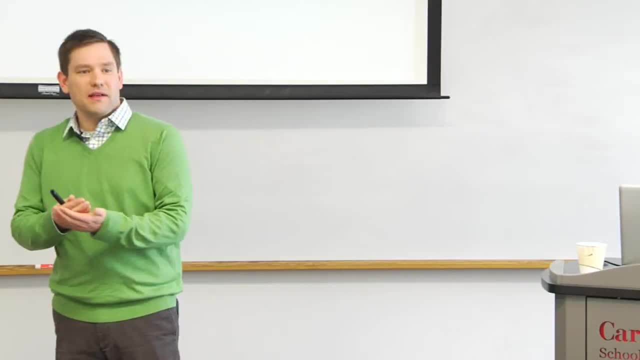 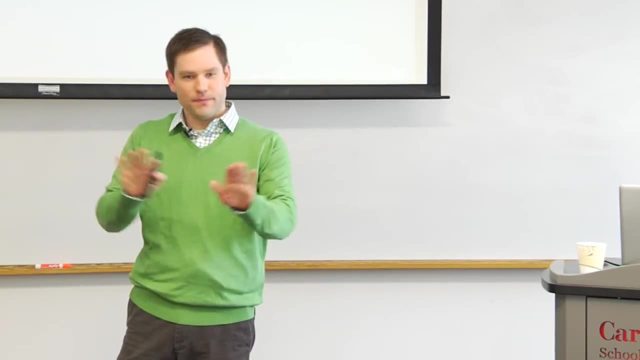 and do this for a microscope- often a non stereoscopic microscope, a flat plane- then you don't really need depth perception. There's only one plane you're operating at and all you have to do is get a linear 2D transform to align these things. 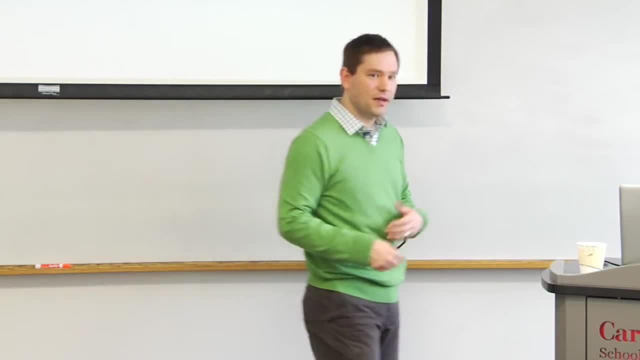 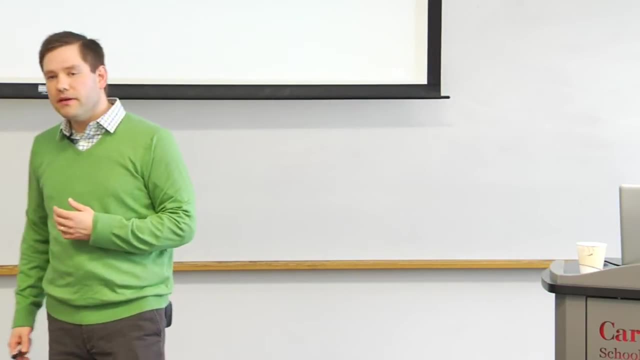 and you're good, Depth perception is kind of irrelevant, But when you're guiding complicated surgeries on three-dimensional structures, this won't work. People who've tried to work around this typically use a stereo vision approach. This is kind of like what happens when you go to the movie theater and see a 3D movie or play a 3D video. 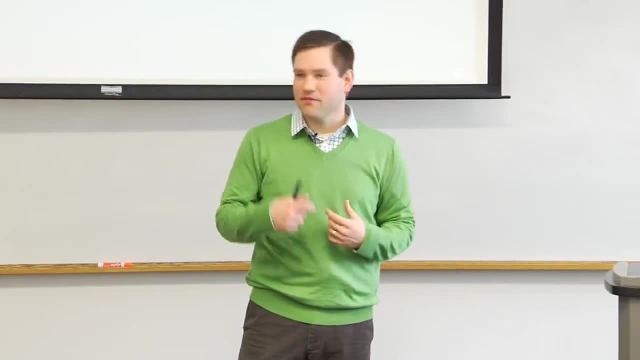 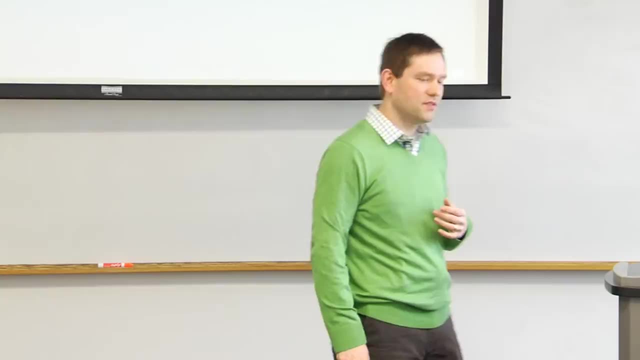 game and so on, where a system directly computes different viewpoints for your left eye, right eye. your brain sees the differences in those images, uses stereopsis to infer depth from that and produce a sense of depth accordingly. Now these systems still have some major limitations. 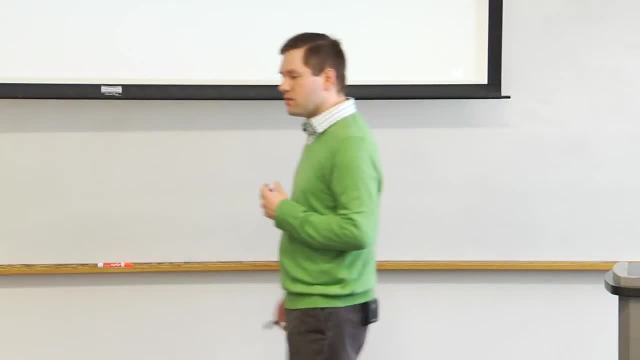 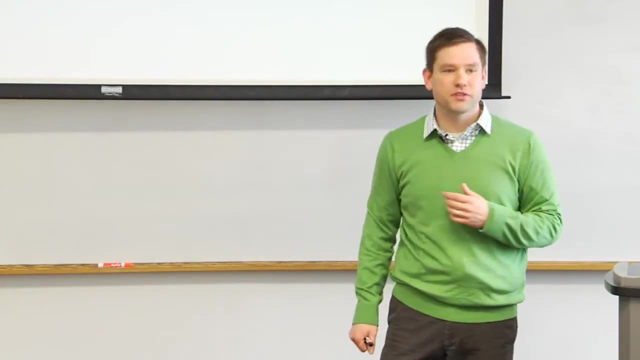 in terms of a microscope, The most important of these we believe to be accommodation, where your eye focuses. As magnification increases, stereopsis tells you less and less about where something is located, The cue that becomes increasingly important with magnification. 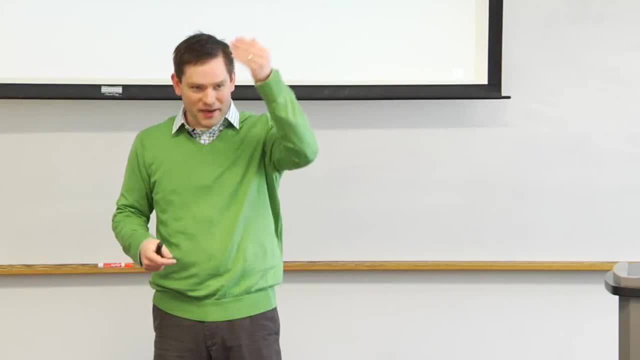 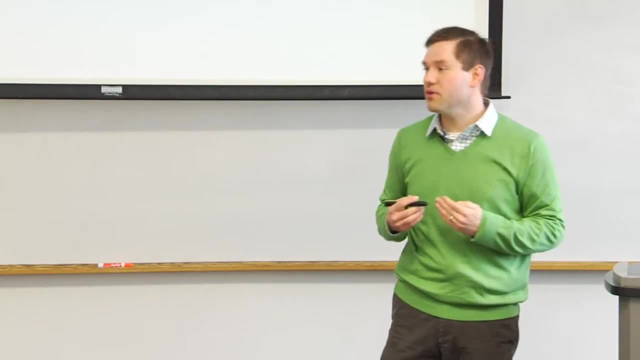 is accommodation, Because your eye is able to focus only at a 3D view. Very thin slice as magnification increases And seeing whether or not two things are in focus at the same time becomes the dominant depth cue to know where they're located Are. 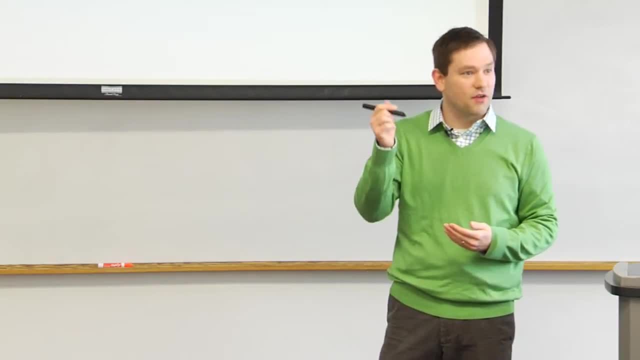 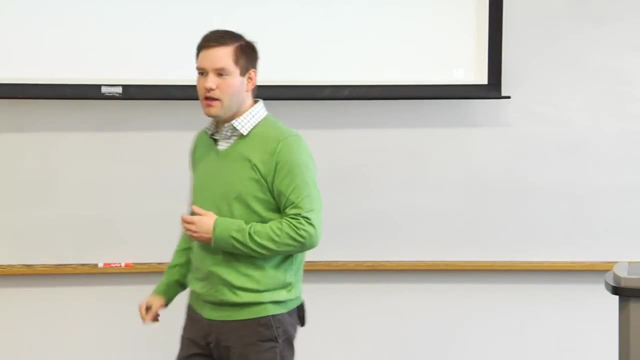 they at the same distance? Are they different? Is my needle tip at the same location? How far away is it? Well, how blurred your needle is relative to the thing you're looking at ends up becoming the most important way to tell how far away it is. And if we use a stereoscopic. 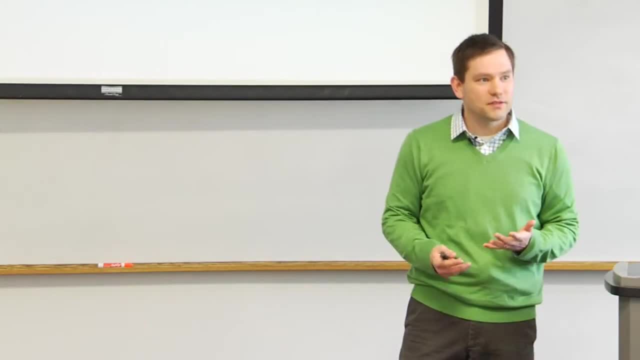 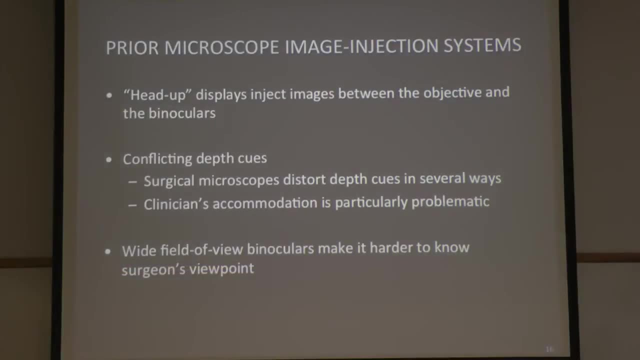 approach. this doesn't work for us. The stereo image is always in focus or never in focus, neither one of which is good, And so, by putting the image correctly in place, the way that, using our technique, all of these cues are going to be able to work correctly. 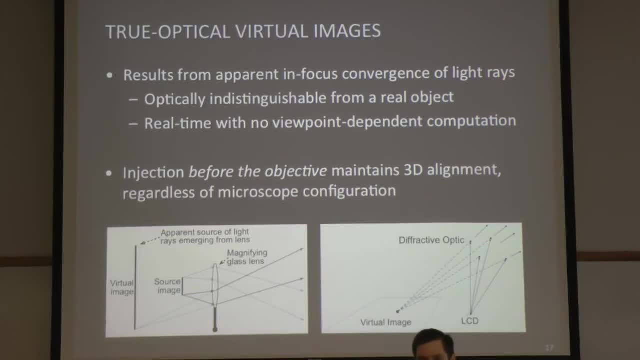 We do this by using true optical virtual images. These are the kind of virtual images made by a mirror that's made by a magnifying glass or so on. An optical virtual image produces light rays that are indistinguishable from a real object, had it existed. where that virtual 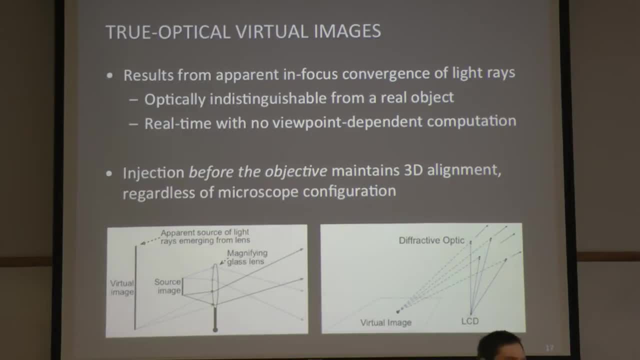 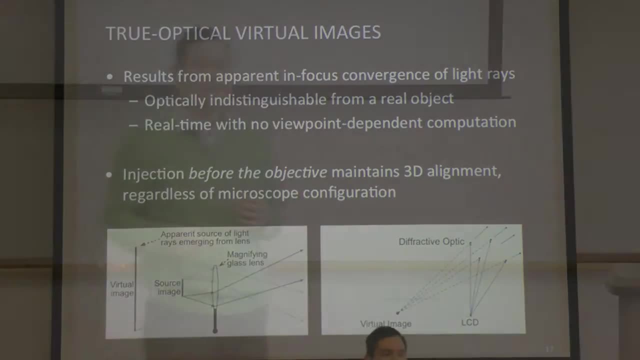 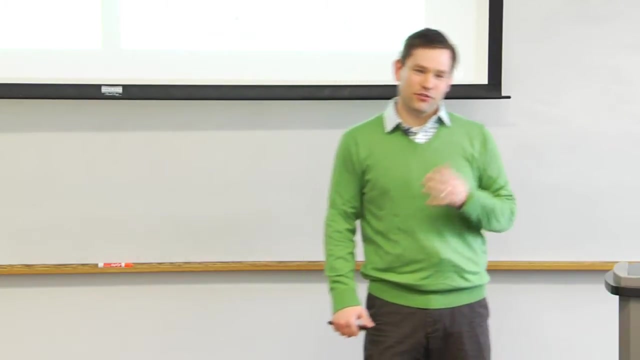 image is located, Your eyes focus on them correctly. Stereopsis happens naturally without any real-time computation. Your ocular convergence works. All of the depth cues work correctly, perfectly and naturally with a virtual image. if only you're making a perfect virtual image. Now it turns. 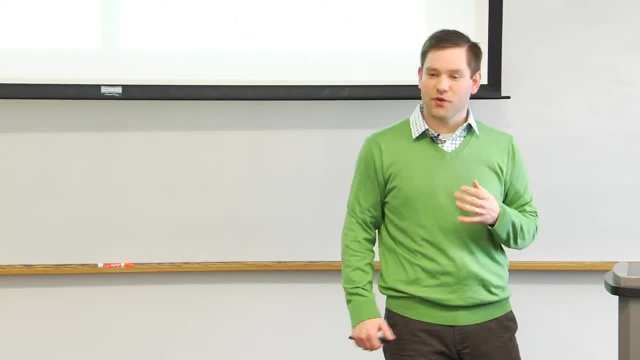 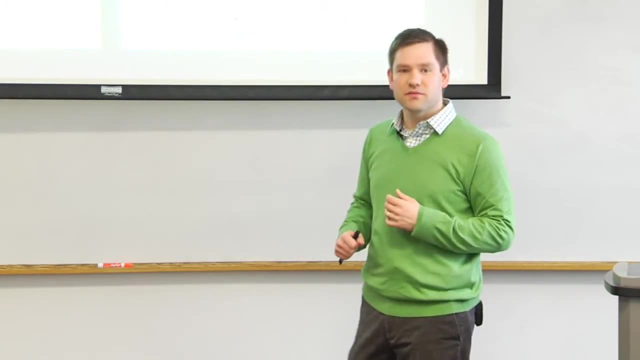 out that trying to produce these for anything other than a one-to-one mapping with a mirror is a really hard thing to do. accurately. You end up with blur and that messes things up. But we can still optimize systems to make the residual error within acceptable thresholds. 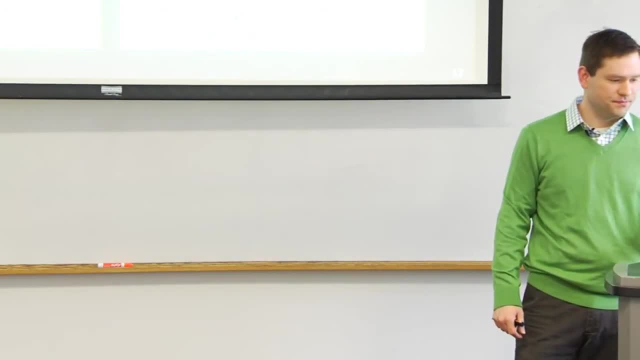 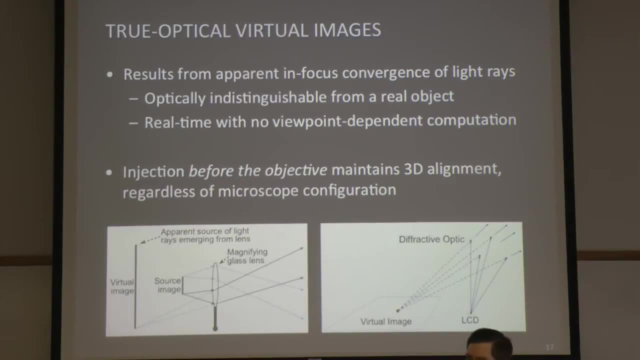 say, a millimeter, microns, whatever kind of scale we're working at, Because we take one of these virtual images and inject it beneath the objective lens of the microscope, as I said earlier, all of the optical distortions of the microscope get applied equally to the virtual image as well as to the patient. And because of that, 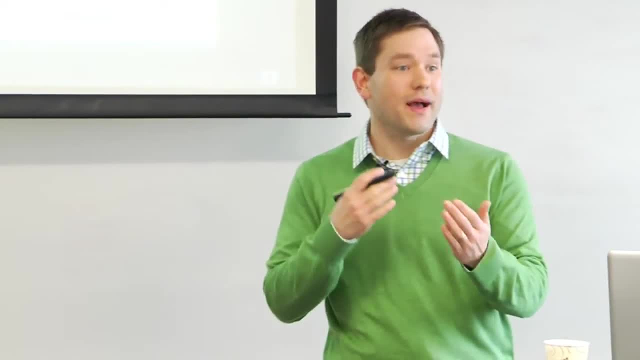 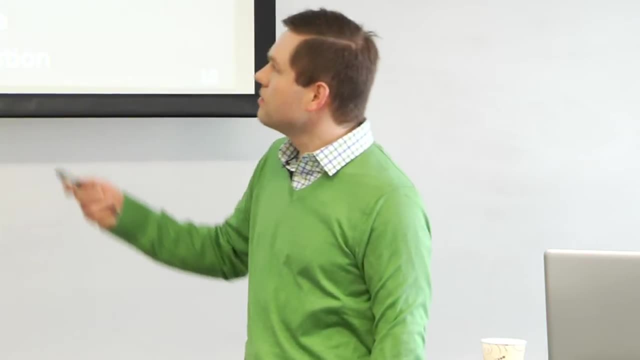 there is this perfect alignment that remains between the two and we have the perfect focus- or lack thereof- between things that are at different depths. All of the depth cues work. The basic idea represented simply here is to have the OCT scanner imaging inside the 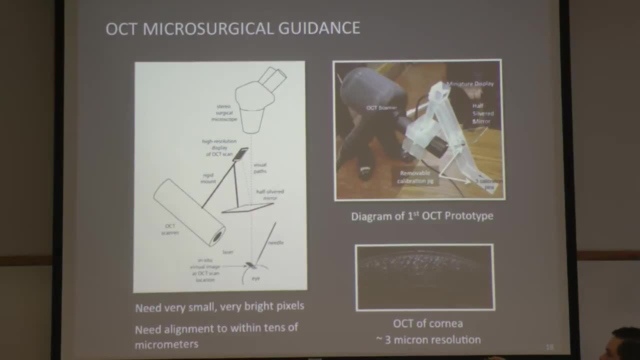 patient's eye And one way or the other we use something like a half-silver mirror to make a virtual image of a life-size scale image of the OCT scan, such that the reflection appears down in the eye in the exact correct location. So when you look through the microscope, through 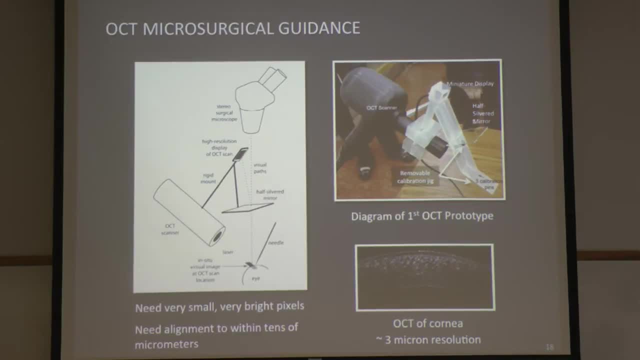 the mirror, you see the virtual image floating in place, And this is the simplest possible way you could do this. We produced a couple of prototypes. This was the first. It actually did not produce a nearly bright enough image to be visible under the microscope. Microscopes expand the image and 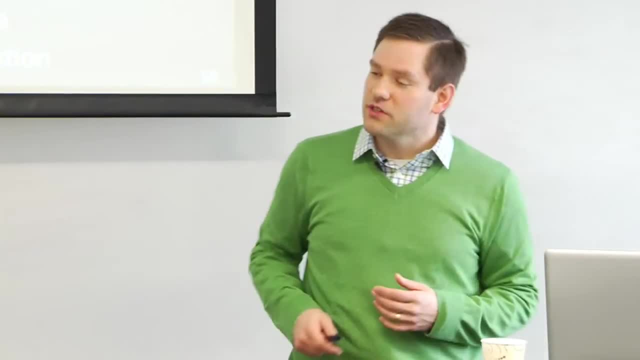 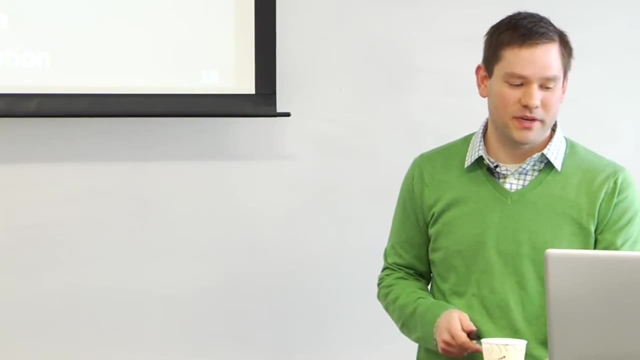 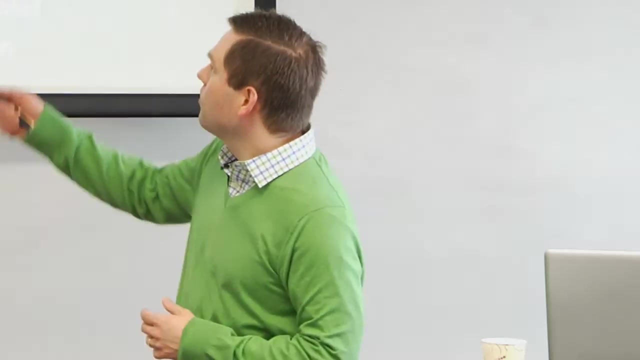 therefore dilute the light flux per millimeter. This is the reason why microscopes have bright lights on them. Unfortunately, bright lights don't help with a flat-panel display by making it brighter, because it has its own internal illumination. I led a senior design team to produce a new prototype which borrowed technology from 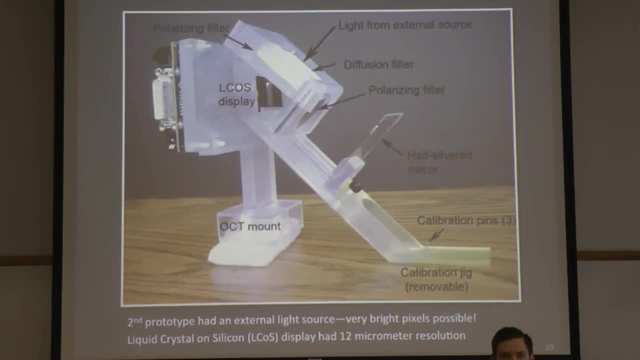 rear projection televisions designed to have external light sources using a liquid crystal and silicon micro-display, And using this approach we actually were able to produce a very small, very bright, high-resolution image. In this case, you can see three very tiny metal pins here. the OCT image of the three. 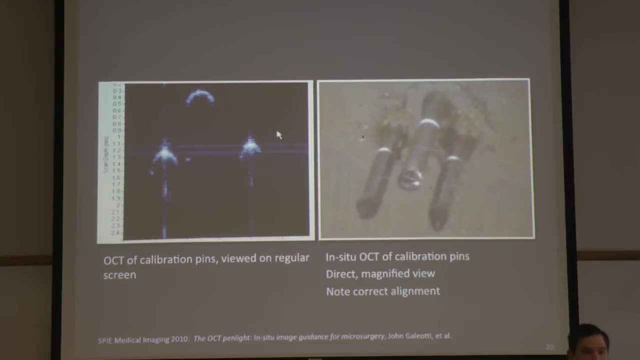 of them. It has specularities happening at the cross-section, but you can see the three simple curves And, looking through the calibrated system, you can see the curves of the OCT are perfectly aligned with the three pins. we're looking at demonstrating that the system is calibrated. 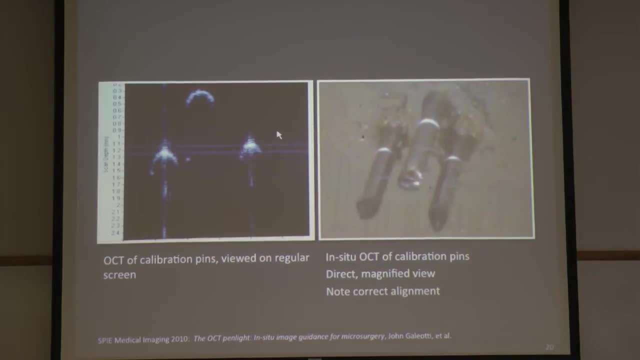 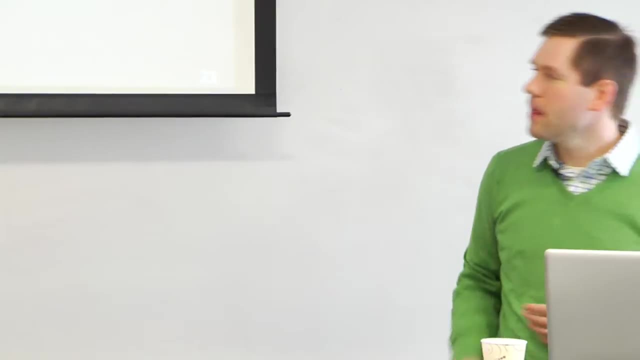 and they're able to see it correctly, And I think the resolution of this display was 12 micron pixels, I believe, and could easily adjust the brightness to whatever magnification we needed. Proceeding with this, we're able to produce the world's first ever in situ image of OCT. 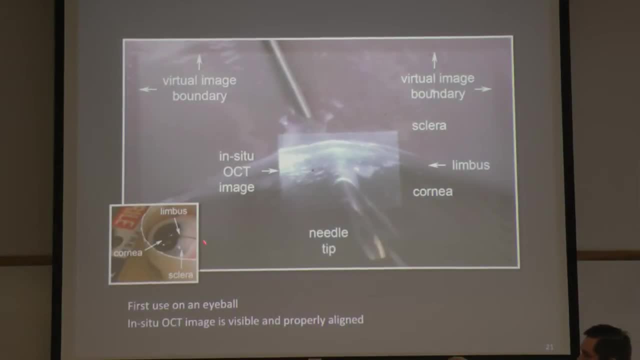 inside of an actual eyeball. In this inset down here you can see an excised cow eye And you can see the cornea here, the white square over here, And that limbus, the interface region, has a needle stuck through it. 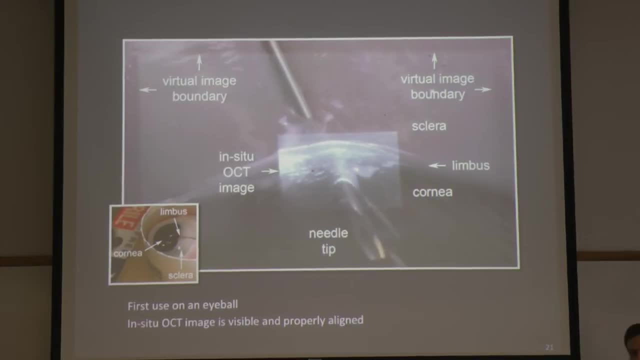 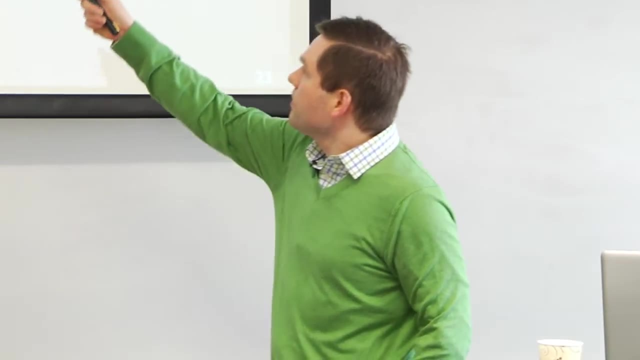 And this is a crude approximation, but to demonstrate for the imaging, something like what's going to be happening in limbal surgery: trying to access the canal, so on and so forth. This is the view: through magnification, You can see the needles coming in. 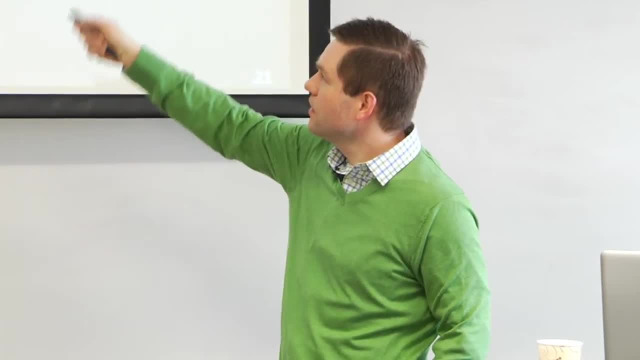 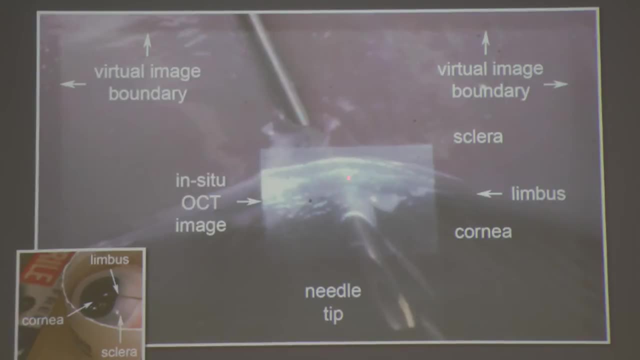 It's penetrating through the sclera right before we reach the limbus here. Here's the boundary, right here between the sclera and the cornea. We can't see the needle here because it's under the opaque sclera. And then as soon as we get to the cornea, we can see through it and suddenly we can. 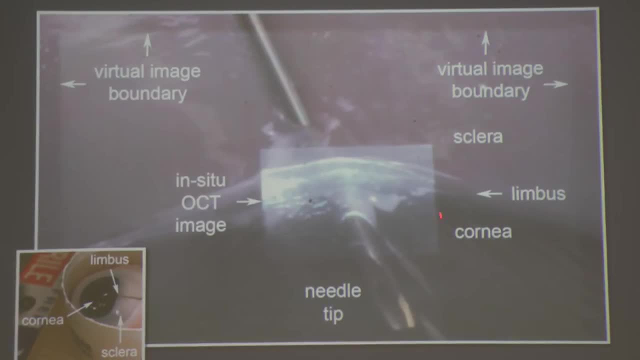 see the needle again. This box right here is our in situ OCT image. If you look at that, you can see that these folds that were made in the surface of the cornea are now open. They're open The cornea and sclera, by inserting the needle, are, of course, picked up by the OCT scan. 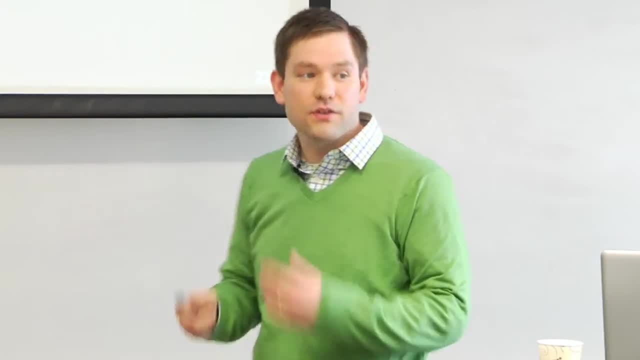 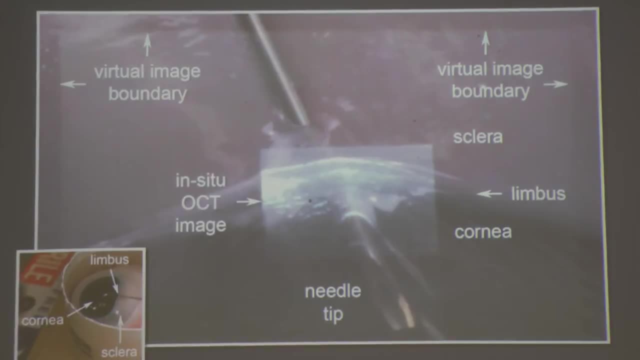 The alignment is perfect. The OCT scan also sees the needle. These are all things that are visible. It's also picking up lots of little subsurface folds that are happening, distorting the tissue underneath the surface that you couldn't see with your naked eye. 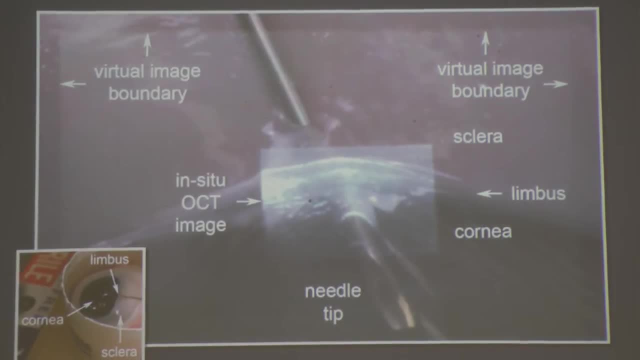 And with increasing magnification. if we oriented this differently, you could see internally into the limbal structures I was talking about earlier. This is the picture that landed us the two plus million dollar four year R01 grant that I'm currently working on. 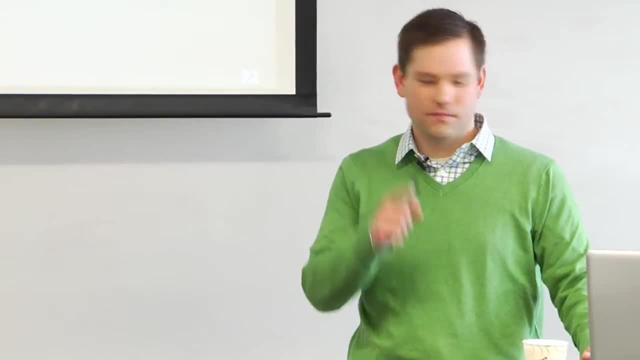 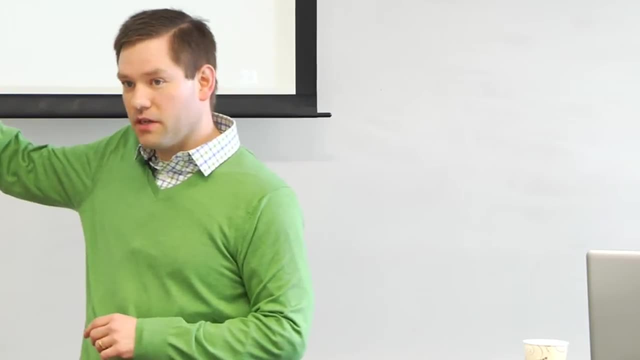 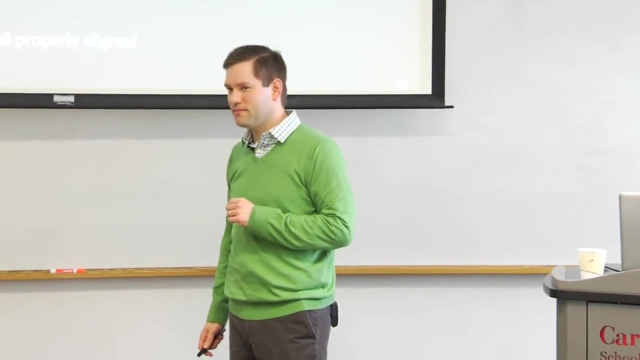 So you're just projecting incoherent light onto the tissue right? Yes, The virtual image, in this case, is incoherent. Yes, What if OCT was to use coherent light so that it doesn't scatter, doesn't come back? Now you're projecting. 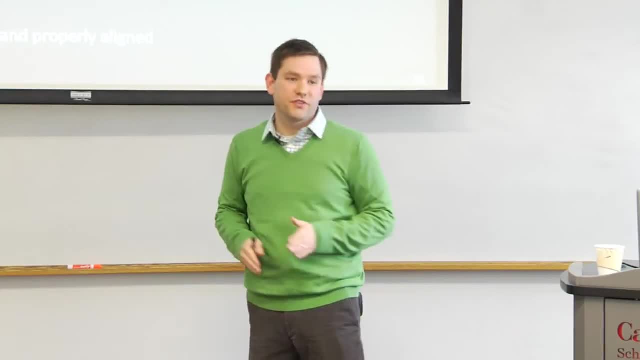 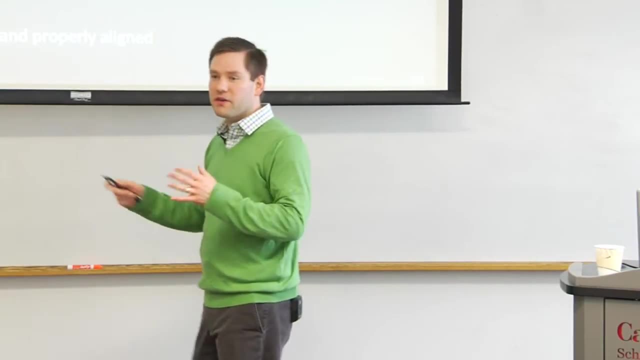 Different wavelengths. Visible light is. OCT does not use visible light waves. It happens in the near infrared, And so we can use the near infrared local coherence, Think OCT, Think OCT scanner, Simultaneously with dumping all of this light into their 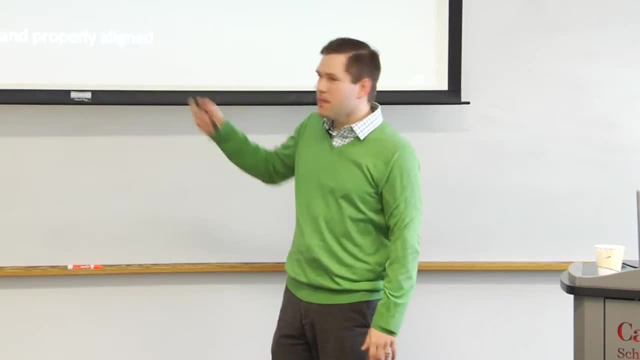 In the visible spectrum. they don't interfere with each other And, furthermore, Interaction of light with the tissue that you said you know, illuminate it off And furthermore, the virtual image doesn't actually have light coming from in there. anyway, The appearance of the tissue. 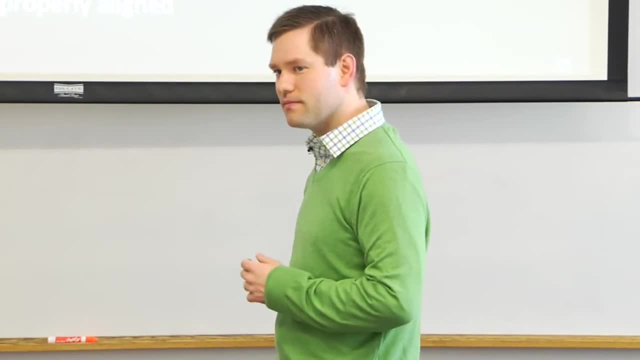 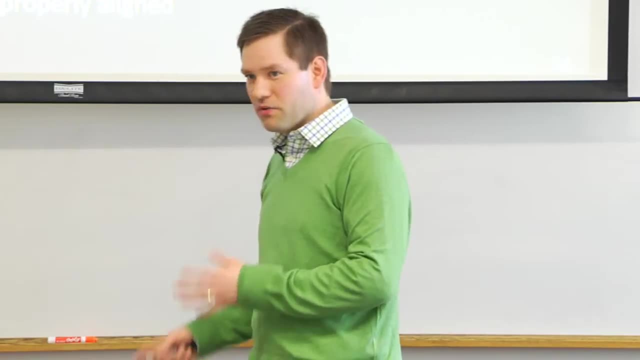 The appearance of the tissue. So if you're sending some additional light onto the tissue, Yes, That's going to get scattered By the tissue, Right, Okay, But we're not sending additional near infrared light onto the tissue And we're only measuring near infrared light. 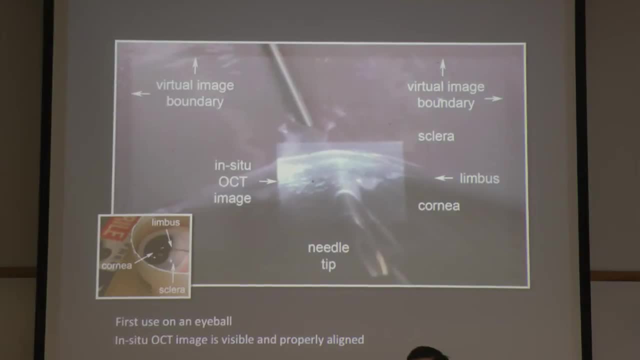 But you're projecting something on. So where is the light going? Is it just onto a screen? So the light that made the virtual image, Yeah Yeah, It's coming from a screen that's external, External, And that screen is being viewed through some kind of a beam splitter, pass over mirror. 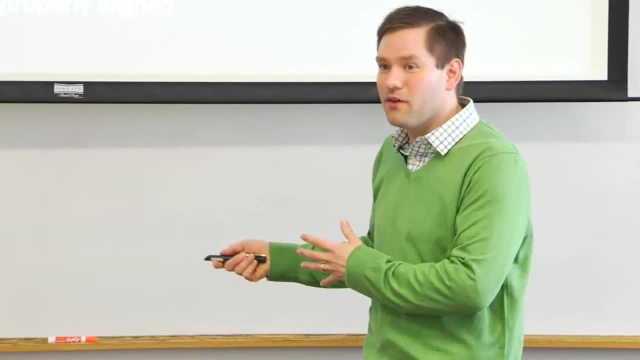 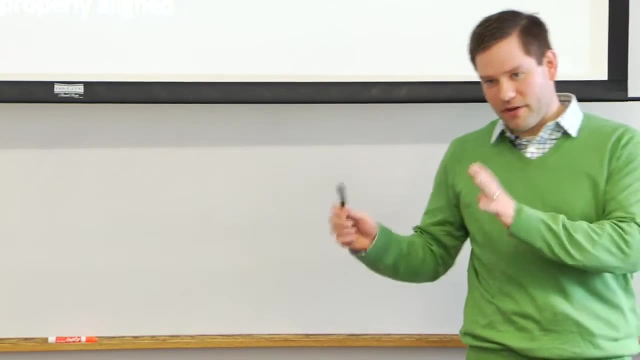 so on. Right, And that actually isn't even reaching the eyeball itself, And we have two different beam paths here. If it was, it still wouldn't interfere, though We have other stuff I'm not discussing now using, Trying to use structured light to do some other fancy things. 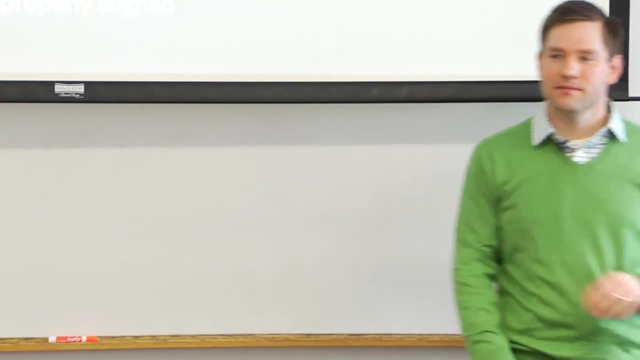 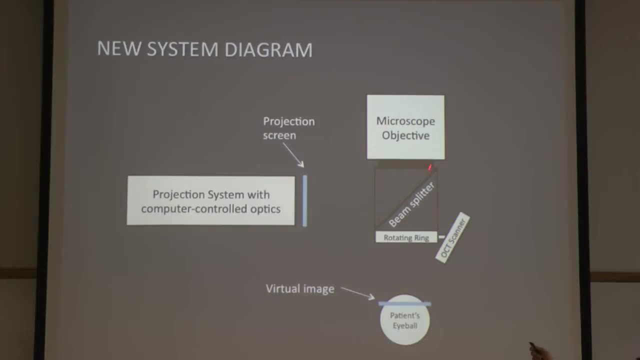 And as long as the structured light's not in the near infrared, we're fine. So we're working to develop a much better integrated system attached to the microscope. You have the microscope up here. It's objective lens, A proper beam splitter with the projection system over here, which will ultimately continue. 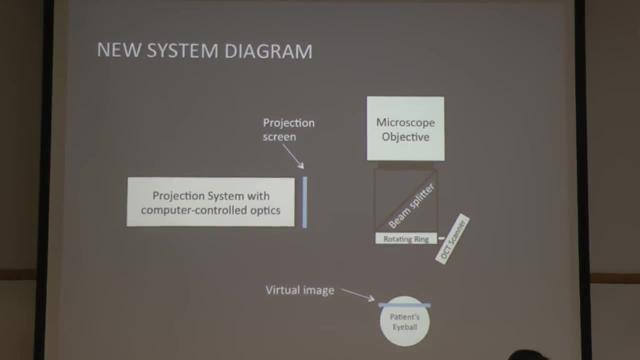 real-time computer-controlled optics, dynamic diffractive optics. to enable tricks in terms of repositioning the virtual image. We have a custom OCT scanner attached with two different rotation degrees of freedom that both have a remote center of motion about the patient's eyeball itself, enabling us 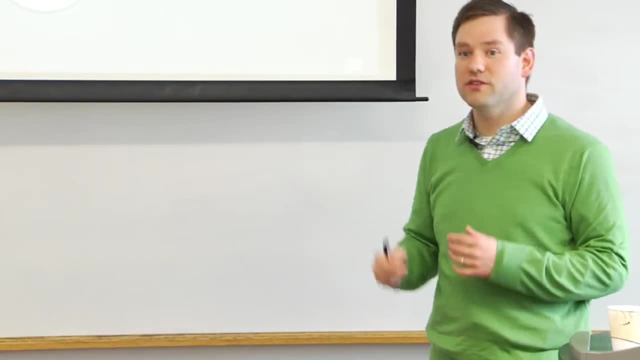 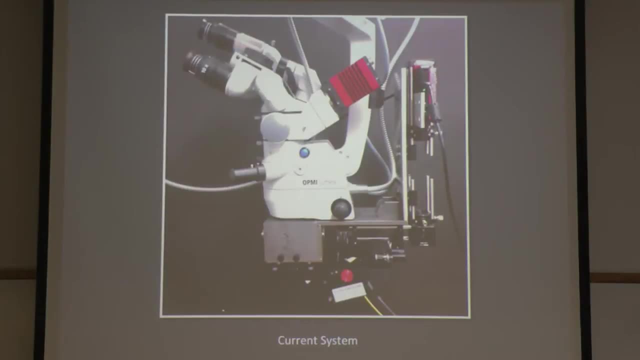 to image from different directions without getting in the way Patient's eye in the virtual image. Currently the system looks like this: We have the microscope here, The objective lens is here, And then we have the virtual image. The objective lens is right here. 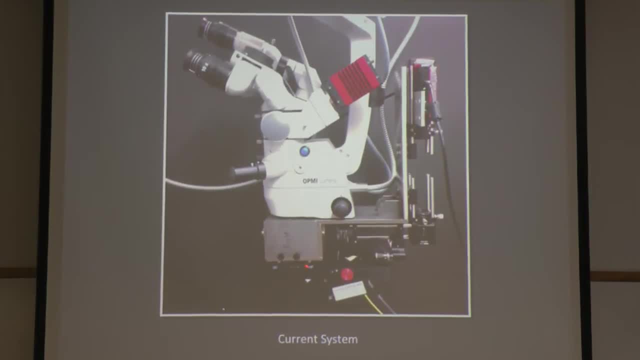 We have a box containing the beam splitter open. on the bottom We have an open aperture rotation stage here that is attached to an arm that holds our custom OCT scan head here. We then have our equipment here that is being used to generate our in-situ virtual image. 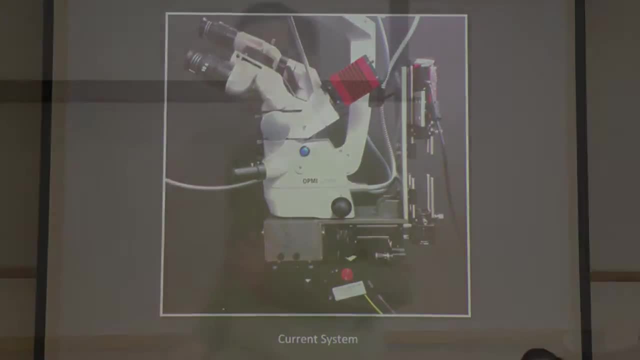 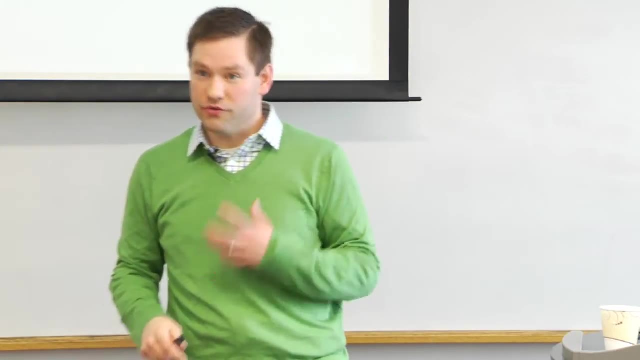 At the moment it does not yet have the real-time dynamic optics in it, but it does have a key requirement for that, which is that we're using laser light, which is important for when we're trying to do diffractive optics. 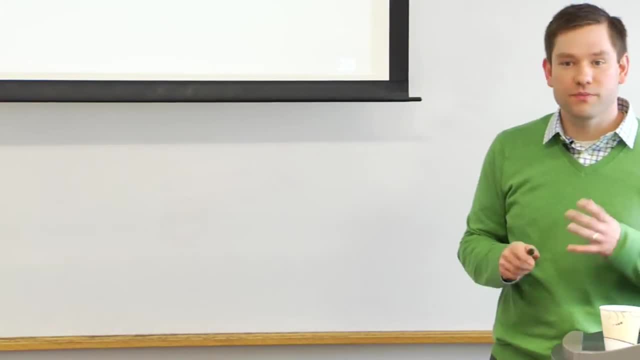 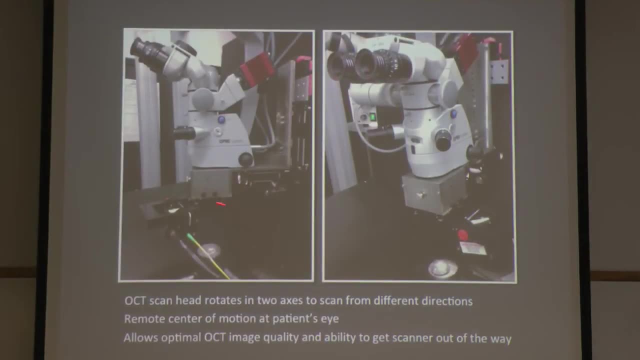 And I'll talk a little bit later about some of the important contributions we've made to imaging with laser scanning projectors. And just to demonstrate, we can use that remote center of motion to swing the scan head out to one side. the other side. 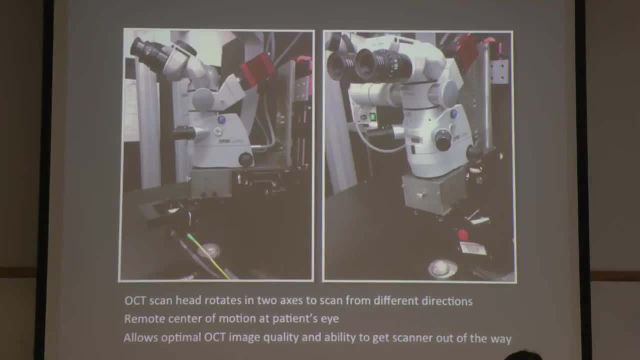 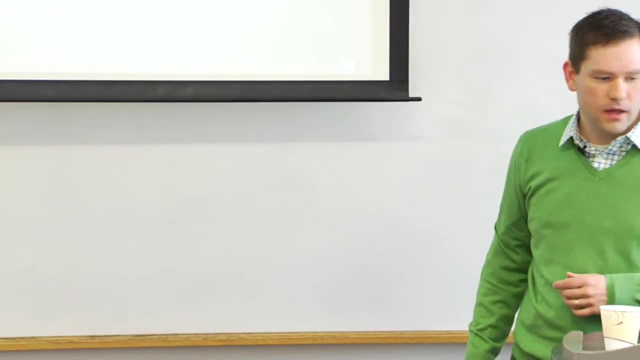 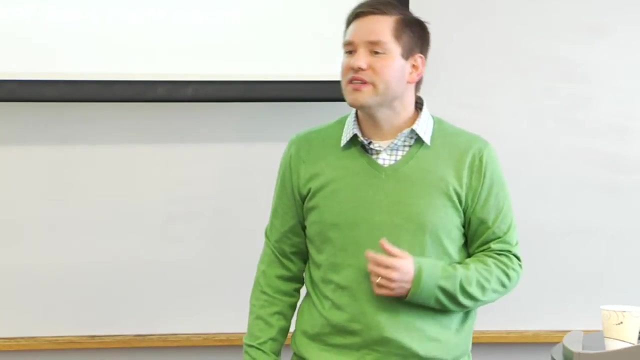 We can image all the way around the patient's eye to see any clock hour of it that we want to, while keeping the microscope stationary and knowing where the system is, And then we can use that to do the laser scan. So, to summarize, we have a lot of things that we're doing that are very small and very bright. 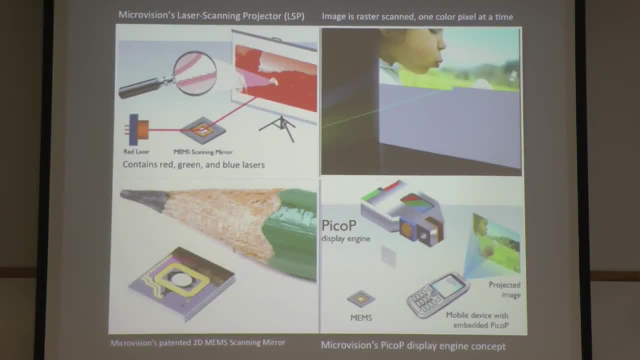 Our approach is to repurpose a laser scanning projector. In particular, we're using Microvision's Pico-P engine. Some of the other people here use these things for structured light applications. The basic idea is they use a MIMS mirror to steer a three-channel color laser beam to. 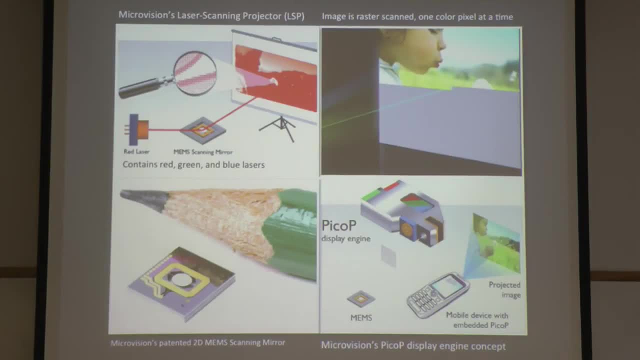 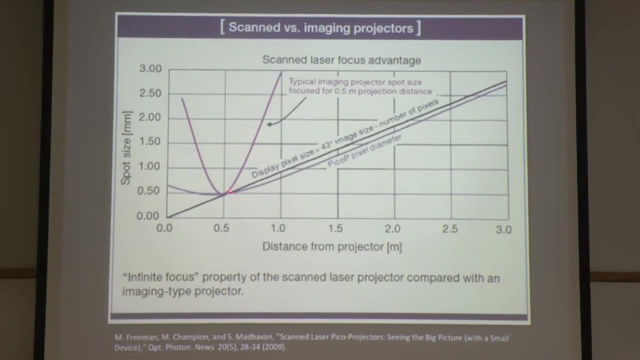 raster scan each pixel one by one in an image, And this is nice in most purposes because the image stays in focus from some short distance to relatively long coherence length, And it's very bright and very small. Now in this figure, what we see is a contrast between a normal projector like the one I'm 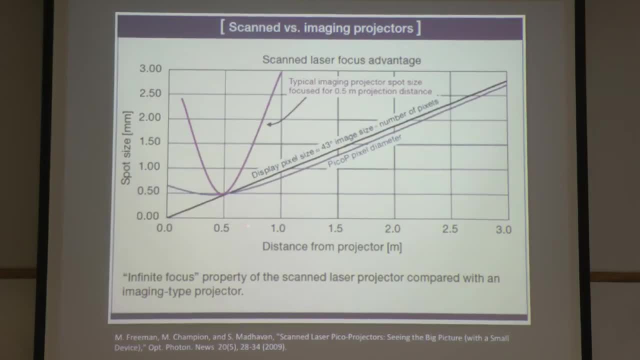 using for PowerPoint right now, which has to be focused And for a given projection distance such as this one, the projector is only in focus at exactly that distance. If I move the projector or the screen forward or backwards very quickly, it blurs. 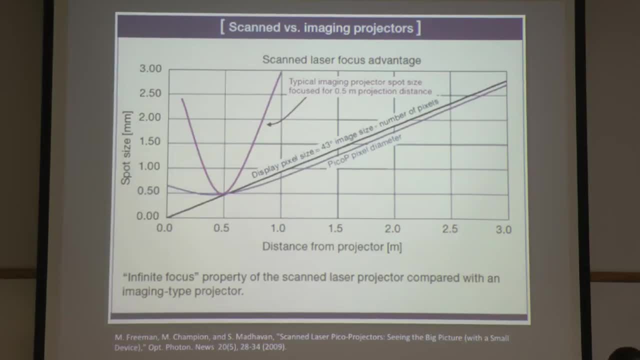 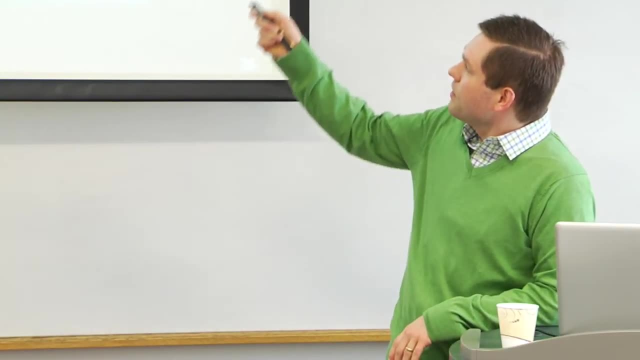 And the pixel size going up here, or spot size, gets way too big. Your one pixel overlaps the next pixel. The spot size is larger than the pixel. That's the pixel spacing. The laser projector follows this line here where, from half a meter out until basically, 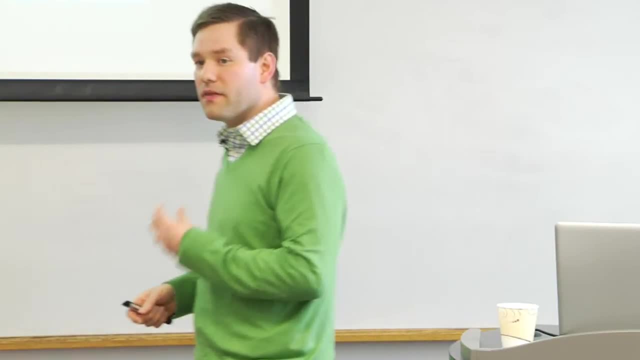 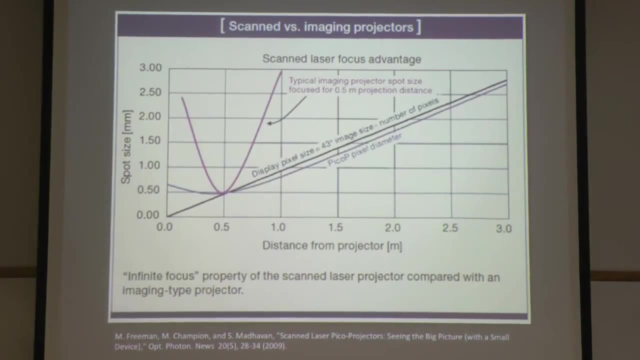 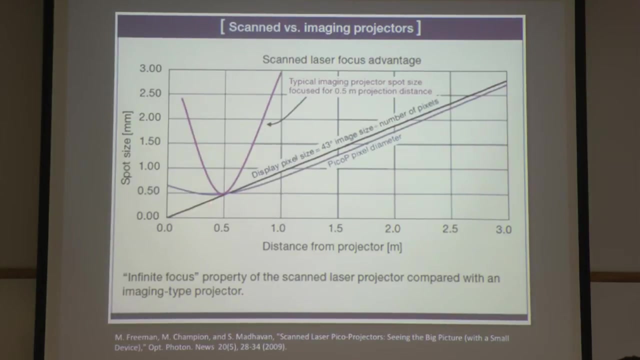 infinity. the spot size is slightly smaller than the pixel spacing, And so each pixel doesn't overlap its neighbor. We have a nice, sharp image Now. unfortunately, Gaussian optics, that is, optics using laser beams, have some unusual properties with them in terms of how the waist of the laser beams behave. 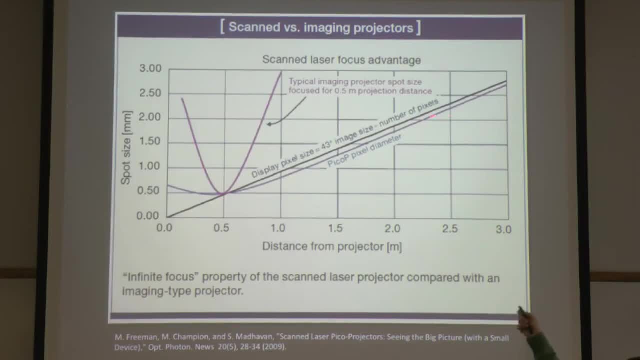 And so while they put the waist here at half a meter, they get this nice, slightly larger property going out. You can see that the laser beam suddenly gets larger as we go. less than half a meter, And this is. we want to be operating right here practically on this axis, at very small. 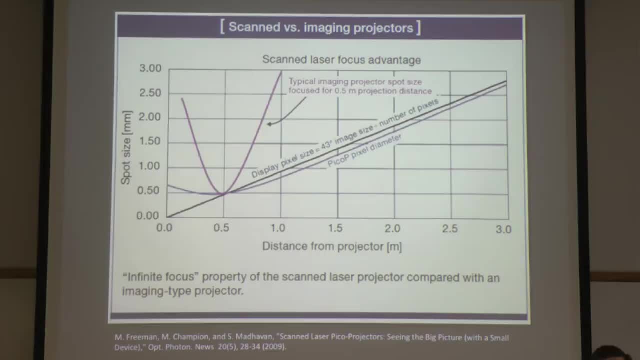 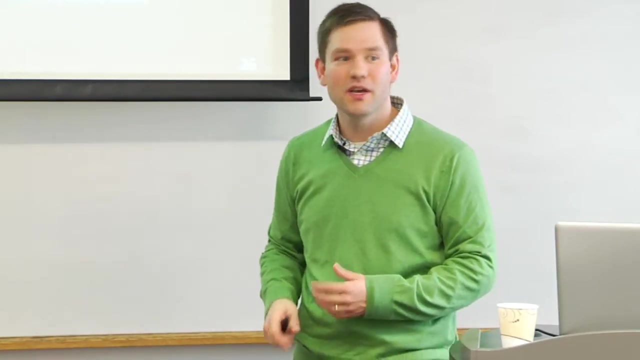 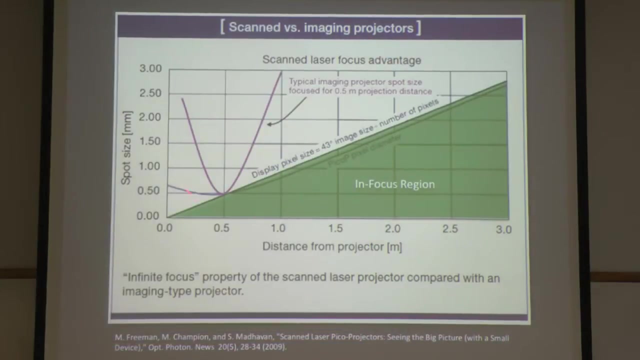 images Distances like a centimeter or less, At which point, using our existing system, we'd have the entire each pixel basically be superimposed on all of its neighbors and not at all usable. So we want to take this in-focus region here and somehow find a way to take this in focus. 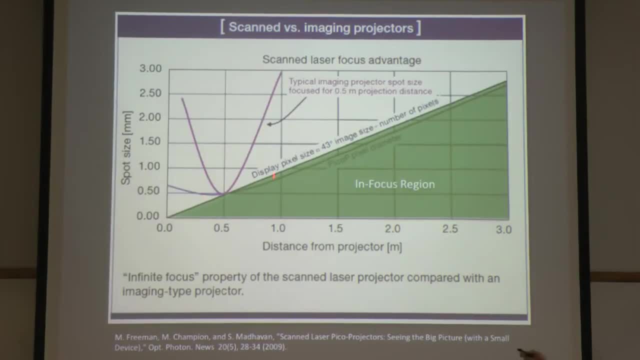 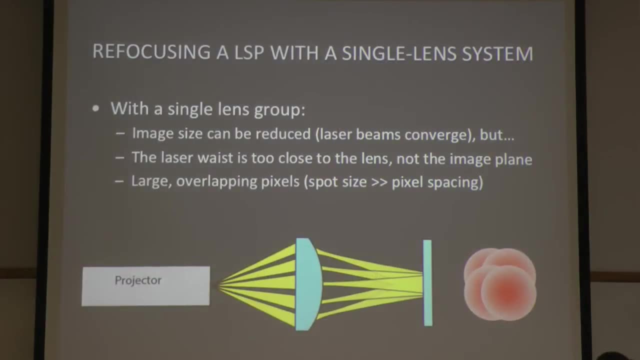 find a way to take a laser scanning projector and treat it like a regular projector where we can refocus it. but down in this region We unfortunately can't do that using a single lens. We can't do that because we have two different optical phenomenon happening. 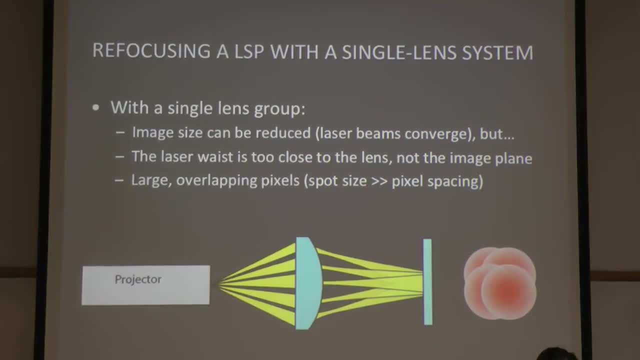 One is the pattern of the laser beams themselves, how the image is spreading out, how the laser beams are pointed. The second is the beam width and profile of the individual laser beams. If we try to take the laser beams and refocus them down to produce a small image, we're 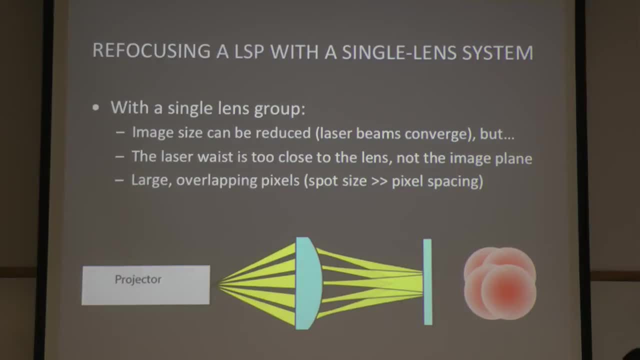 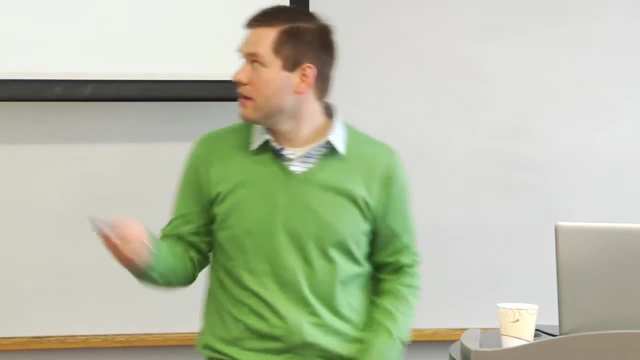 never going to be able to get the laser beam also to have a small waist at that image location. The image waist is always going to be closer to the lens than where we're trying to image it, And the smaller the image we try to create, the closer the waist of the beam will be to. 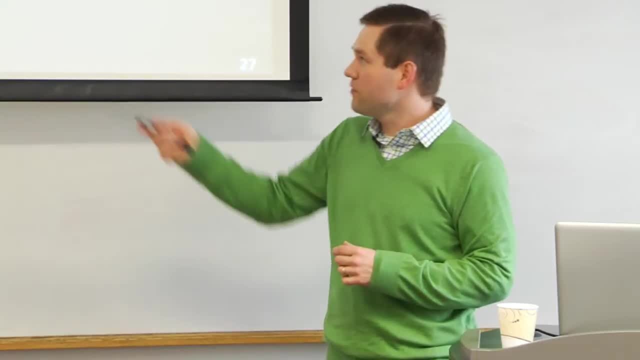 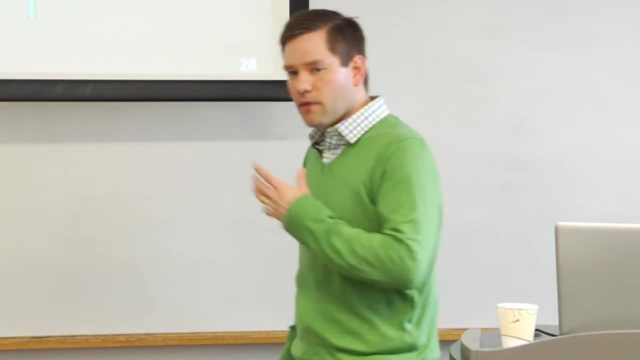 the lens and we're never going to get the waist small enough. even if it's right by the lens, the waist will still be too fat to get high resolution images. RIPHT student Sam Horvath. RIPHT student Sam Horvath has been working under my supervision to produce the world's 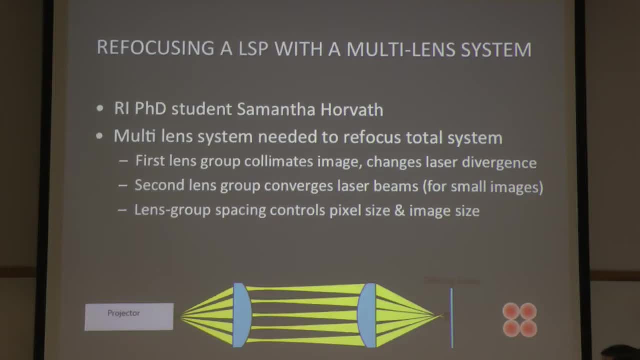 first system for refocusing an LSP, And the key trick here is that we use two different lens groups to be able to gain degrees of freedom to independently control the orientation and path of the laser beams and the cross section of those laser beams as well. 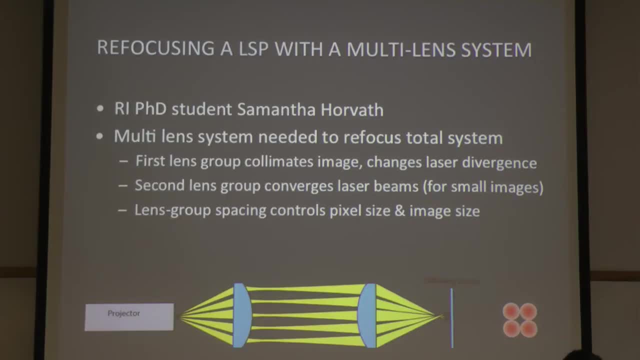 And we arrange it in a special setup where the first lens collimates the laser beams and the second lens then causes them to converge, And so the spacing between these lenses is very important. RIPHT student Sam Horvath. RIPHT student Sam Horvath. 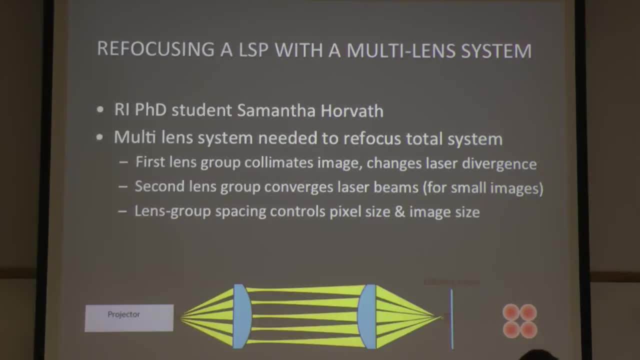 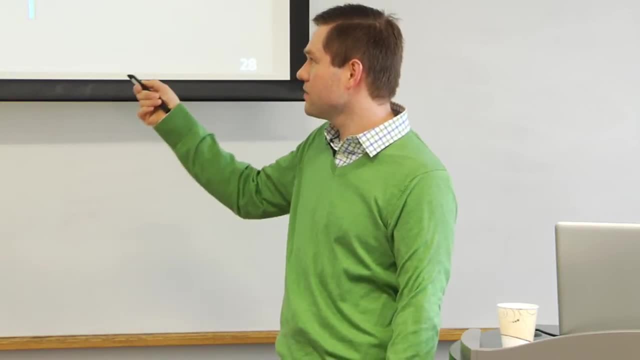 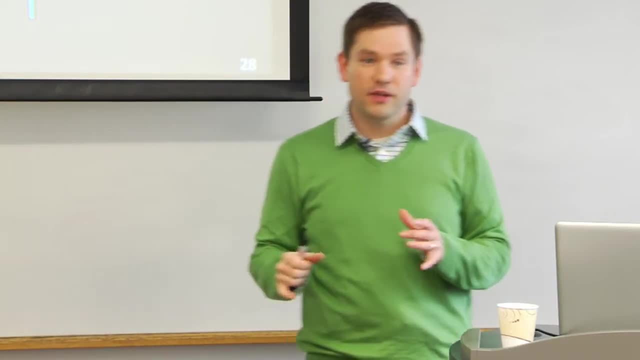 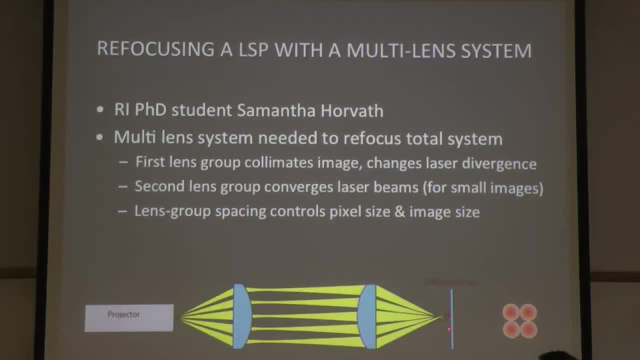 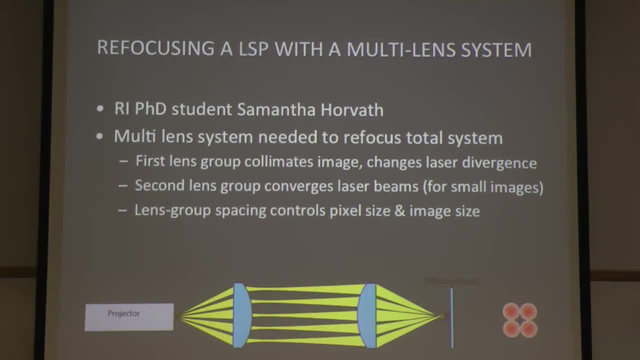 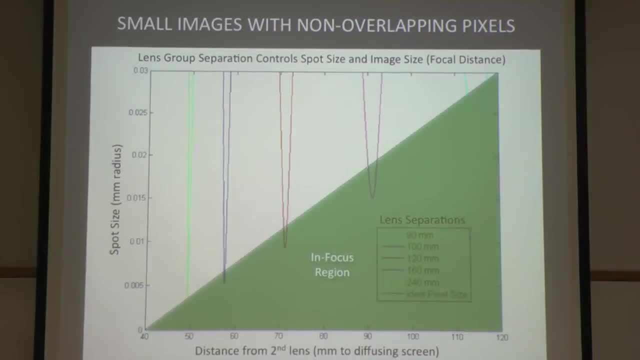 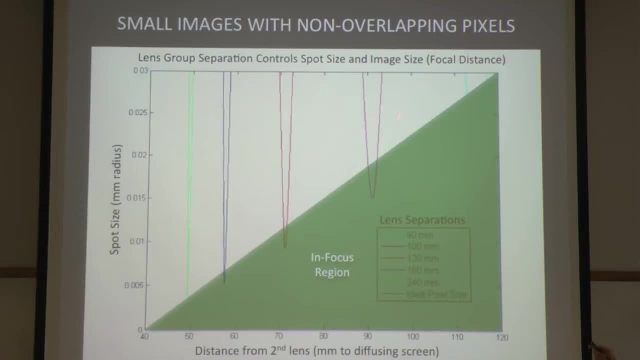 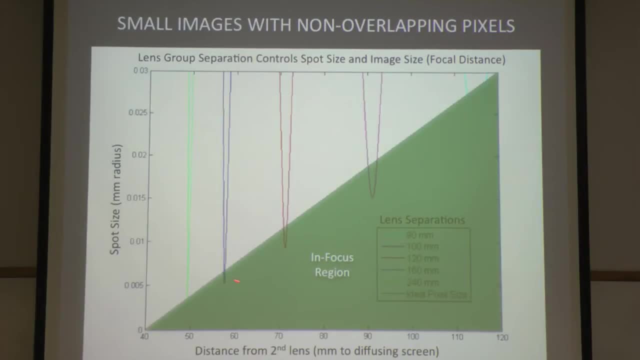 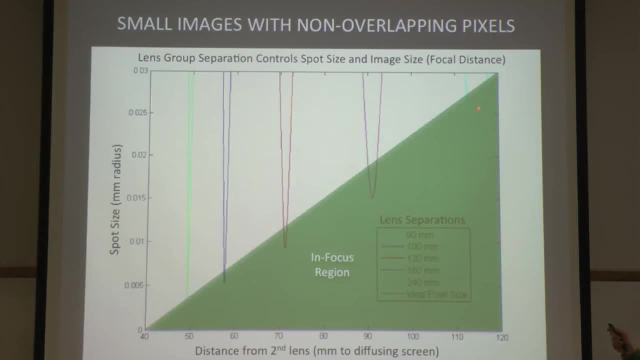 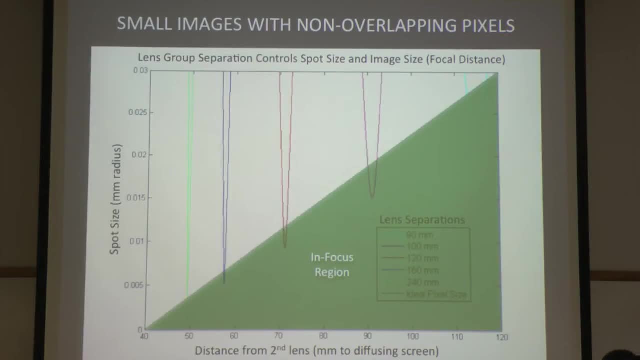 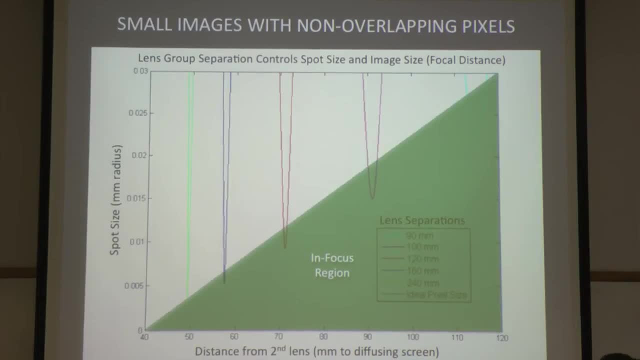 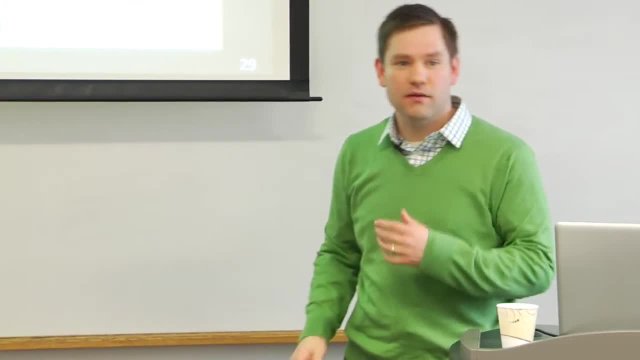 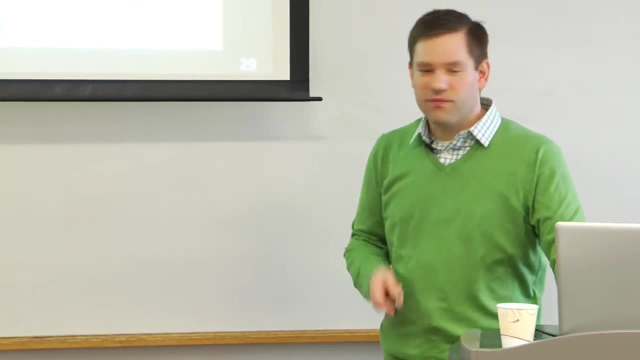 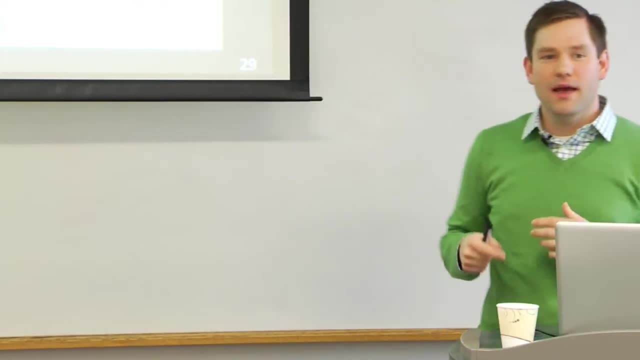 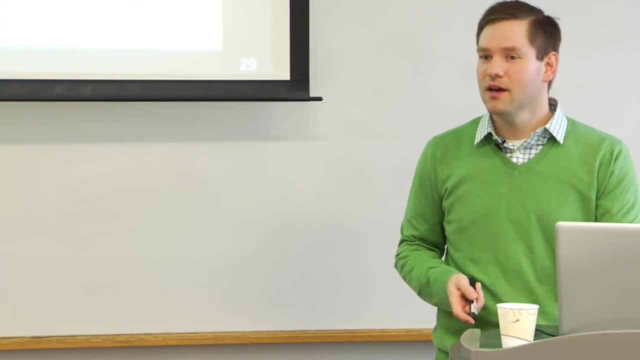 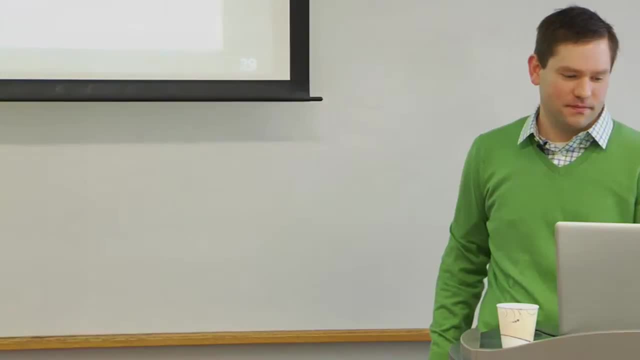 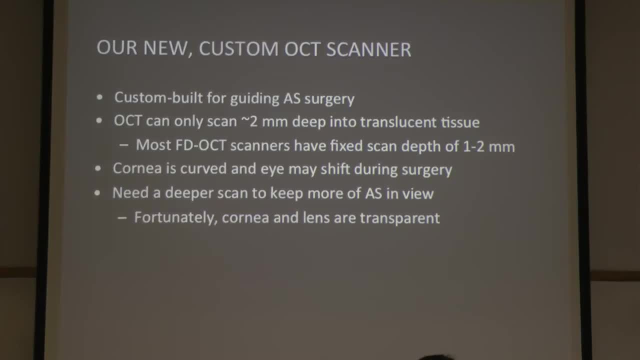 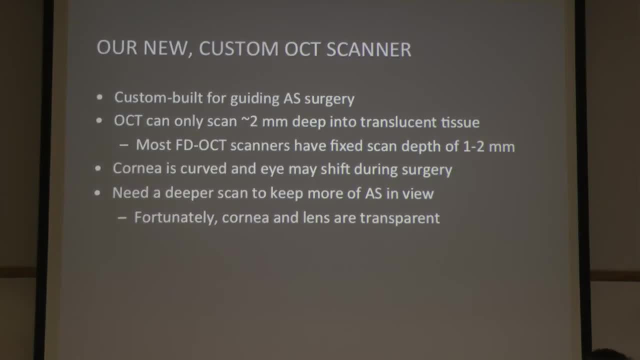 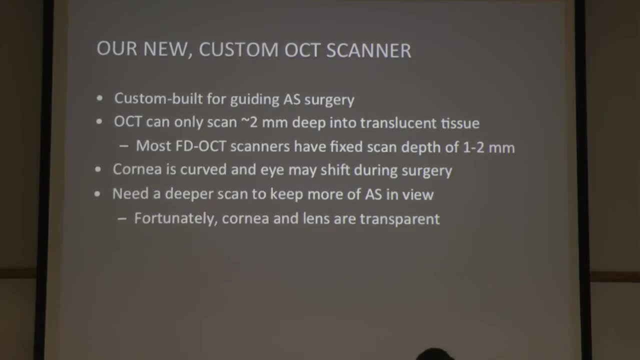 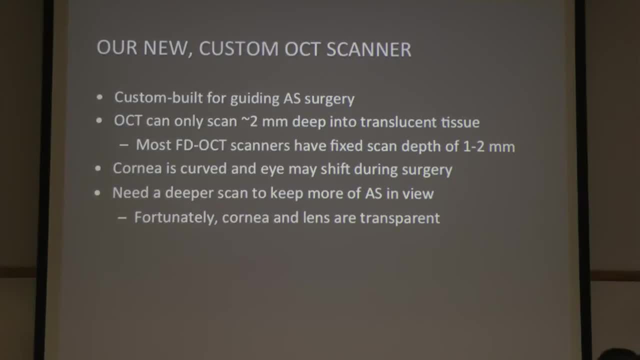 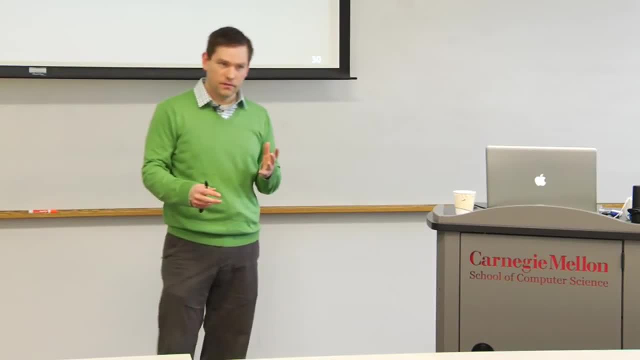 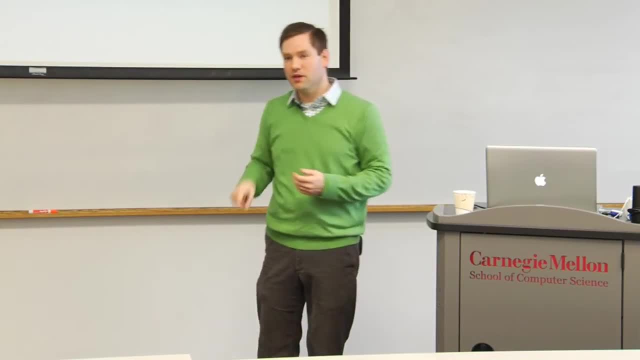 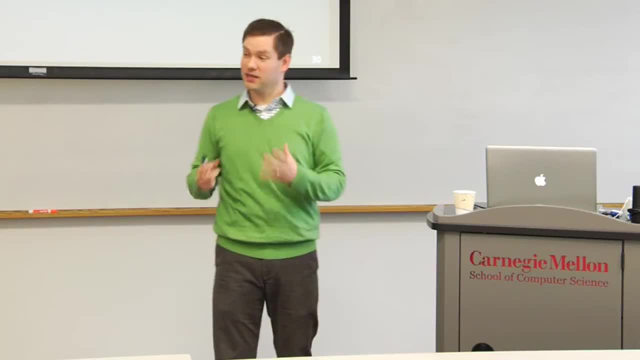 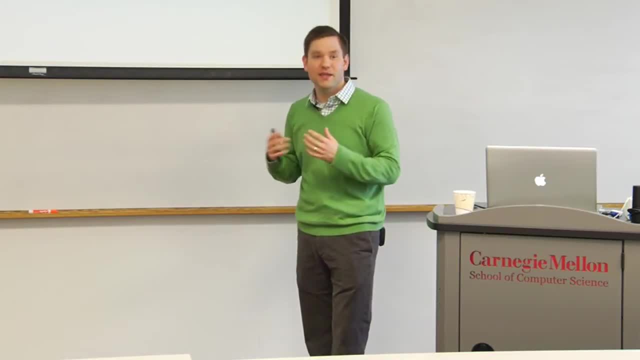 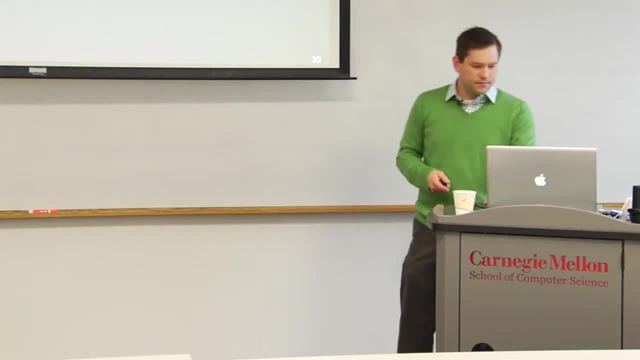 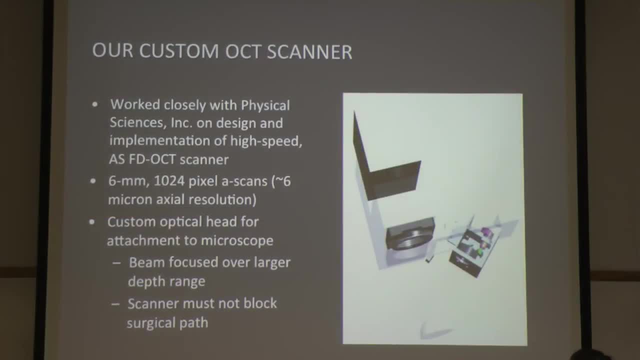 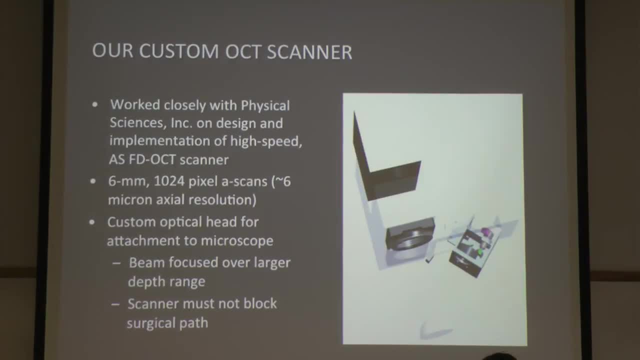 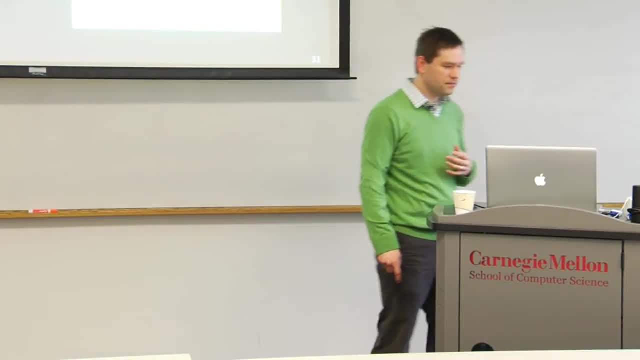 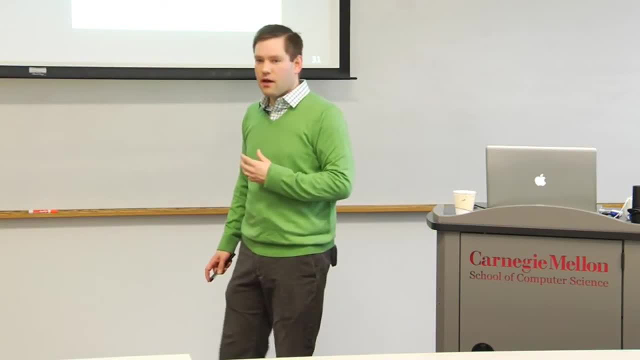 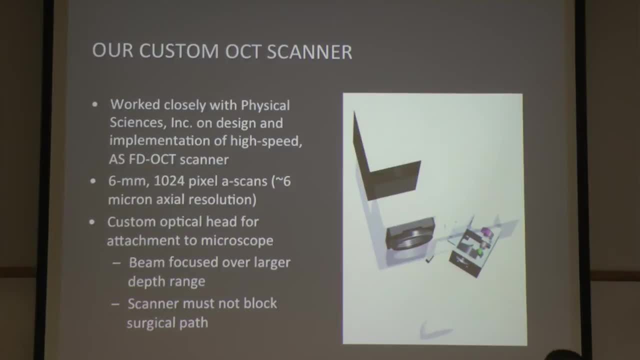 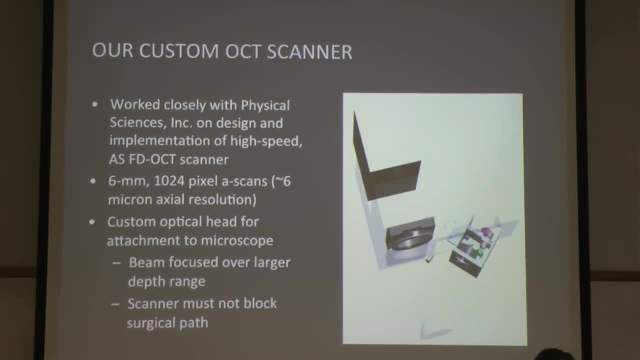 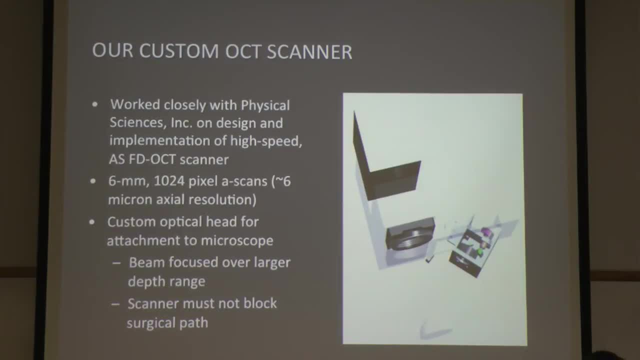 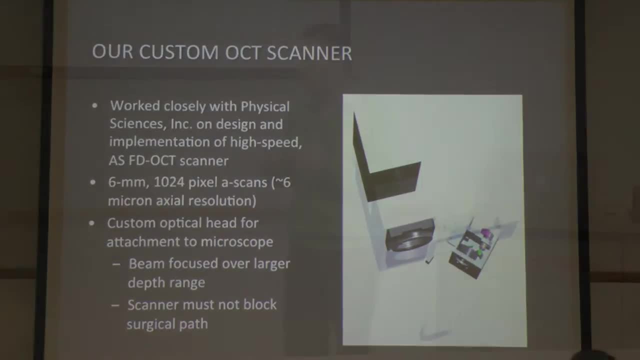 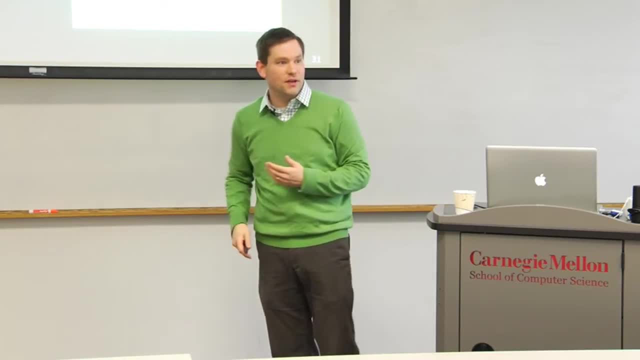 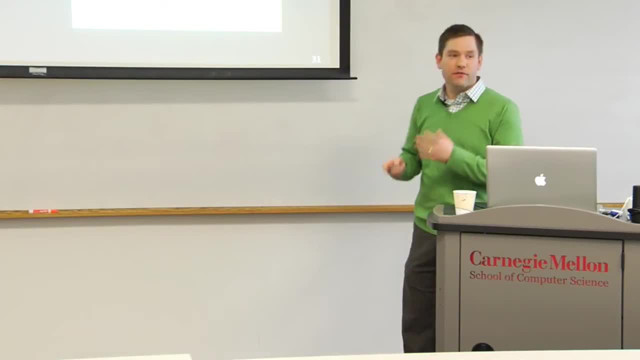 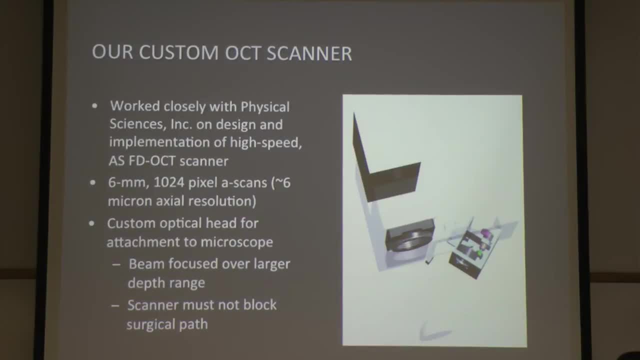 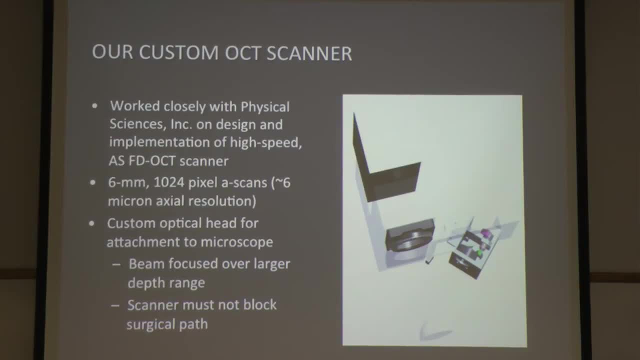 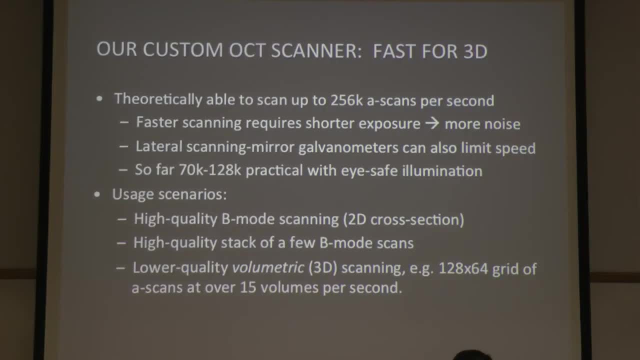 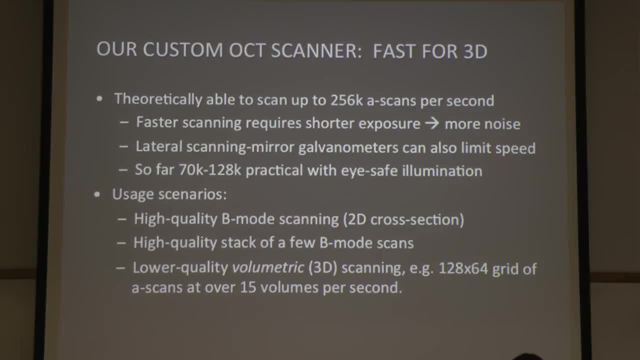 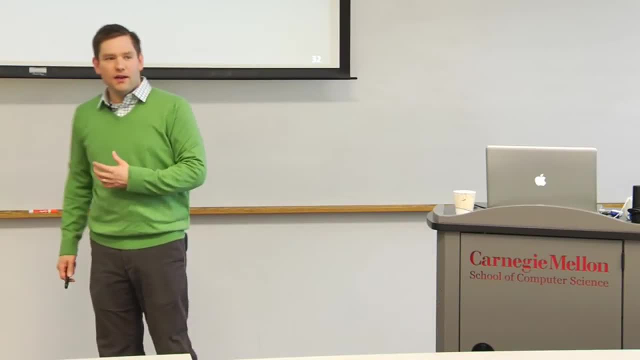 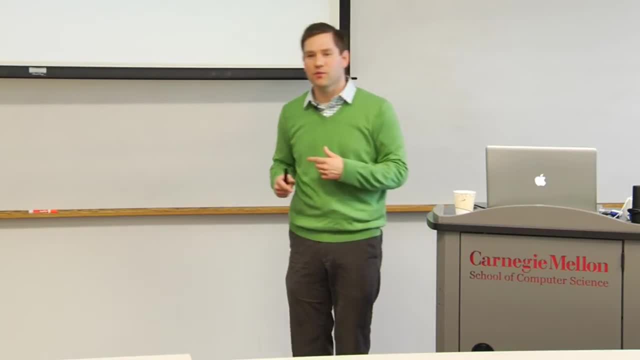 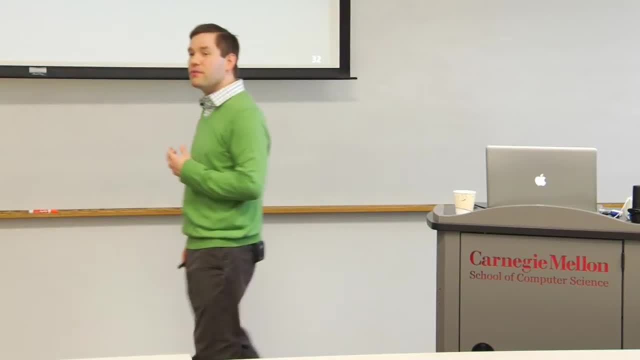 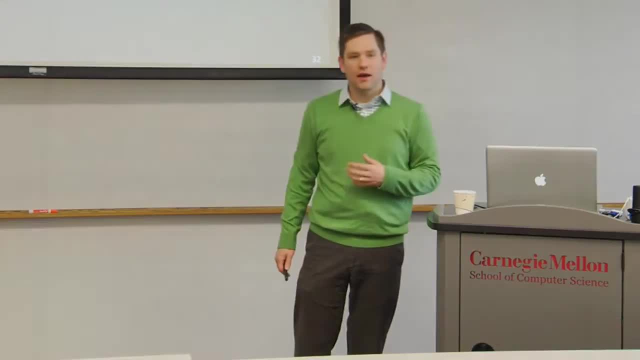 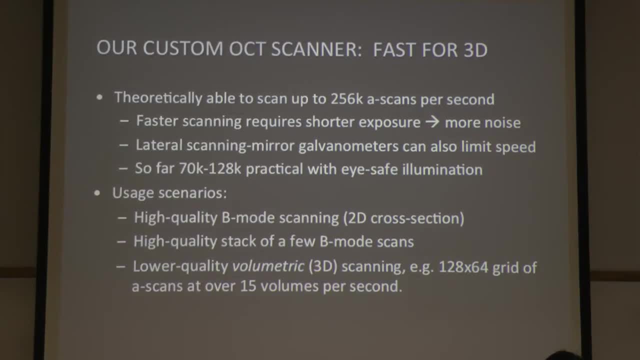 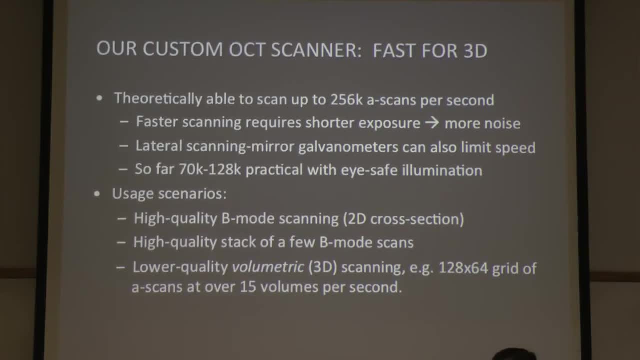 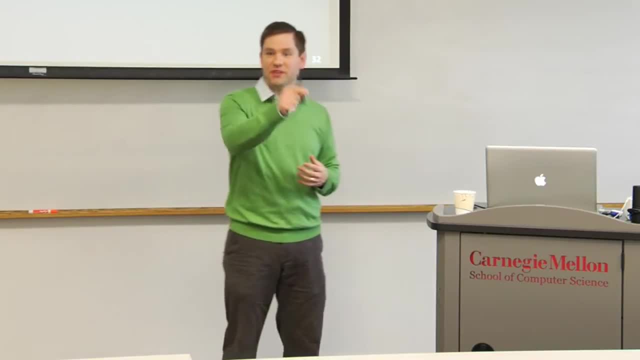 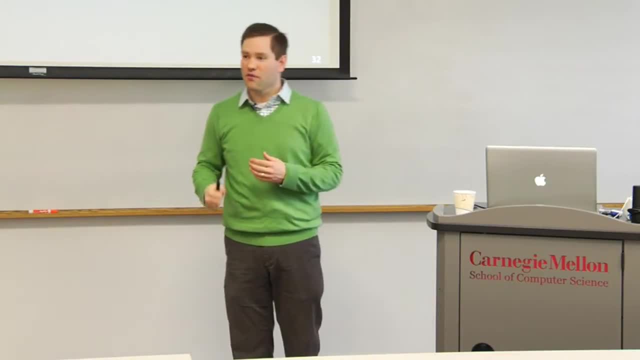 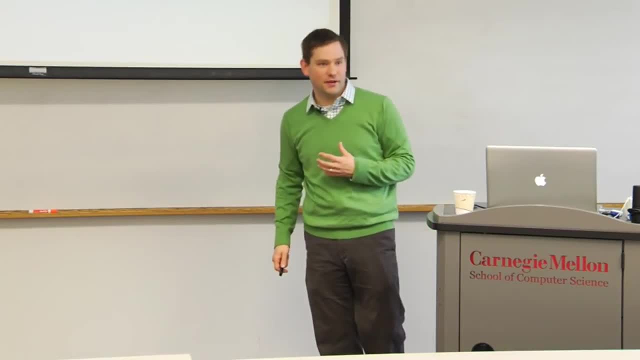 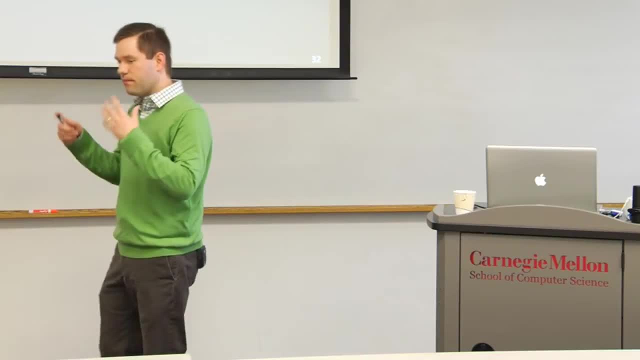 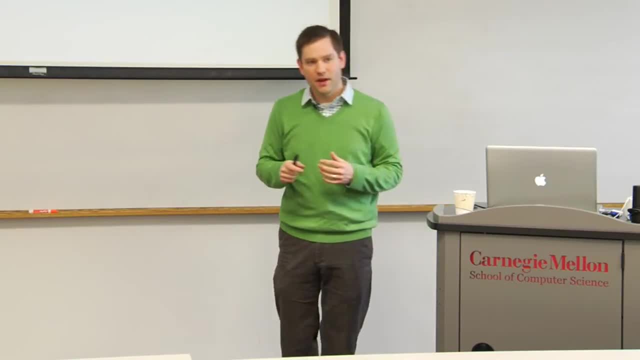 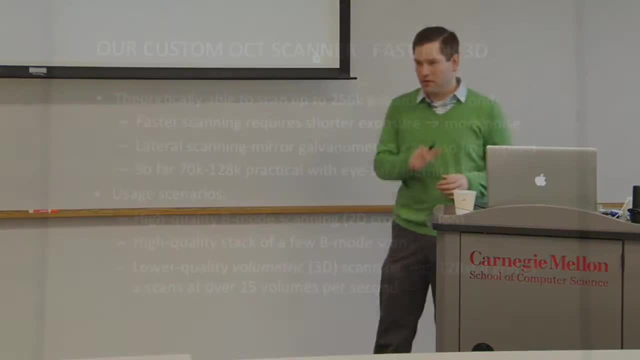 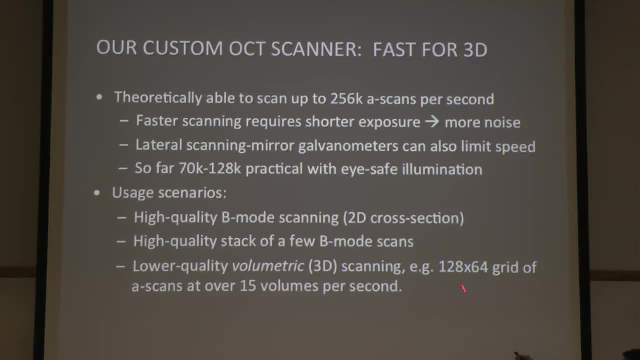 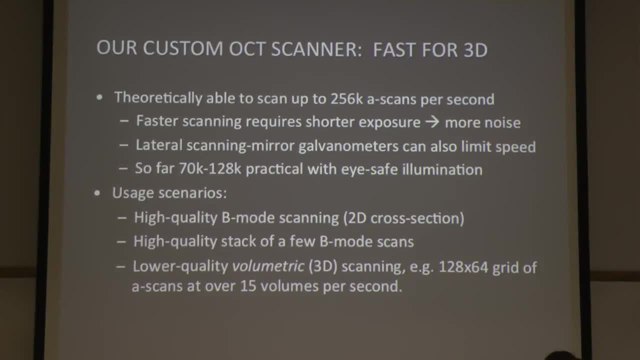 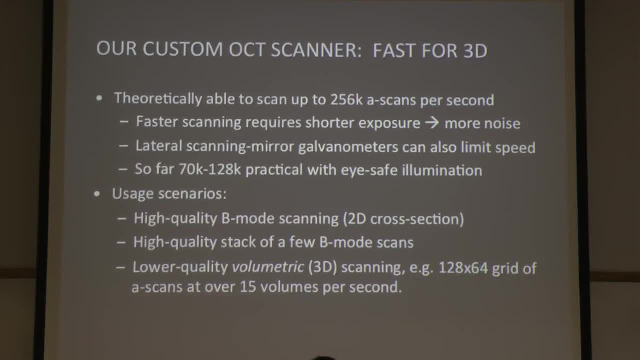 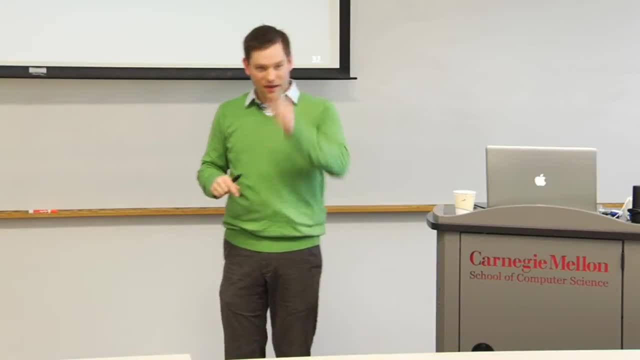 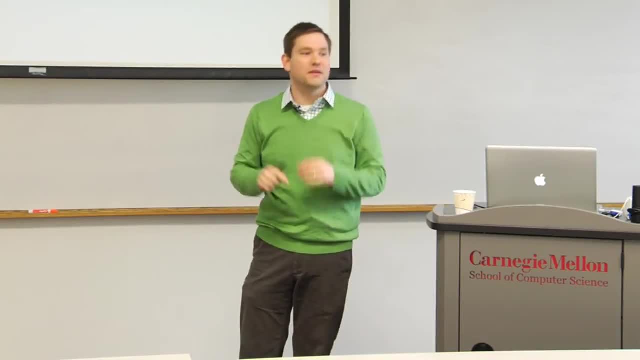 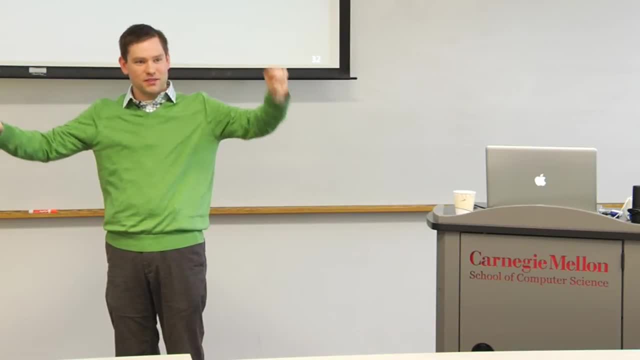 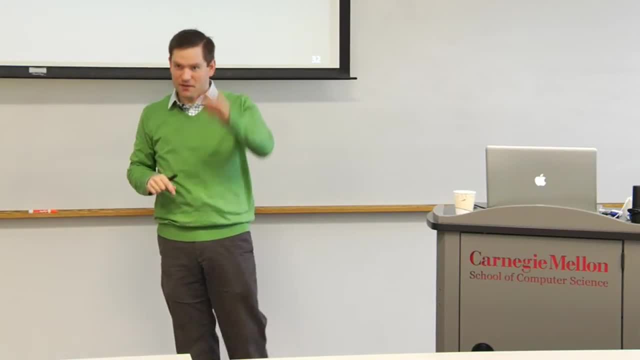 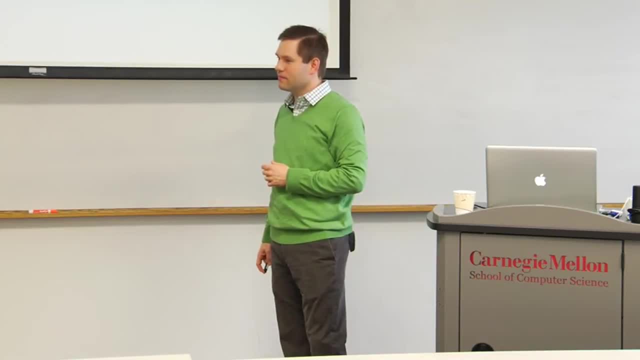 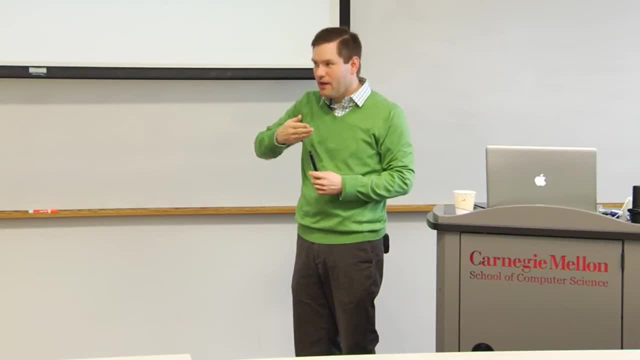 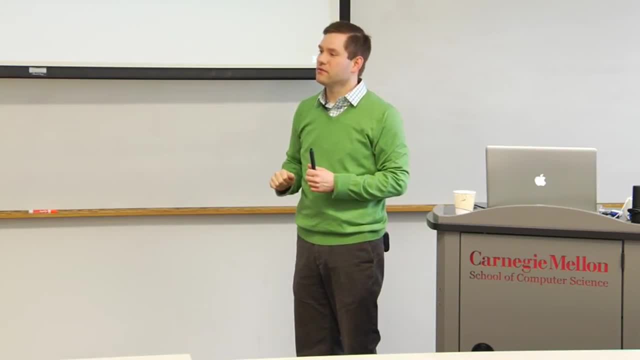 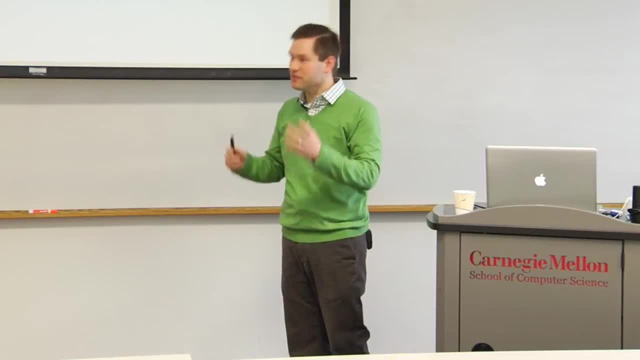 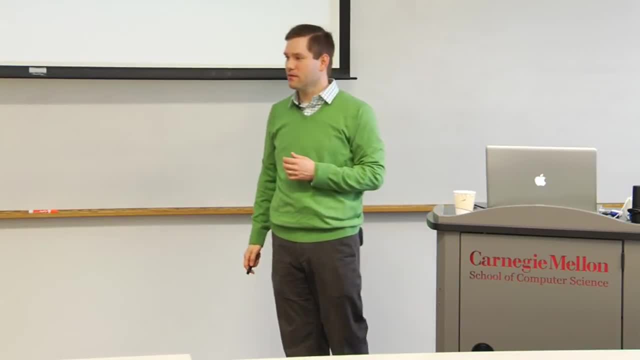 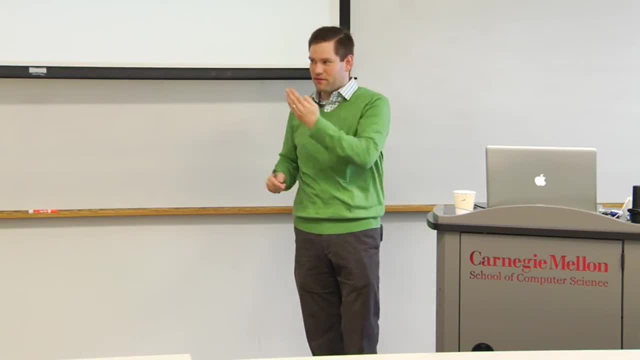 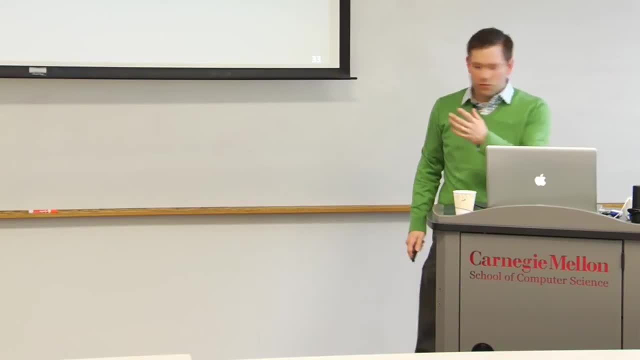 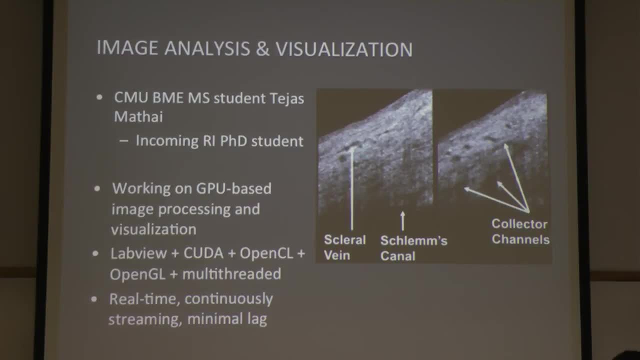 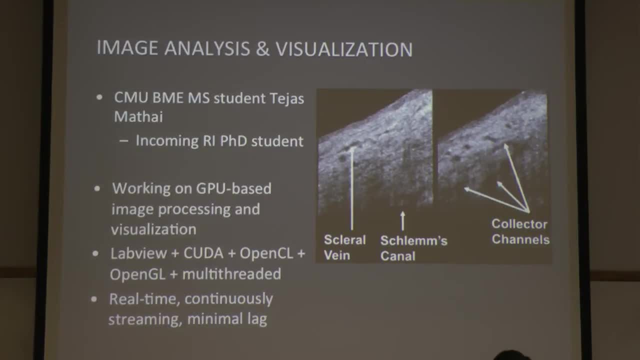 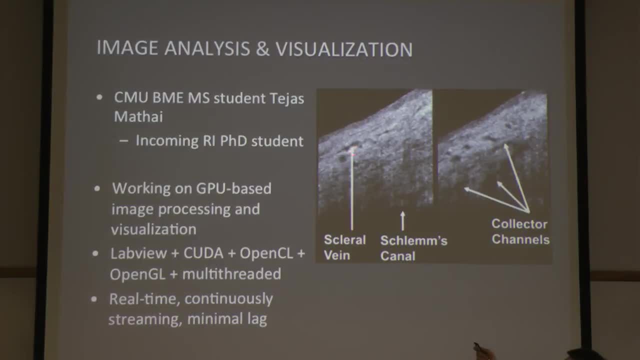 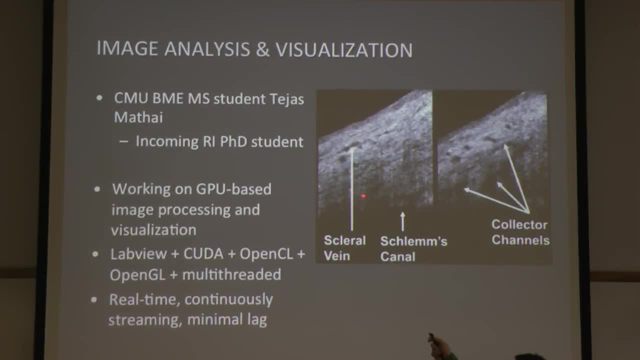 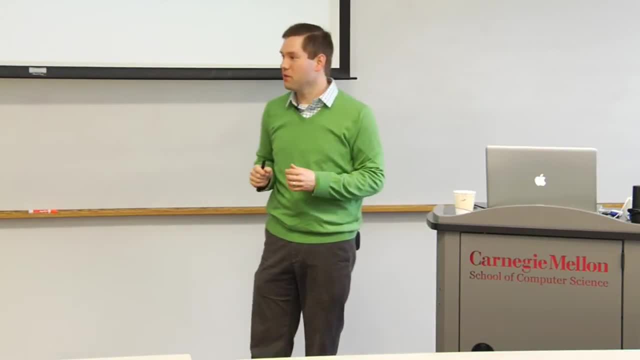 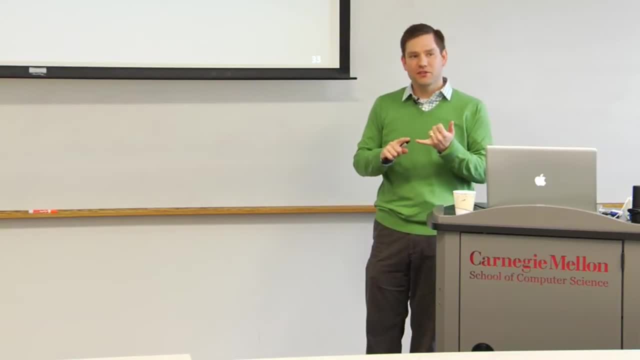 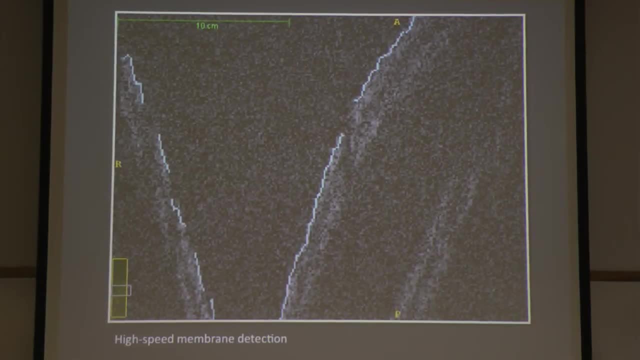 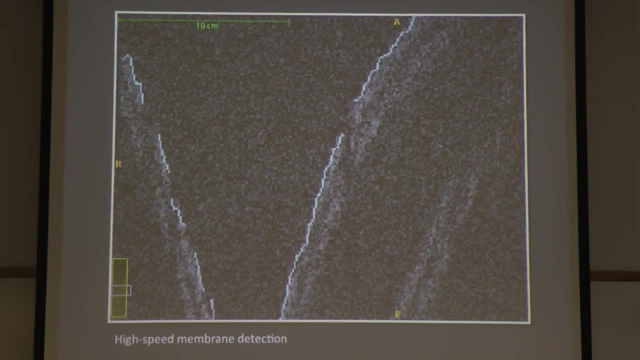 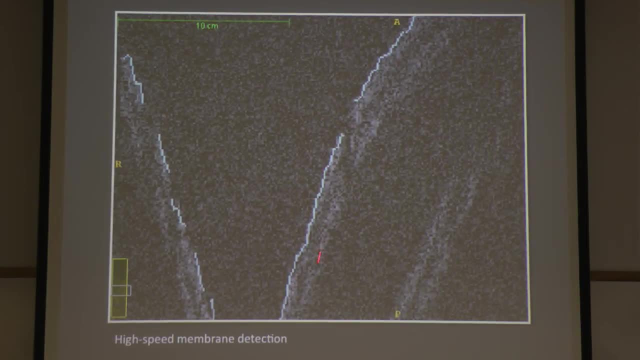 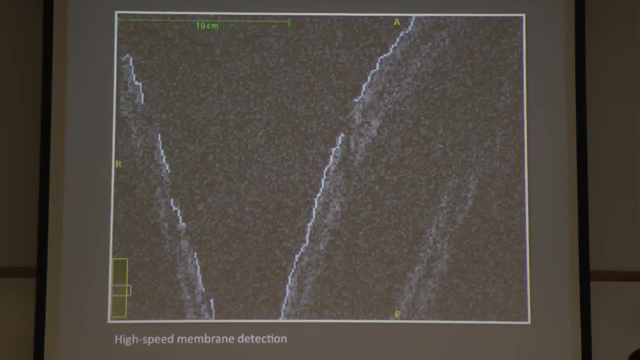 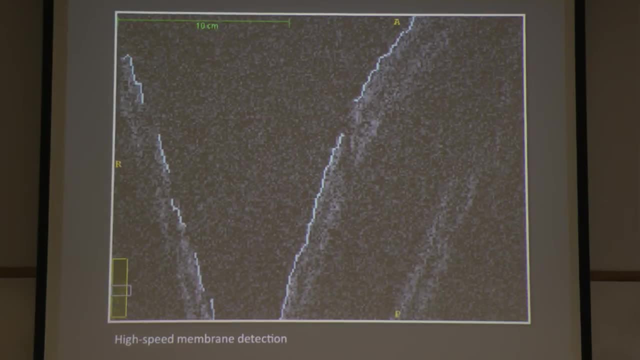 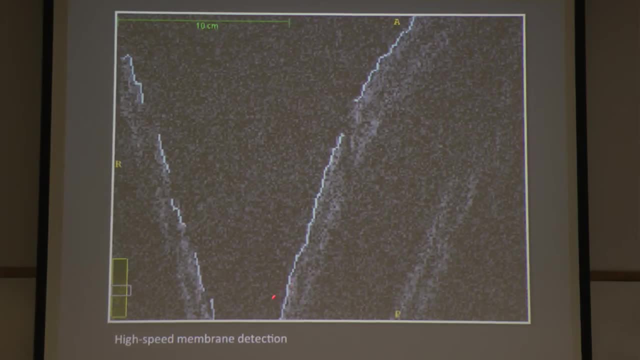 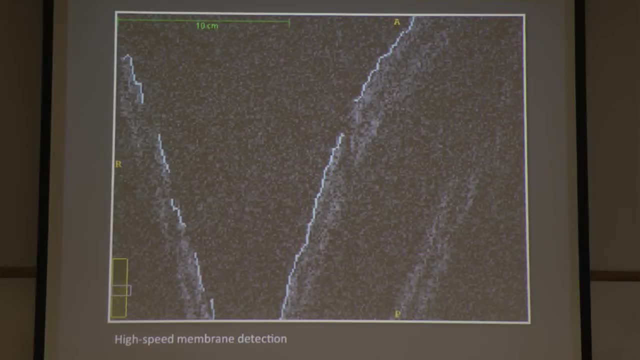 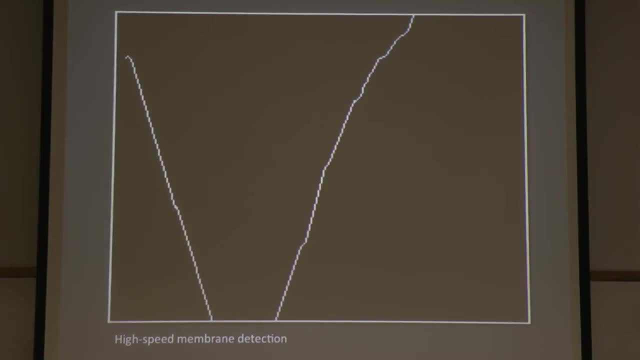 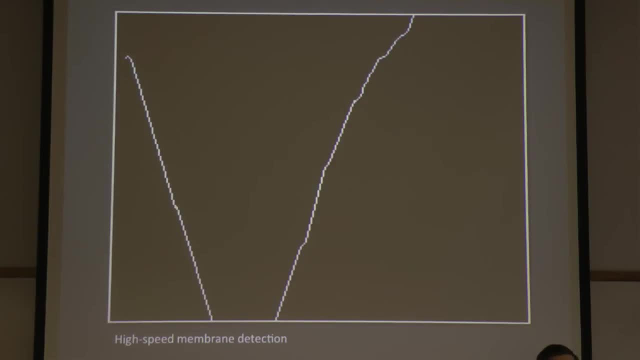 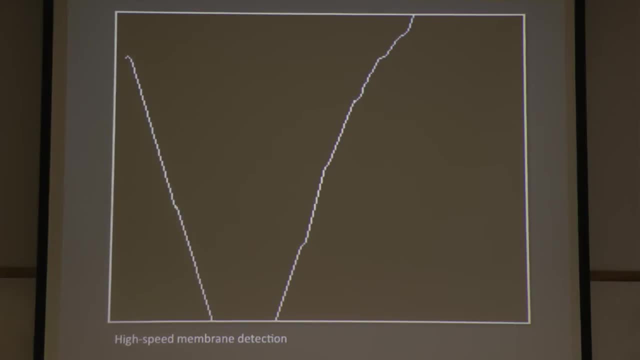 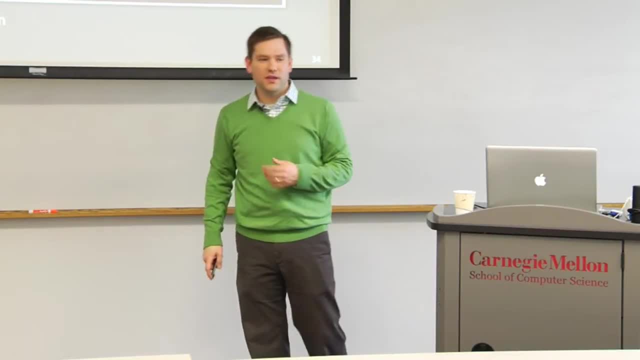 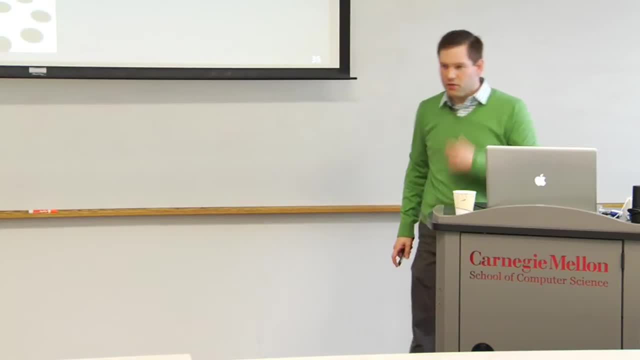 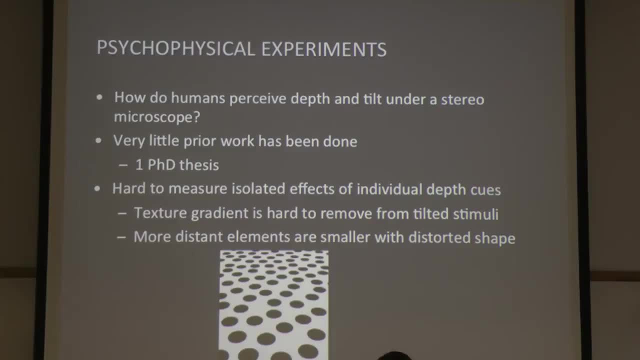 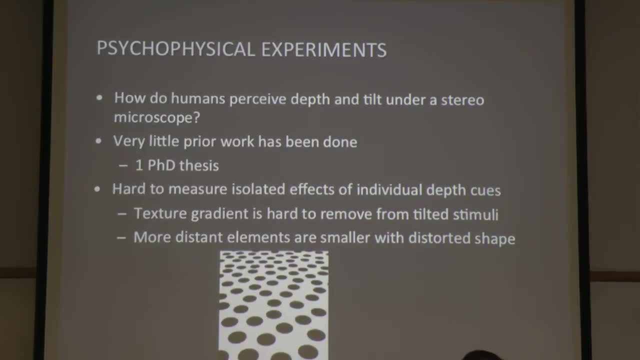 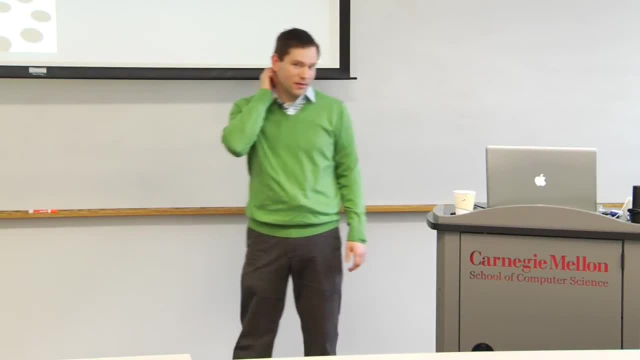 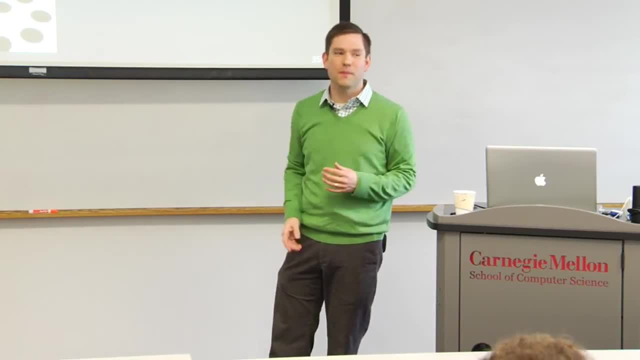 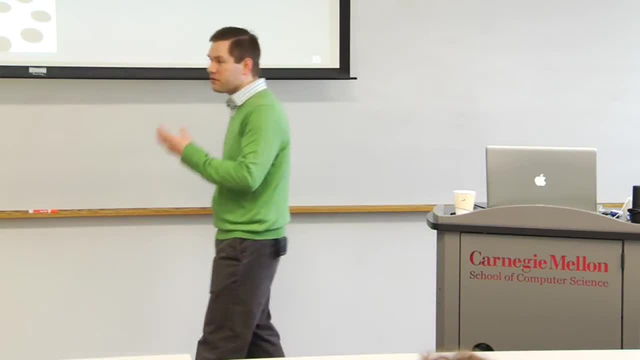 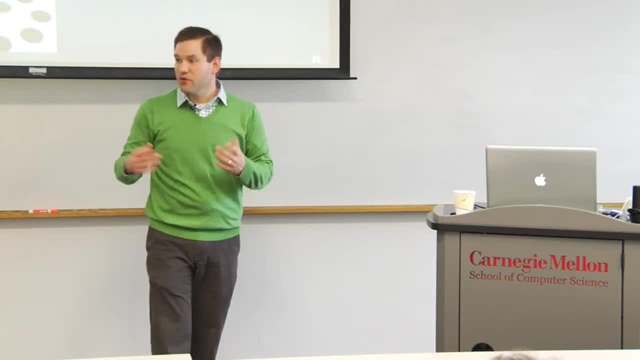 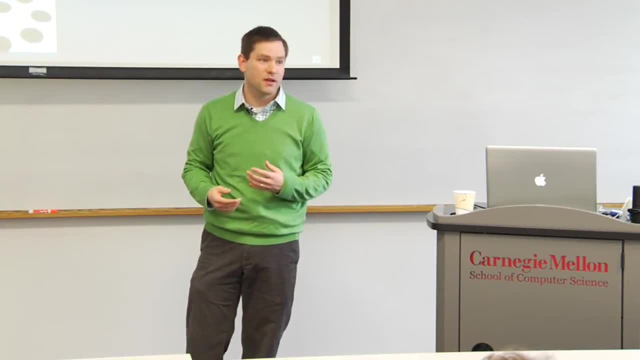 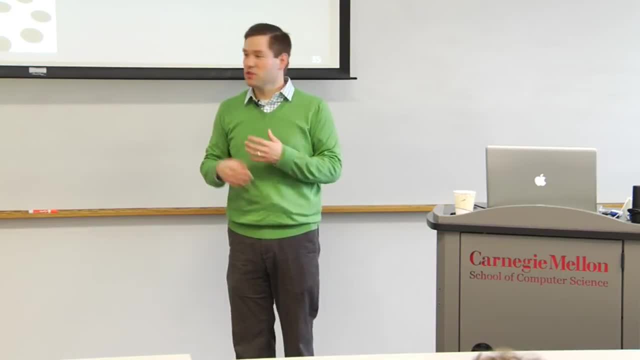 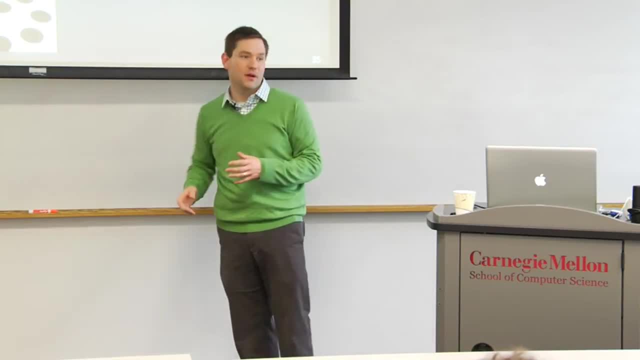 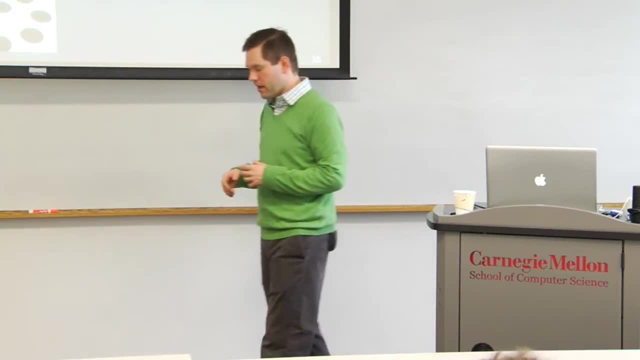 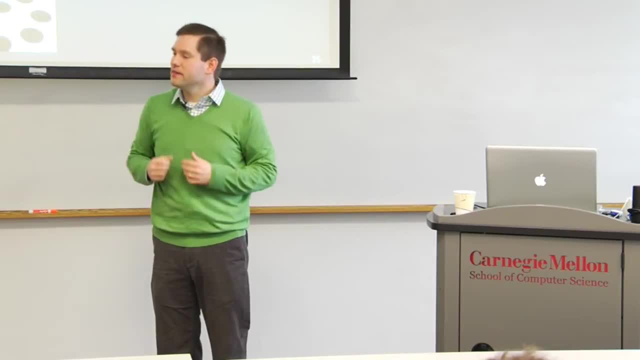 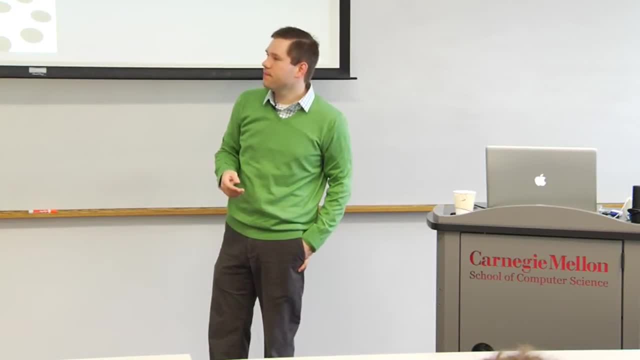 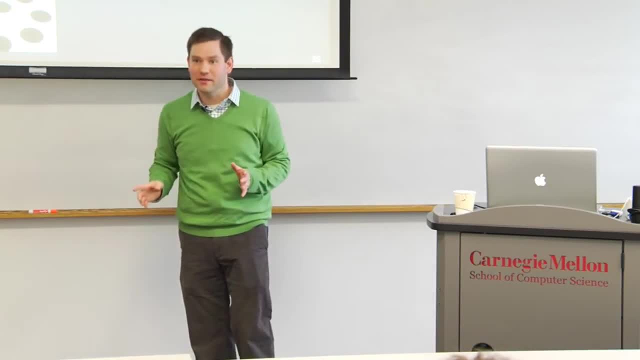 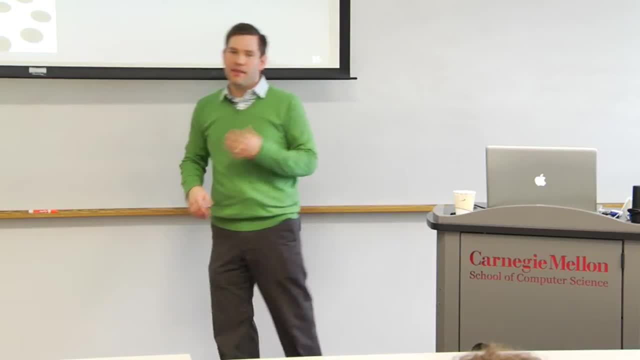 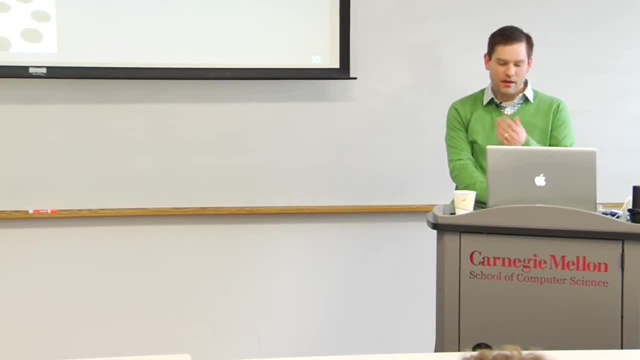 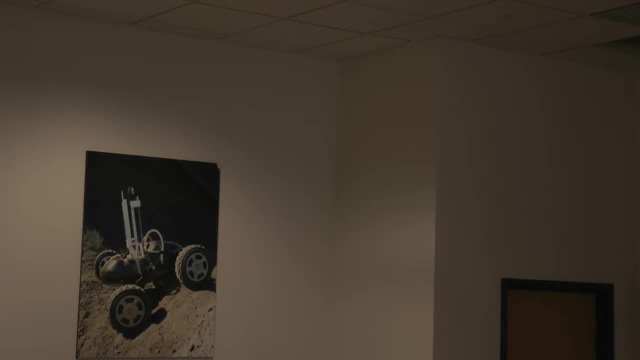 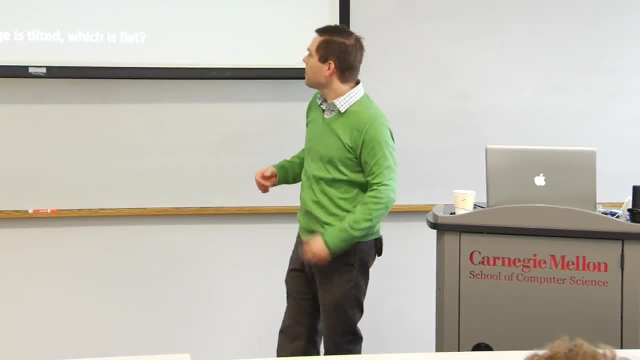 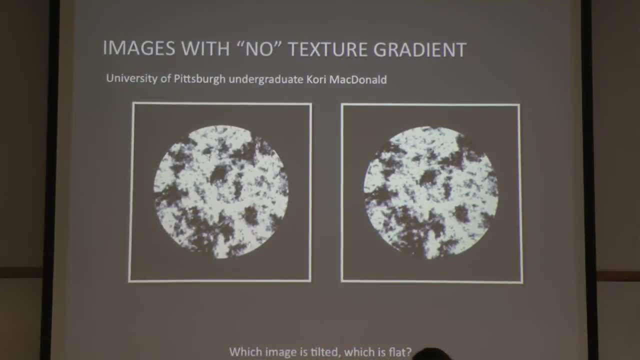 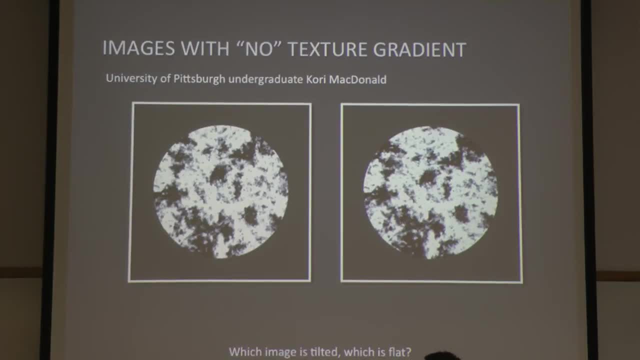 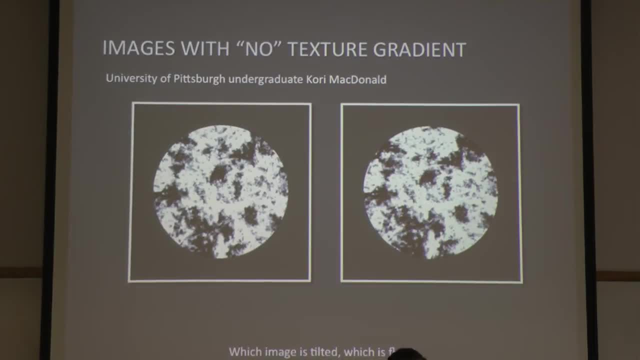 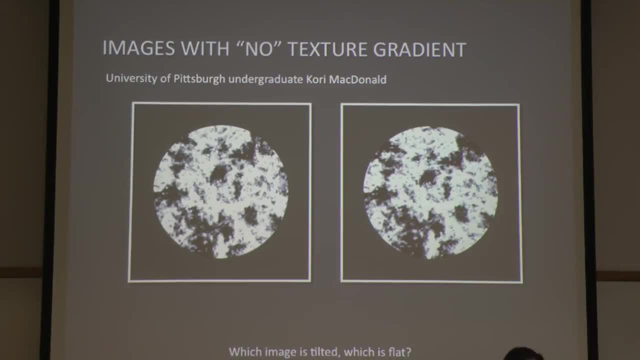 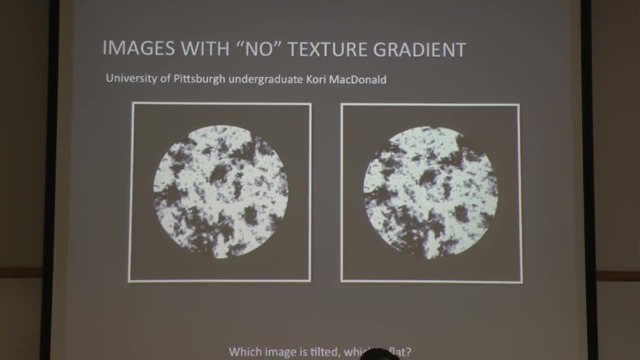 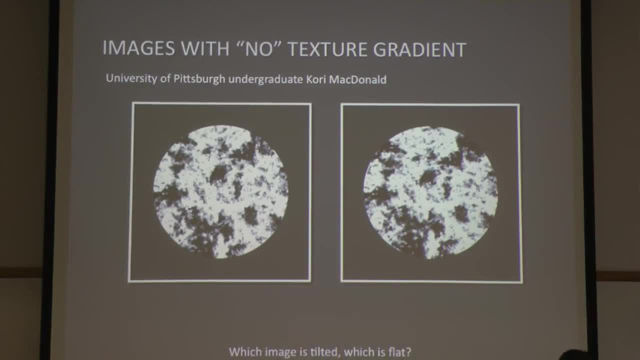 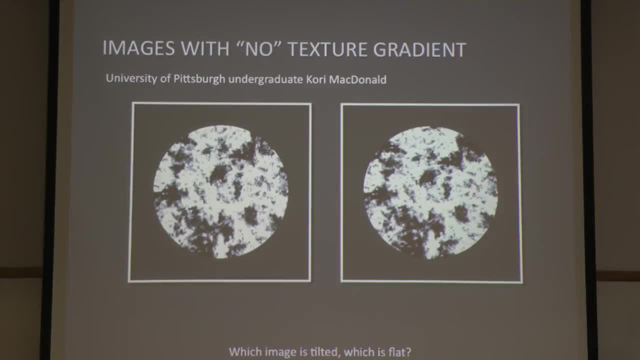 and when you look at that, I presume that you cant really tell which is which. But in fact the one on the left is flat and this one is tilted 30 degrees with the top towards you, But nothing there jumps out about it. 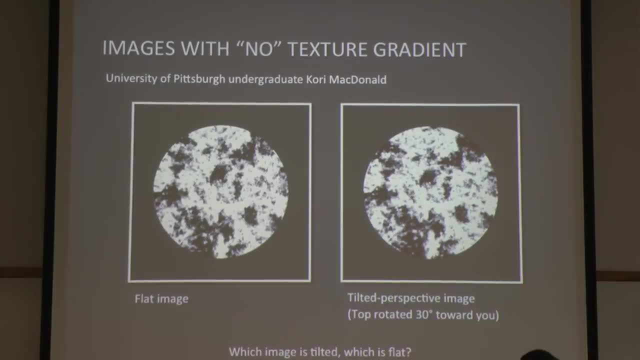 Now, and we've done extensive experimentation to show that nothing at all jumps out. There is virtually no information from these images you can use to tell which one is tilted the hardest, which one is the making slash. So there are a lot of jobs to do. 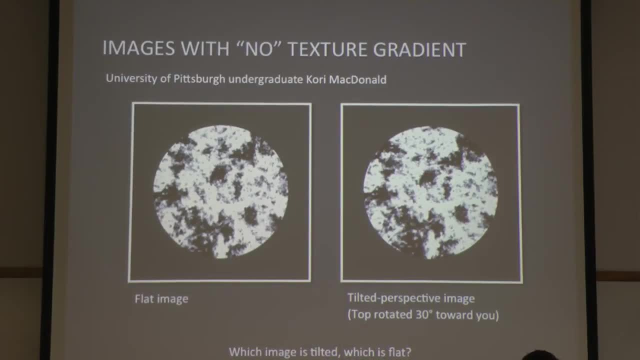 and which one isn't. But if we turn on stereo shutter glasses to allow stereopsis to work, people become very accurate at knowing exactly which one is tilted and which way it is, and so on. Visual system suddenly works nicely. Stereoscopic stereopsis works perfectly. 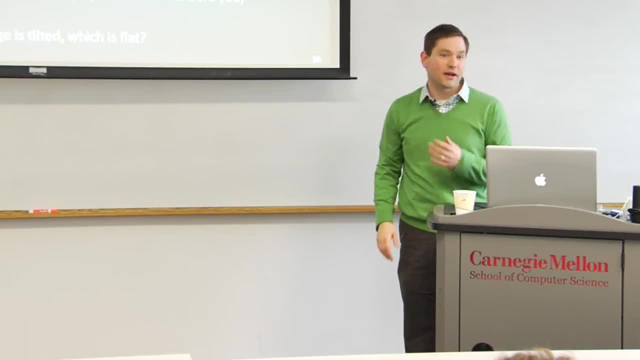 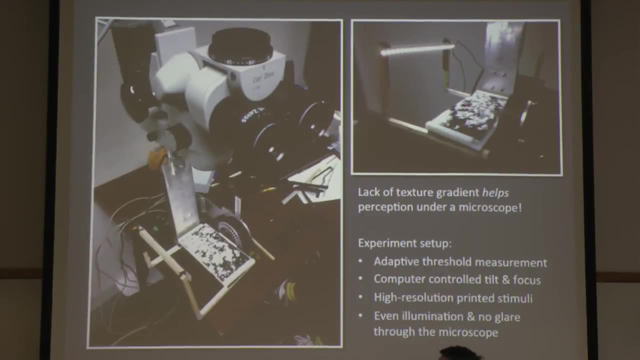 You can tell how it's tilted and do this to less than 15 degrees of tilt very accurately. We've then proceeded to take these images we've developed and validated, print them out at the highest possible resolution we can and put them on computer-controlled rotating stages. 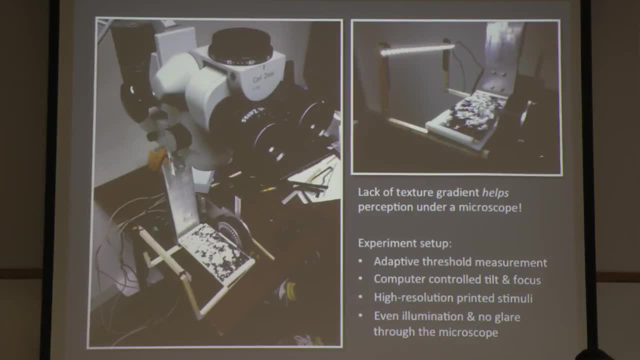 under a surgical microscope with controlled lighting to preserve exact lighting on the thing, regardless of how we tilt it, And we're just now starting to study how people perceive these things, And, while we don't have fully rigorous data that I can present on this yet, this is just starting. 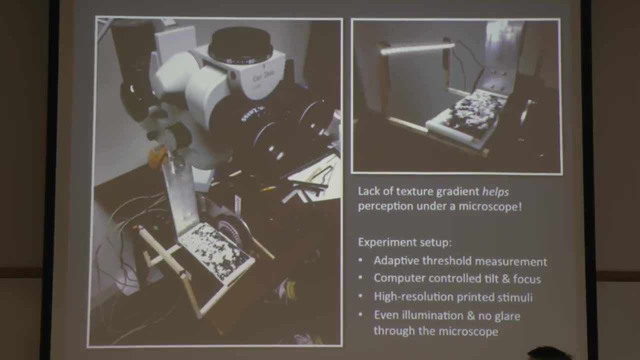 we believe it's reasonably safe to say that one of the key takeaways, to start with, is that people perceive tilt, position and orientation of these images better than anything else we could put under the microscope, Because they lack the pectoral cues that are misleading. 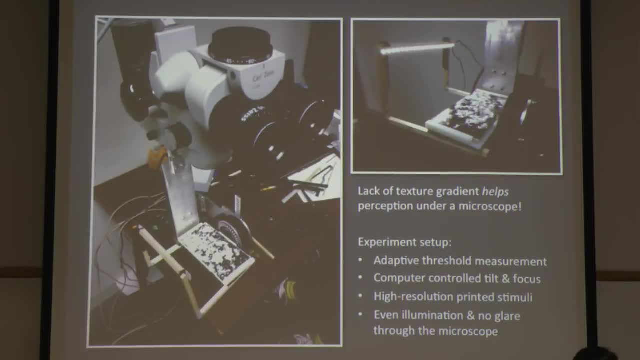 all that you have is a stereopsis which works and the accommodation which works, And so you can actually tell how these things are tilted. You can pull out these subtleties. Now, these things still don't scale correctly because of magnification. 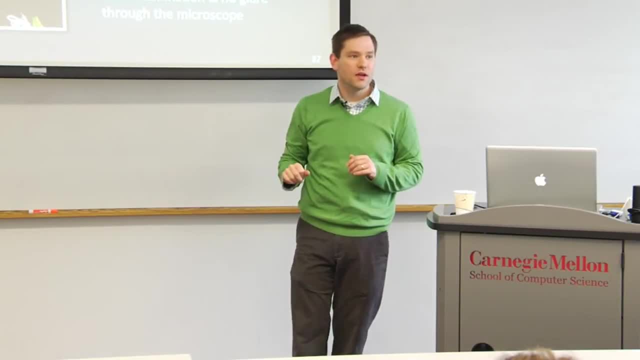 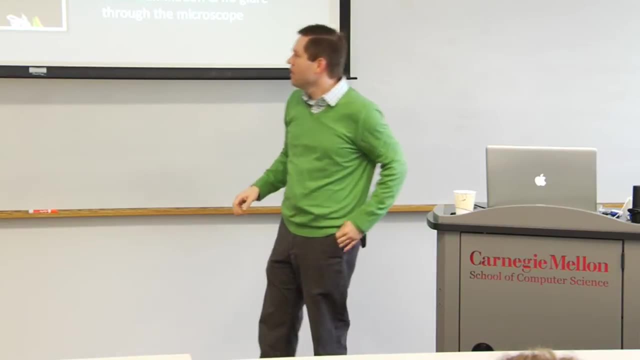 Magnification doesn't even scale depth the same way that it scales the transverse image, But at least you can pick up subtle changes and these changes are going to apply equally to your tools and to the image. Now this has direct clinical relevance to our image overlays. 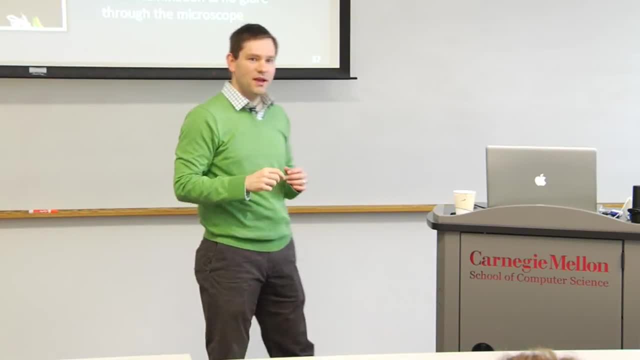 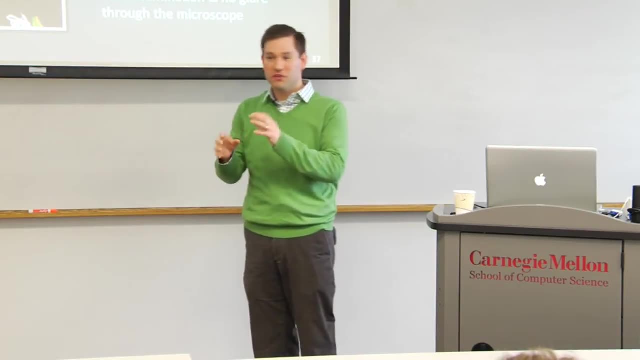 because when we're putting a tiny patch of OCT image in the surgical field, that patch is going to be a tiny square with some OCT data inside it. It's hard to tell exactly how a tiny patch is tilted and oriented if you don't have more information around it. 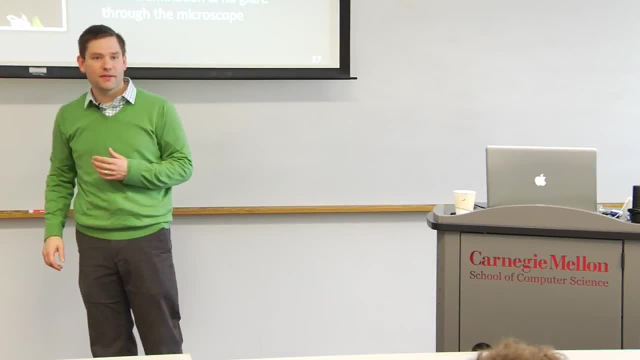 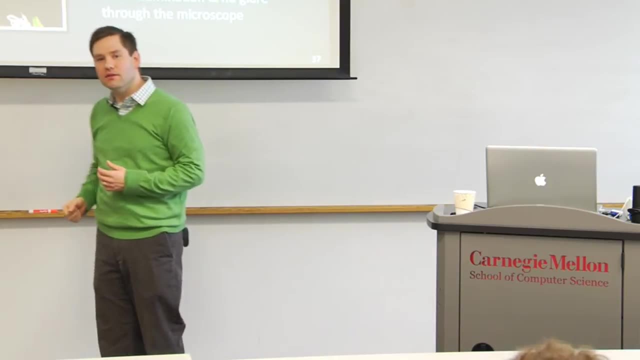 We had originally thought we could get around this by making a grid that you can turn off and on. that gives you this large image in the same plane as the OCT image and have a nice grid in it. so you get all these rich features, Turns out. that's bad. 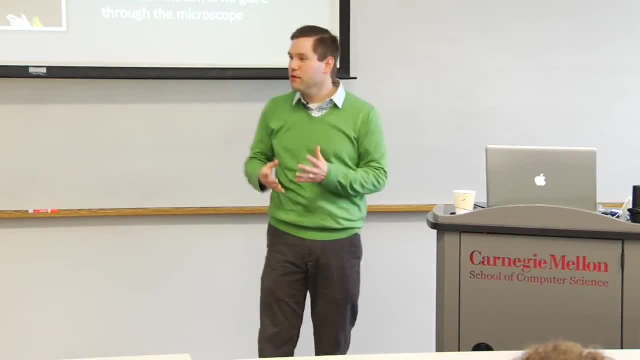 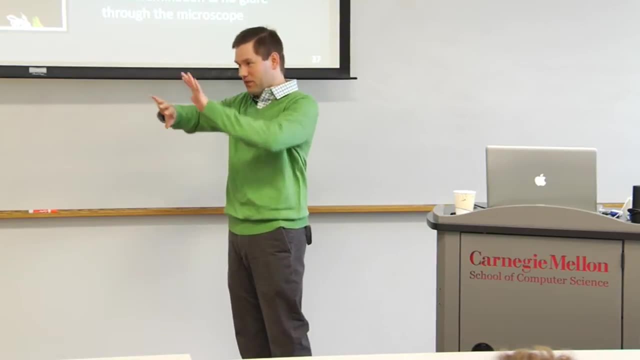 It actually confuses you. The fact that the grid doesn't scale as the way it's supposed to messes you up when you misperceive the orientation. If we want to add any features to help perceive things, you know if this is the plane that lies. 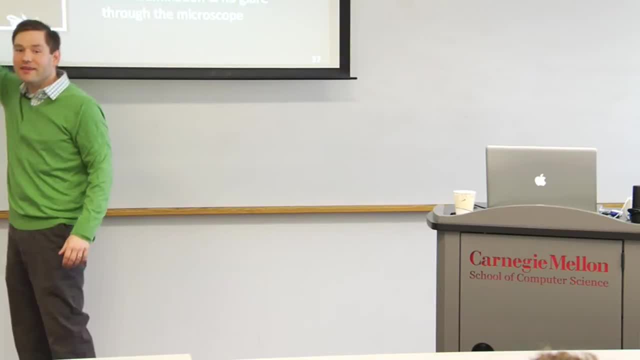 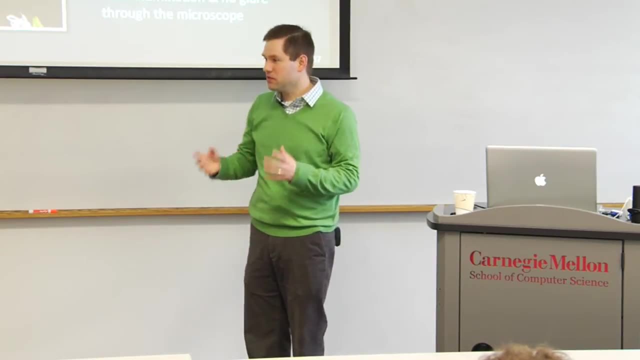 and we're putting some padding the image with other stuff. we want content like this And furthermore, in the OCT images themselves, if we tweak the image contrast to highlight speckle, not highlight speckle, and so on, we need to be careful. 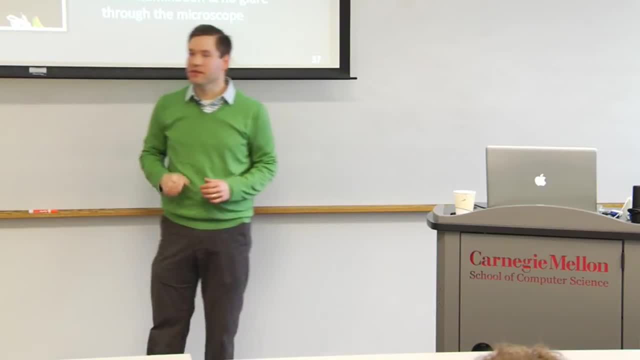 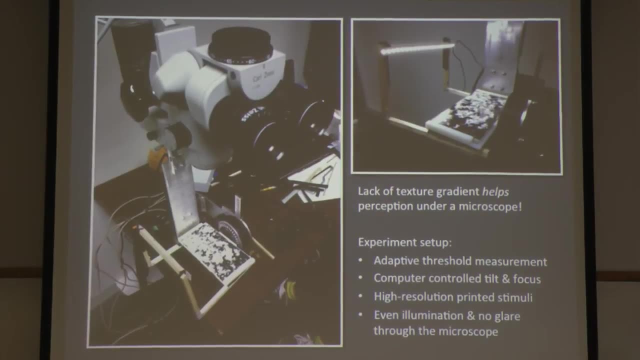 that we aren't accidentally introducing texture gradients that are going to be misleading, And so nobody's ever studied this under a microscope before. Nobody has analyzed how people perceive these things, and we're the first to ever be doing this. I'm studying human perception. 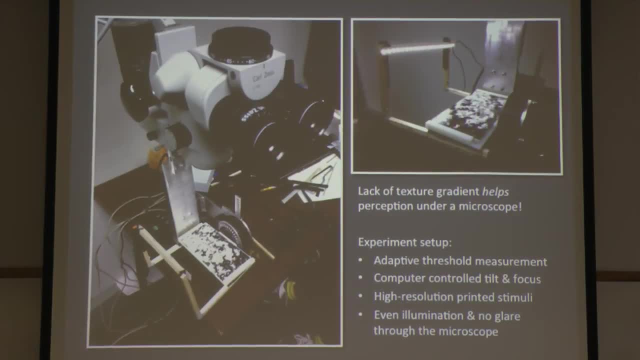 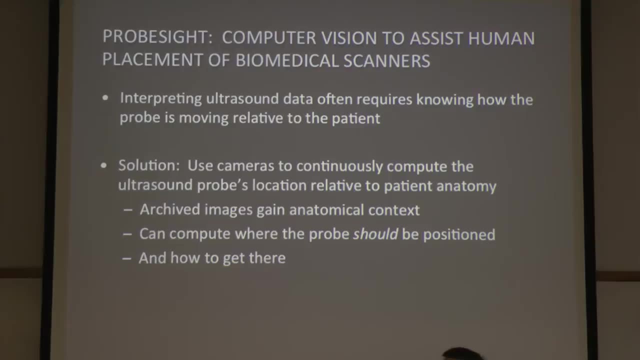 I'm studying human perception under magnification and how the different depth cues interrelate to one another. Now I'd like to move on to talk about the next system. This is the system for which we're getting our funding now going into contracting shortly. 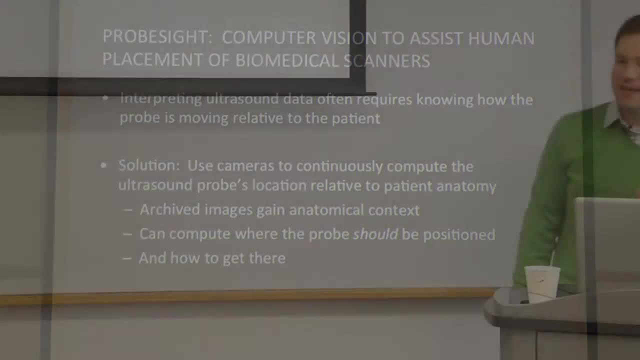 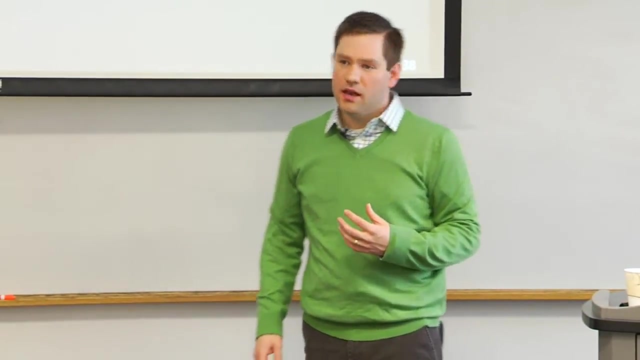 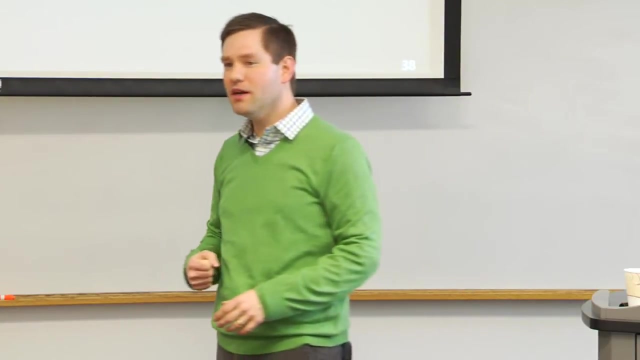 And this is a system to give anatomical context to ultrasound data. Interpreting ultrasound data typically requires knowing where the probe is at all times. An ultrasound tech who's imaging you is looking at the computer screen and taking this probe and pushing it on you, twisting it, moving it around. 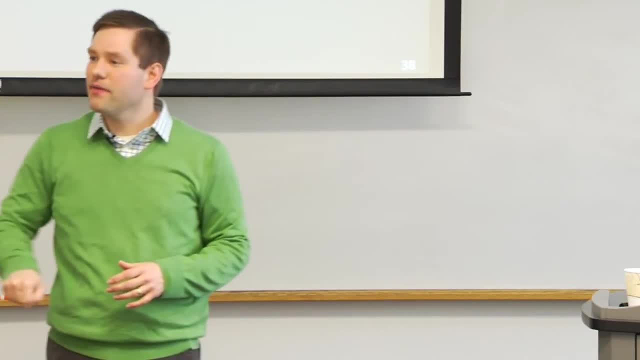 And they know what's going on because they can look at you see where the probe is, and they know exactly how they just move that probe to get from this image to that image. On the other hand, if you've ever watched an ultrasound video, 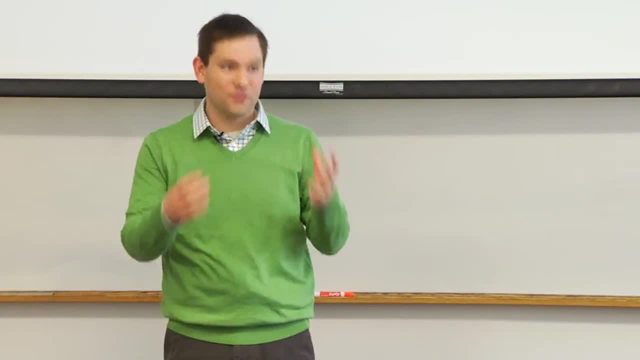 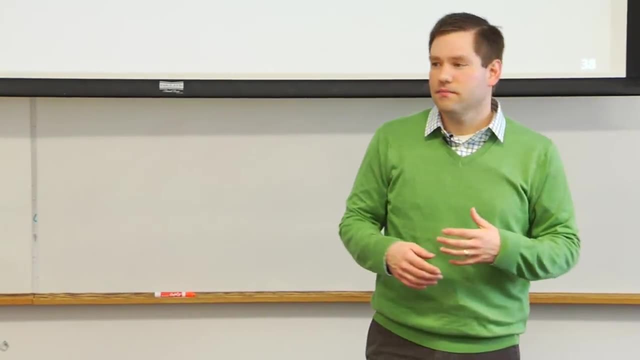 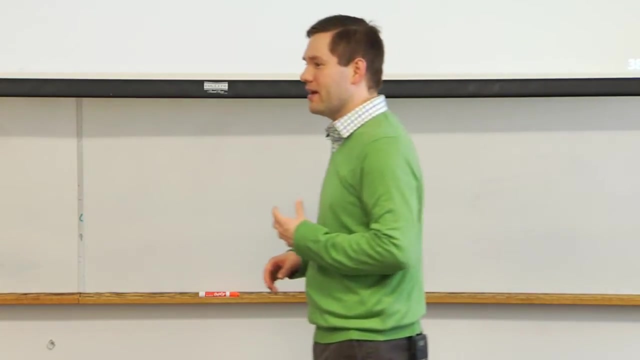 and by ultrasound video I don't mean fetal ultrasound, where it's an easy image of a baby floating in space. I mean something like liver biopsy or liver imaging, thyroid imaging, normal clinical medical ultrasound. outside of the pretty pictures of a baby. It's really hard to know what you're looking at. 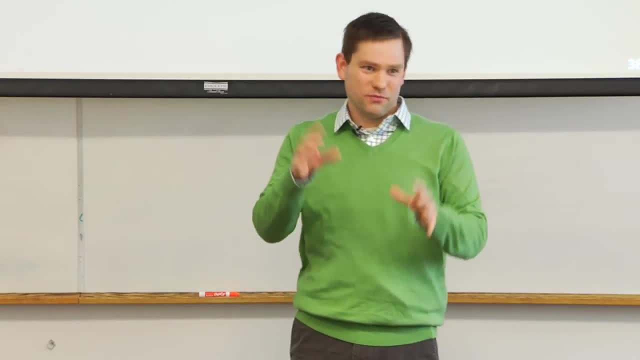 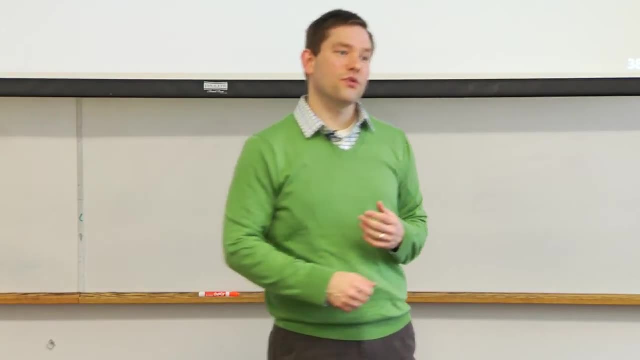 You see these blobby noisy images with some tubes through them and you see new blobby noisy images with some tubes through them And you don't know, did the probe move this way? Did the probe move that way? It's incredibly disorienting. 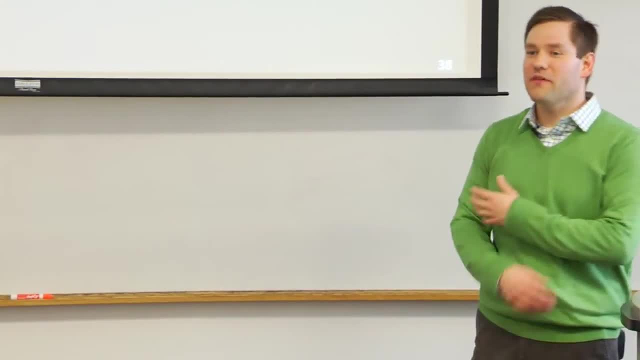 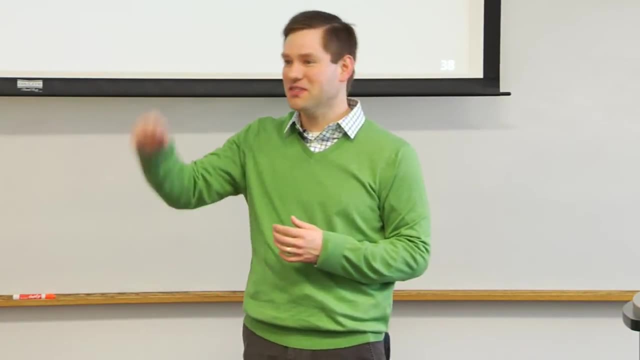 And for that reason, the current clinical practice is to basically discard the entire ultrasound video And all you keep are a few slices that the expert technician, when they're taking the image, said. this slice corresponds to this. believe me, I told you so. 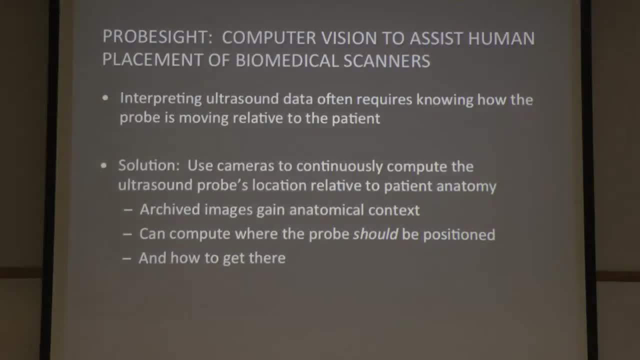 And that's all we record, because it's impossible to make heads or tails of the rest of it. This obviously leads to shortcomings in terms of how we can go back and do post-processing, post or follow-up analysis- legal ramifications, if you want to analyze what happened- and it makes it a lot harder. 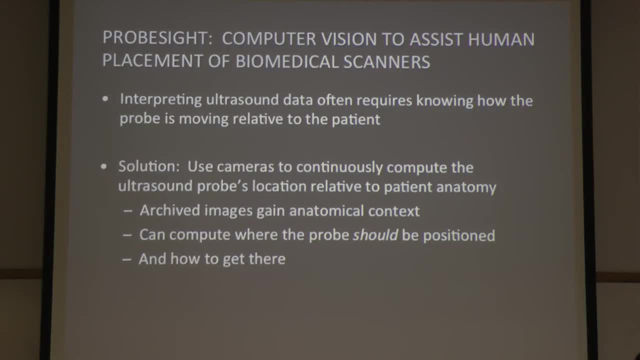 to do longitudinal studies because we can't really get the same image twice. Our approach is to use cameras to continuously monitor where the probe is relative to the patient's own scan and anatomical coordinates. so that we can record where the probe was, We could play back videos that show the image. 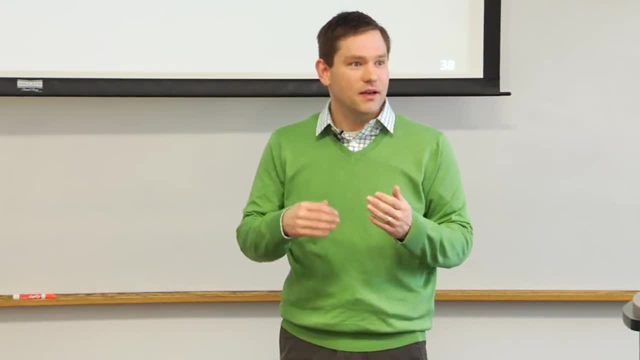 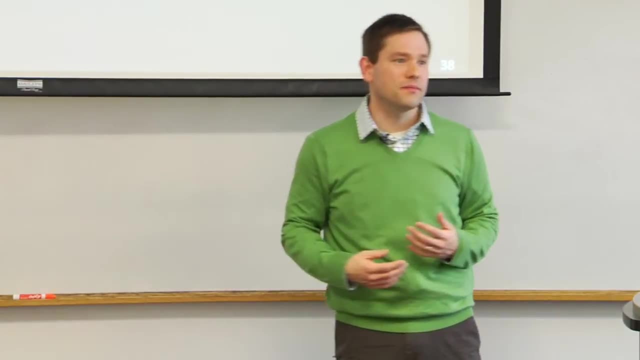 as a 3-D rendering, floating inside a 3-D rendering of the scan, so that now you would see the ultrasound slices exactly in the locations as they moved through the patient. And suddenly, hey, I know where these images were taken from. I can understand them. 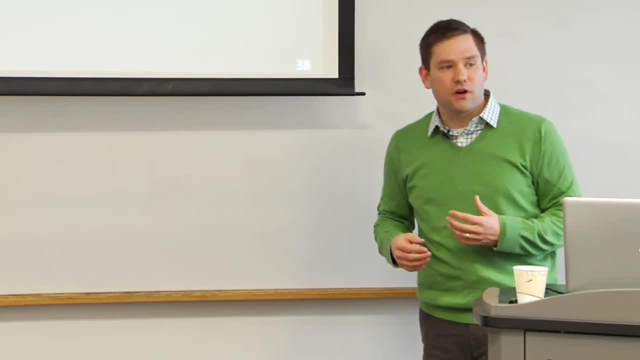 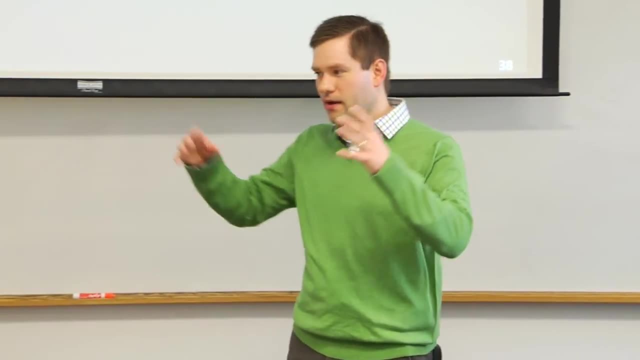 Perhaps even more importantly, though, the computer can understand where the images are. We can do 3-D volumetric reconstruction, And, unlike other systems people have built that rely on cumbersome external optical tracking, we can actually tell when the skin was indented. 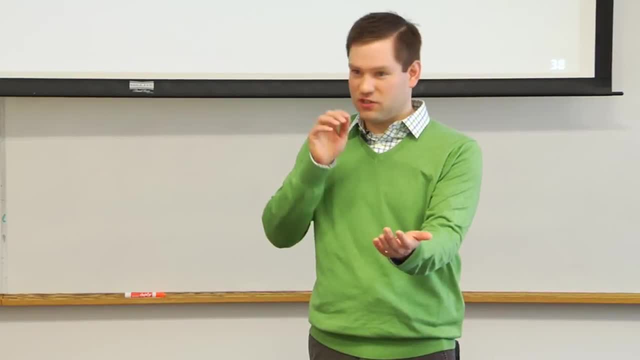 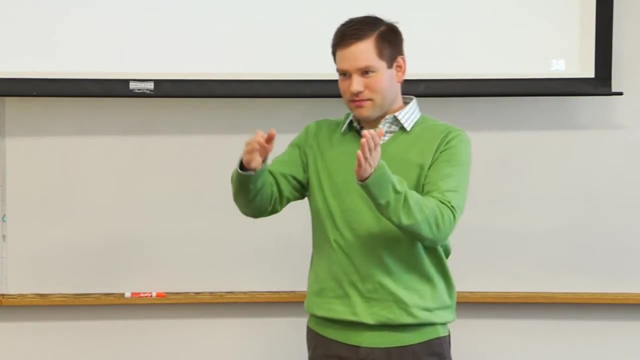 The cameras can see that, hey, the skin right around the probe is suddenly indented half an amp, one centimeter relative to the surrounding tissue. So now, this image that I'm acquiring does not exist. It exists at this place in the world. but, more importantly, 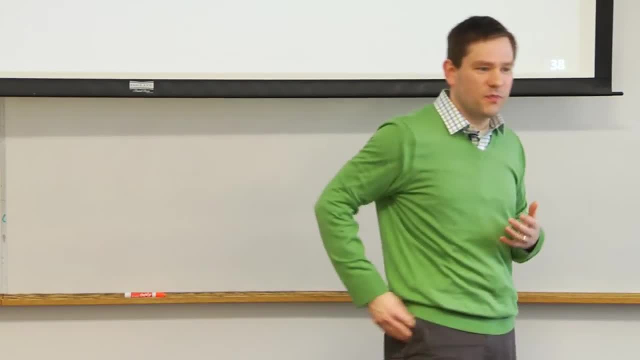 it exists at this point relative to the patient's skin, And this is part of why there's been lots and lots of papers published over the past decade about tracking ultrasound to do 3-D volumetric reconstruction, And virtually none of them have seen any kind. 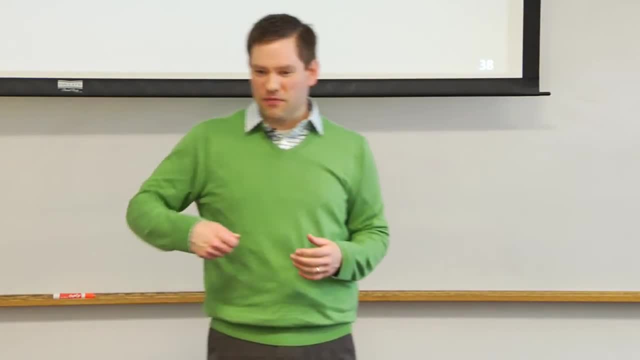 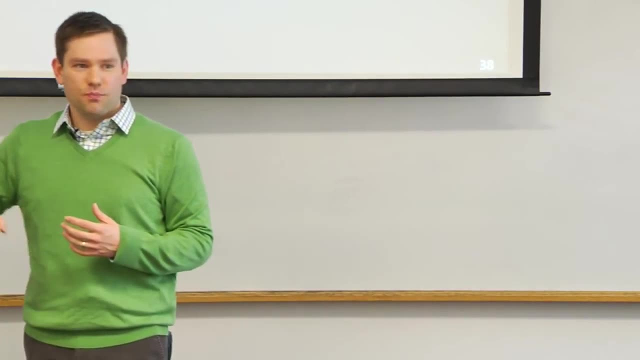 of real, meaningful clinical practice. Because, while you can do a great job if you just barely touch the probe of the skin with gel and move it around, real ultrasound requires that you use the probe as an active manipulator to push and twist and get the probe in just the right position. 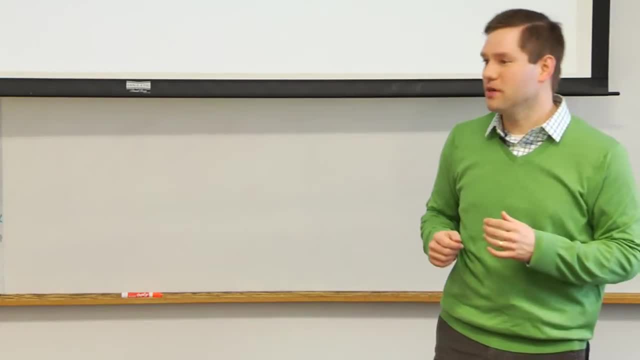 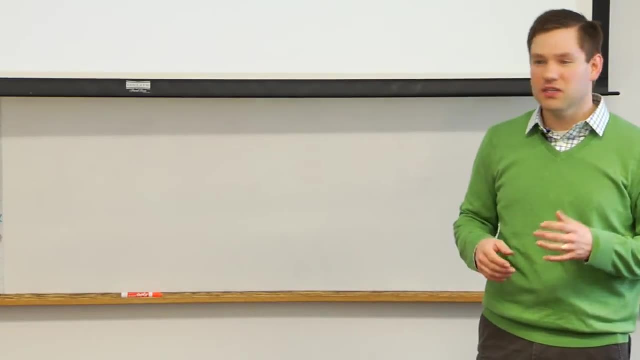 get things out of the way to actually see what you need to see. It's very hard to get a good ultrasound image And to get good ultrasound images we suddenly can't be doing this nice surface-only thing. We're continually deforming the patient and we need to take 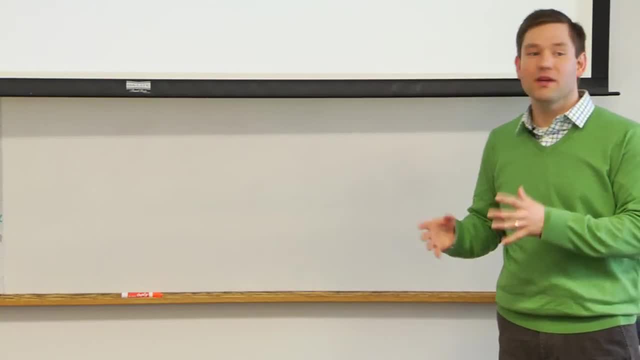 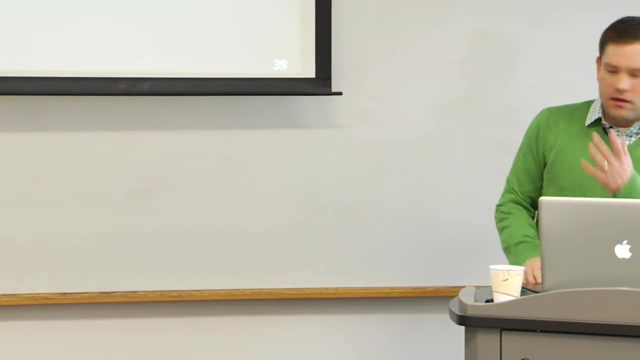 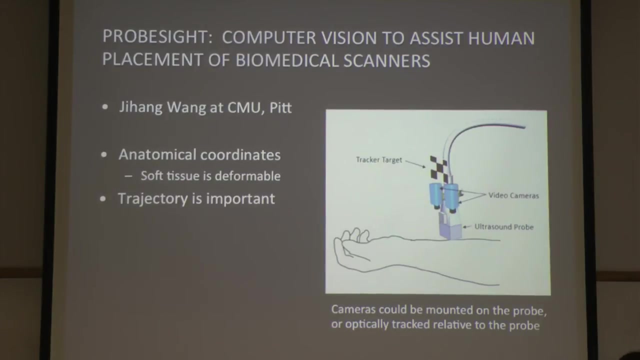 that into account if we have any hope of producing a quality 3-D reconstruction of the data using quality ultrasound images. So our approach is to mount probes or cameras directly on the ultrasound probe to give it this visualization, so it can see where the probe is relative to the patient's skin. 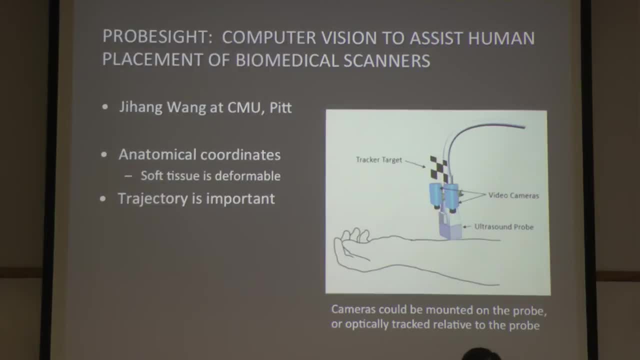 And this work is being carried out by former CMU BME student, Ji-Hung Wong, who's now a PhD student at the University of Pittsburgh, And in doing this, we're able to track the probe and the trajectory of the probe to know how the skin was deformed. 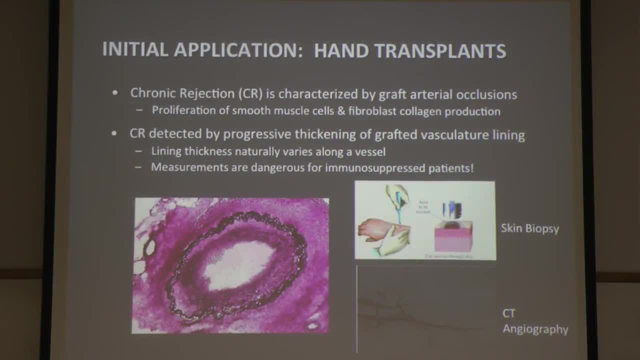 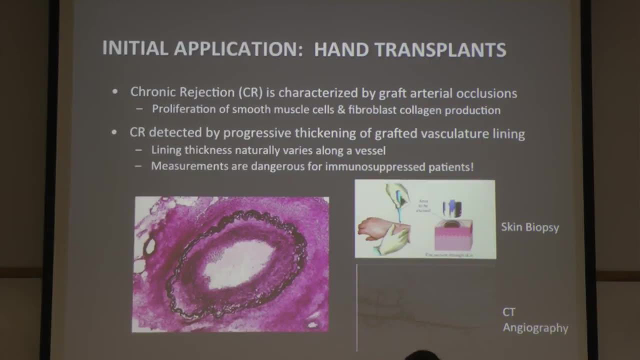 how we got there and so on. Our initial main application of this, for which we're getting funding, is to study chronic rejection and nerve regeneration for hand transplant patients. DoD is interested in hand transplants, as you can imagine Now, with any kind of transplant. chronic rejection is a major problem And there's lots of ways we can try to monitor for it. The problem is all of the methods that would let you know in time to do something about it are not safe for patients that have compromised immune systems. 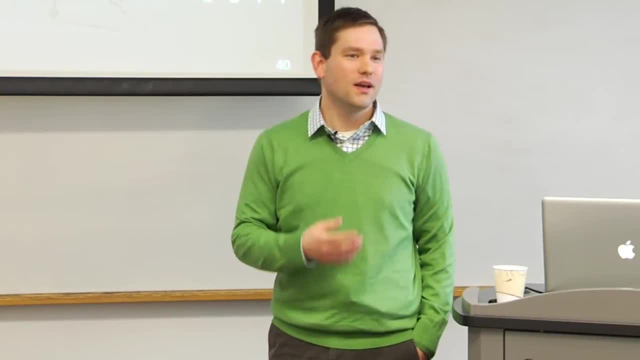 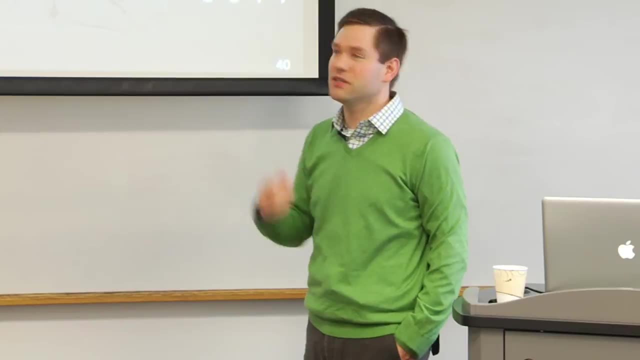 And patients who've received transplants have immunosuppression going on, so their immune systems are compromised. We can do CT angiography, but we're dumping radiation into them. sticking needles into them could introduce bacteria. We can do biopsies, which is even more likely to introduce bacteria. 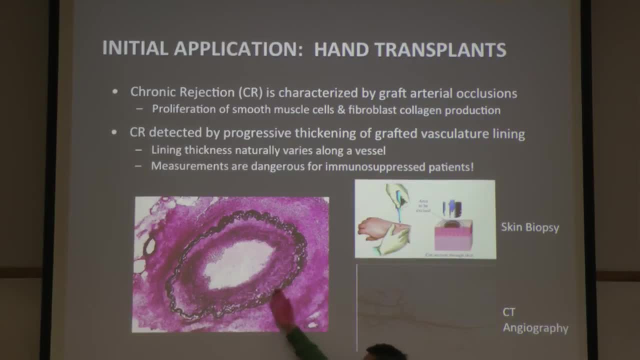 and do nasty things. But if we did a biopsy and looked at the medium vessels and took that and looked at that under a microscope, with staining we can see various structures here that would indicate intimal wall thickening of the vessels, which is the first sign that chronic rejection is happening. 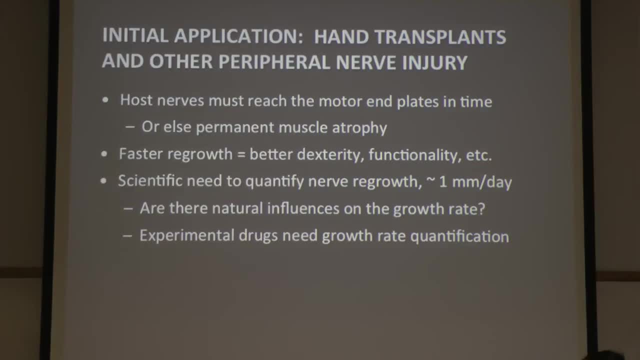 Also for these hand transplants. it's very important for the nerves from the host to re-innervate to the transplanted hand as quickly as possible, Because until they reach the motor end plates, the muscles are continually atrophying. 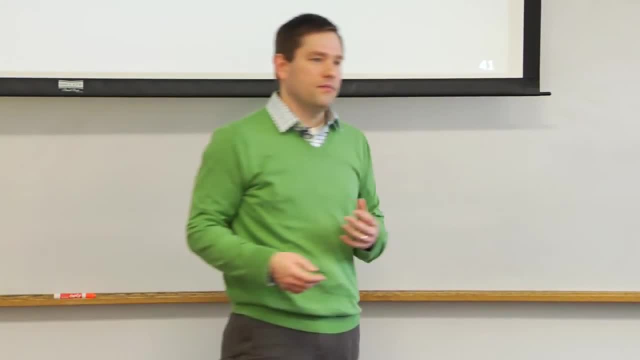 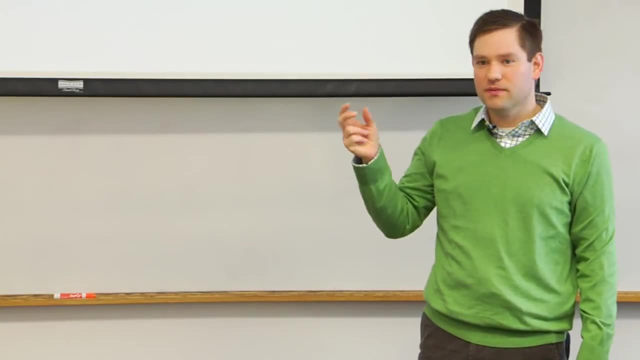 And if they don't get there in time, you'll have permanent loss. If you transplant just a small portion of the hand and life is good, then the patient eventually regains full, dexterous motor control that they can pick up a bottle with one hand. 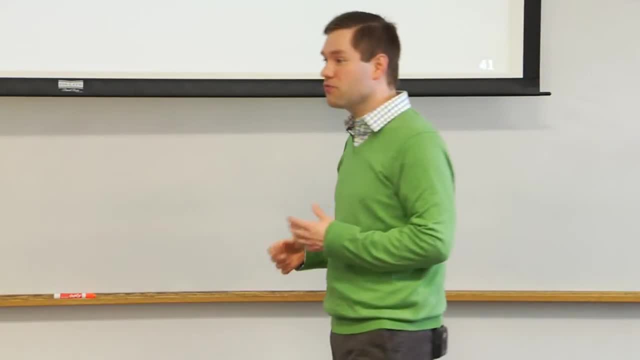 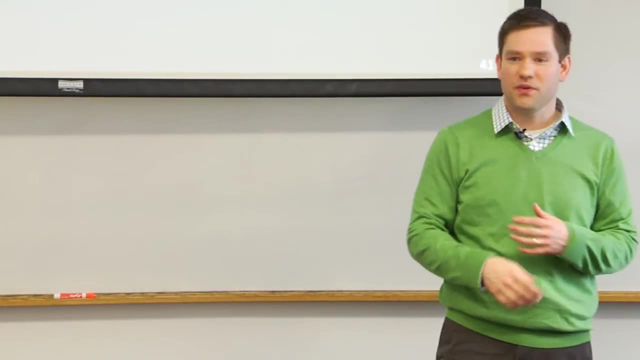 twist the cap off with the same hand and basically have full human control. That's one of the most complicated things you can do, as I understand it, in terms of fine motor control in a hand. It's something that monkeys can't do. 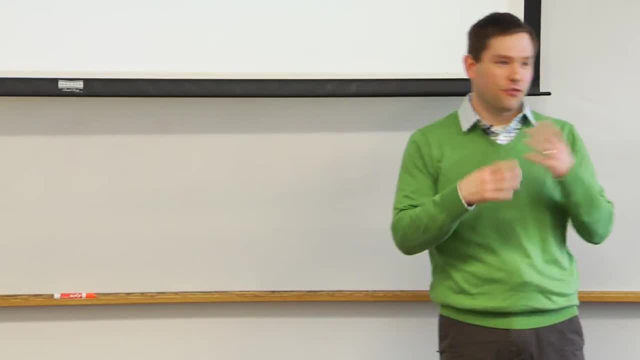 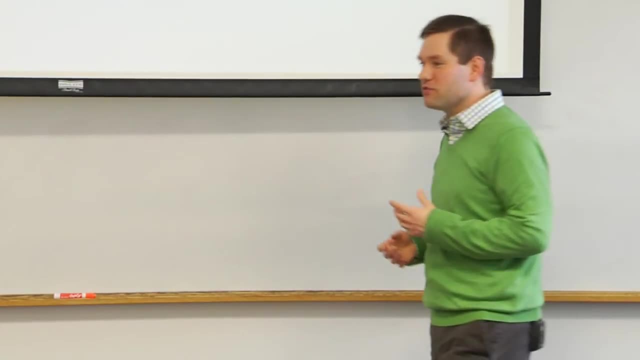 It's unique to people And they regain this full level of functionality. They regain full sense of touch perception and so on. It's basically a fully functional transplant. But because nobody can really monitor how these nerves are regenerating, it's really hard to do clinical studies in terms. 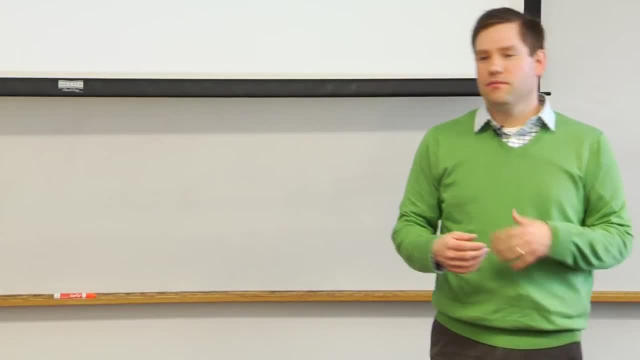 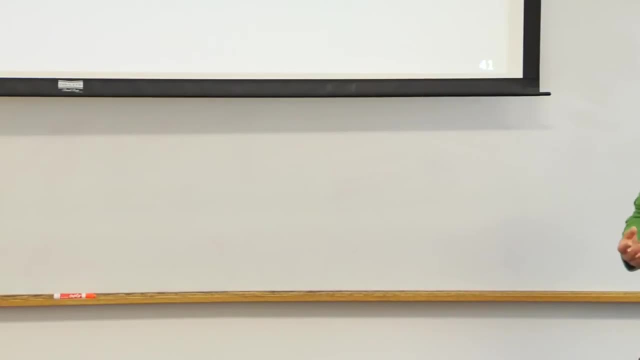 of which drugs can we give them to make the nerves regenerate faster? How can we change our surgical procedure to make this more likely? If we have to put a graft in place, what's the best way to do that? The science is an open-ended question that's starving for real-time feedback. 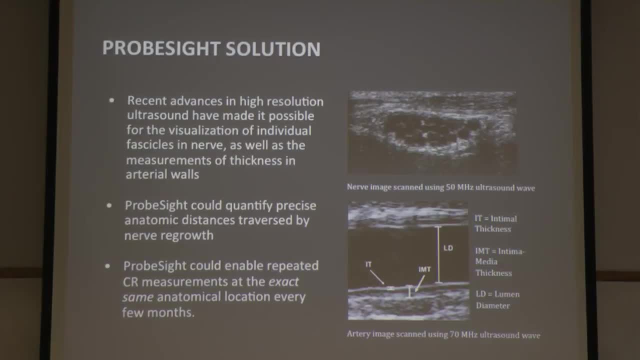 in how these nerves are regenerating. There have been recent advances in ultra-high-frequency ultrasound that can actually see the individual fascicles of a nerve bundle here. This is brand new. There are only four machines in the world that you can use to do this. 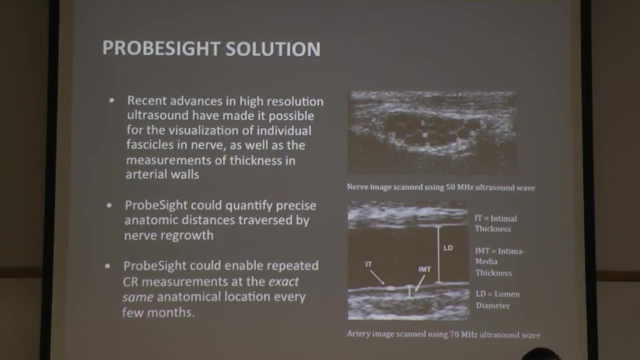 And this is again, only under IRB approval. They're experimental systems And we have access to it. We have access to one of them And our hope is that, by looking at subtle changes in edema swelling, so on and so forth- 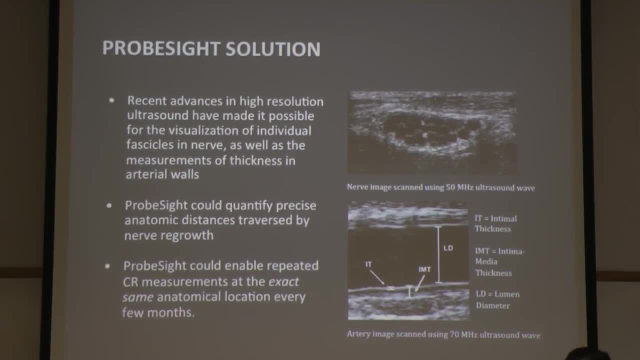 compressibility of these fascicles, that we can actually infer where the nerve fibers are and where they aren't along the length of that. This is going to be a giant study we're going to be doing. And likewise, this same scanner can image blood vessels inside the arm with such fine detail. 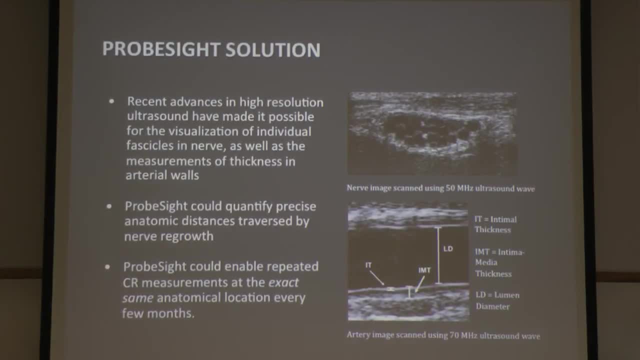 that it can see the intimal wall right here And we can measure the thickness of this. Now, as you can see, the actual thickness varies naturally along this, And this is problematic because, while we could take the scanner, this brand new system- 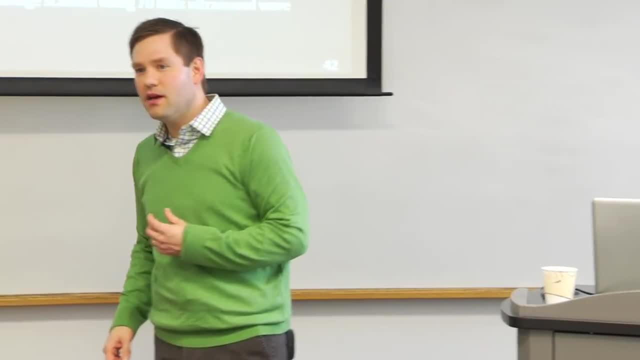 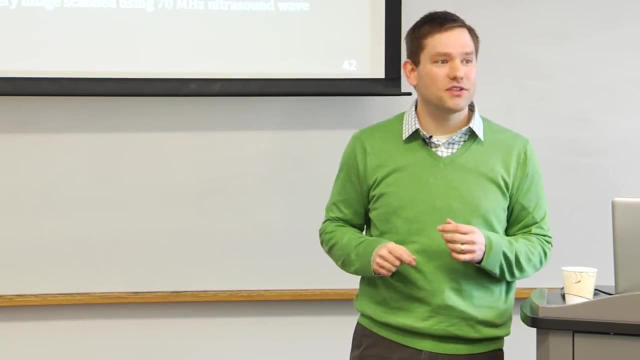 and we could put it on you and get a measurement of intimal wall thickness. if we come back three months from now and get a new measurement, even a subtle shift in the angle of the probe will have us imaging a sufficiently different patch that we can't say whether any differences we measure are because well, 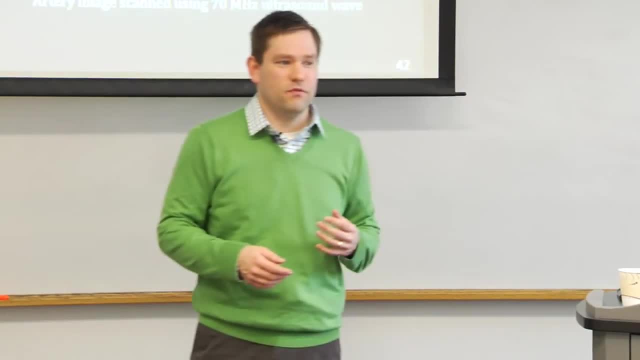 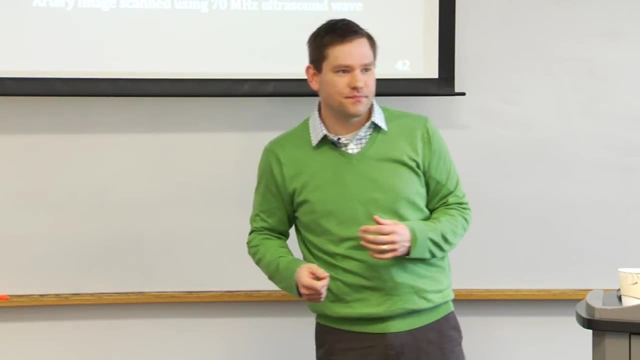 we just imaged a different place in the vessel and it was bigger. but so what? Maybe it was already bigger there, Or is this actually a meaningful change that's happened over time? Using our approach with the cameras, we will be able to tell where the probe is located. 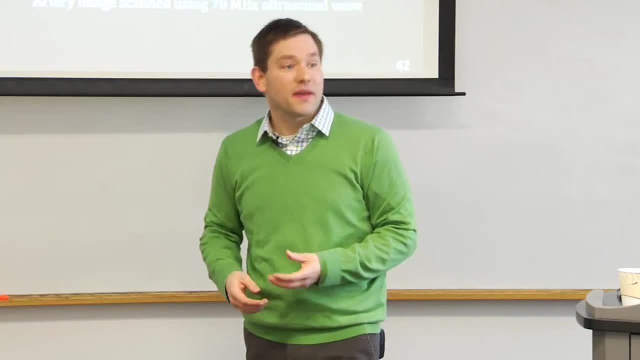 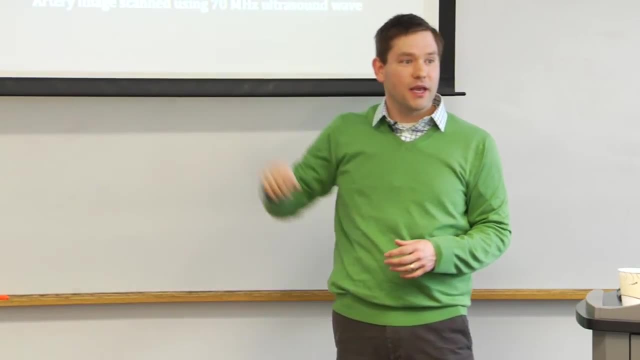 how the probe is tilted, how indented the skin was when that image was taken, and precisely get back to the same configuration so that we can actually tell meaningfully, you know, the changes that we're seeing, do those correspond to something real? 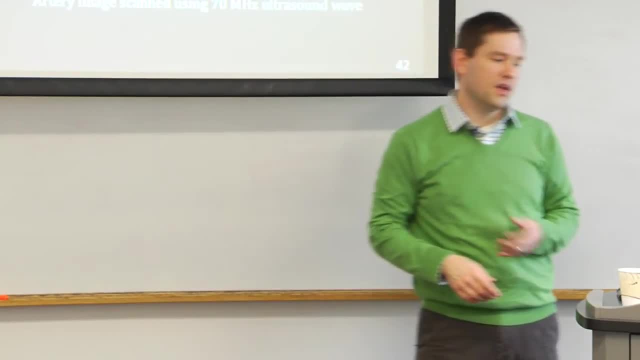 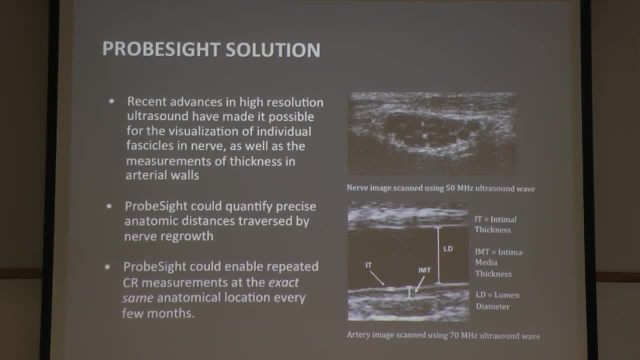 And this would enable us to measure the length of the vessel. And this would enable us to measure the length of the vessel, We could enable, for the first time, safe diagnostic measurements of chronic rejection. And we could use the system likewise for many procedures where we want 3D information on patients. 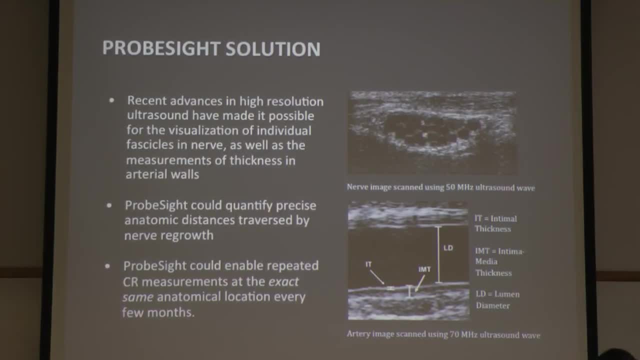 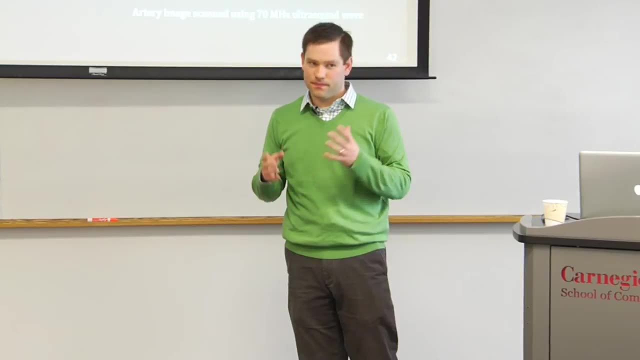 that we can't do otherwise for other things that are visible, for example in an MRI scanner. These patients have metal shrapnel embedded in them. We can't do MRI CT again has radiation and these patients often have you know. 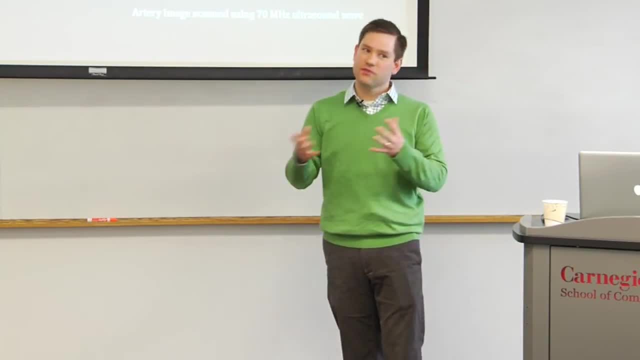 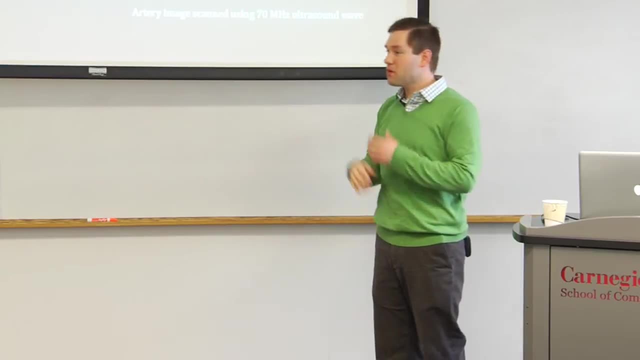 systems that have a trouble regenerating other clinical problems. can't do MRI, don't want to do CT, And if we could enable 3D imaging with high-resolution ultrasound like this, this would be groundbreakingly huge for the treatment of these patients. 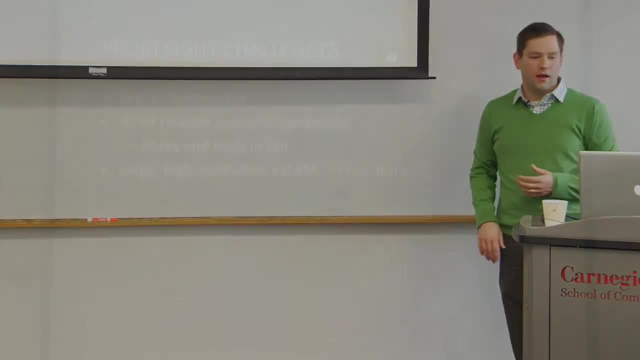 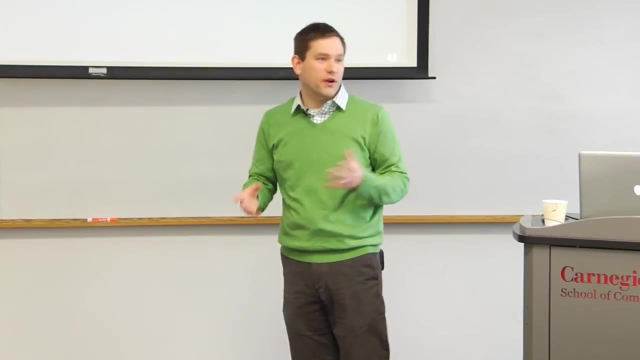 Challenges with probesite. the skin is deformable. We need reliable anatomical landmarks And, if we're working on patients that don't have lots of freckles, hairs and other things, basically all we can rely on is skin pores and the folds in the skin. 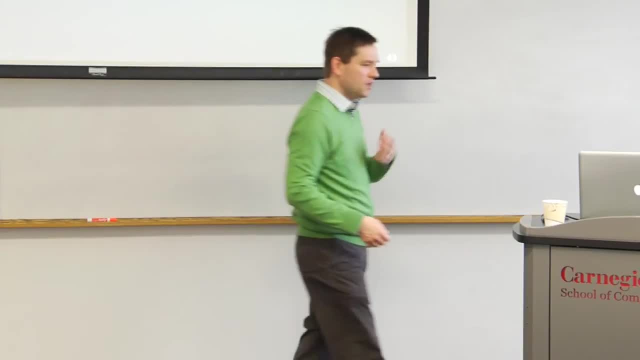 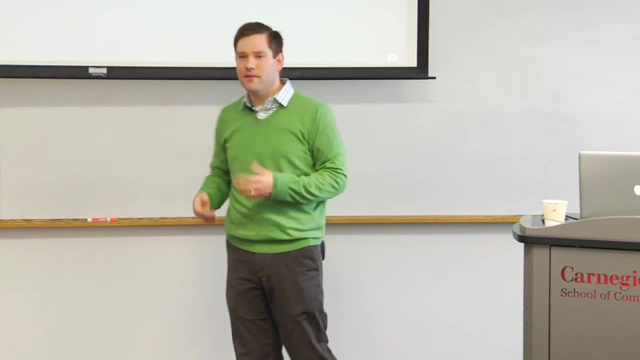 Think fingerprint, but on your arm. To be able to see those structures, we need large, high-resolution images. In essence, what we're wanting to do is visual slam- 10-megapixel resolution, if you will, in real time. 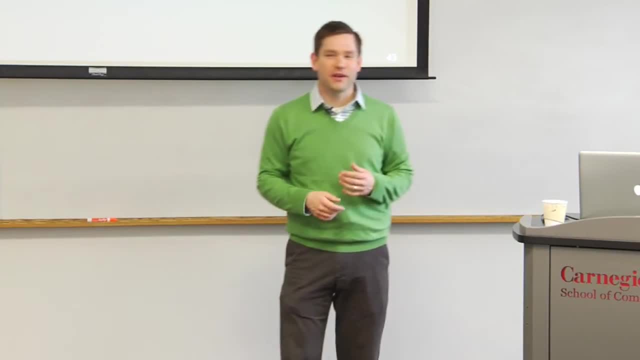 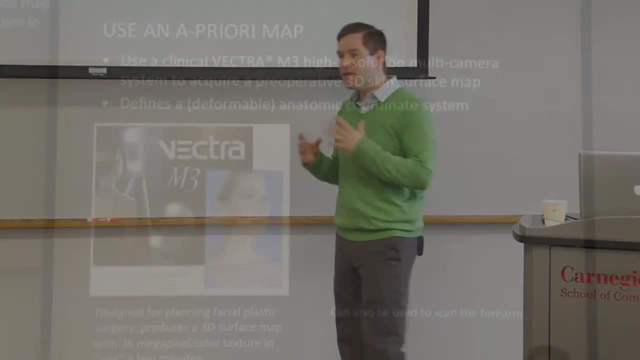 And hopefully you're chuckling inside at this point, because we can't really do that. You're lucky if you're doing visual slam at VGA resolution. Our approach to get around this is to use a high-resolution operatory map. We have access to a special system. 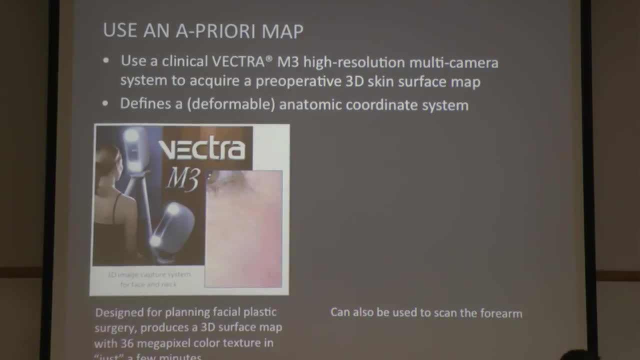 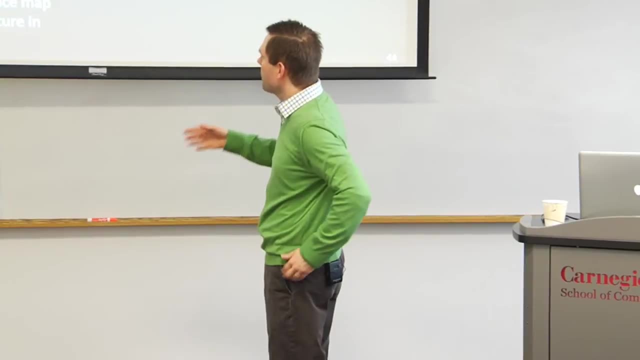 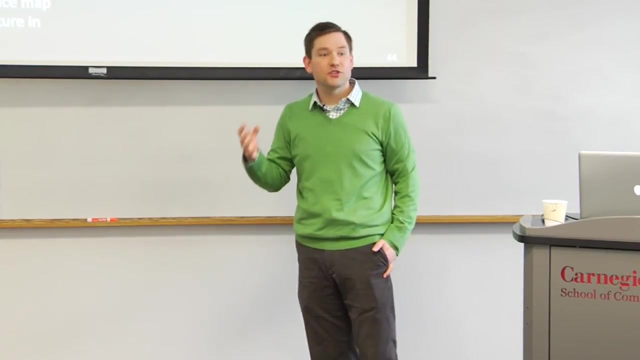 in the lab. We have a system in plastic surgery at UPMC that was designed for pre-planning on plastic surgery, for face procedures and so on, And this system is able to produce 36-megapixel high-detail 3D color images. 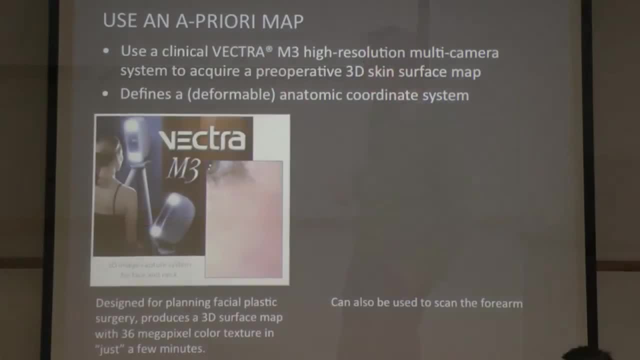 with full shape and visual appearance of a face with sufficient detail that, as you can see, hopefully you can see there. you can see the individual crease lines in the cheek. there They're all visible. The system basically uses three pairs of SLR cameras. 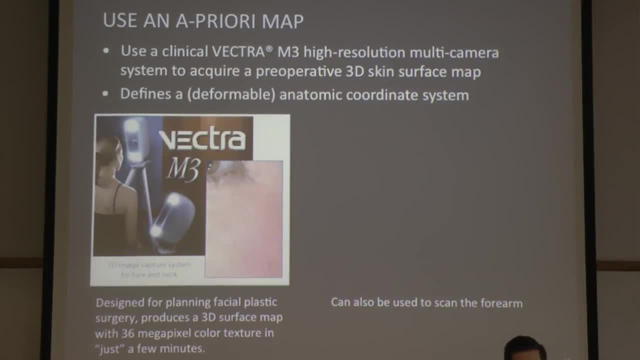 and stereopsis between all three of them and then between the pairs, additionally from different viewpoints, to be able to run some advanced proprietary software that takes several minutes to take this instantaneously acquired image and compute to produce the point cloud overlay it, produce this image. 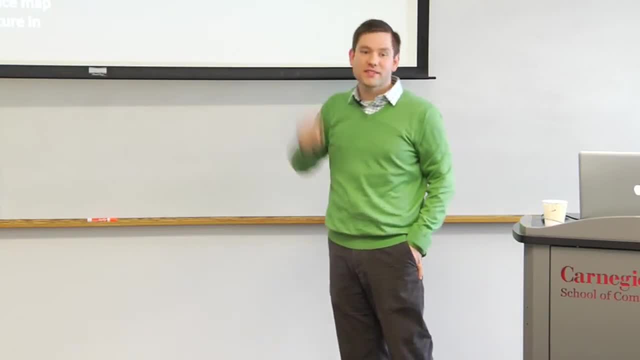 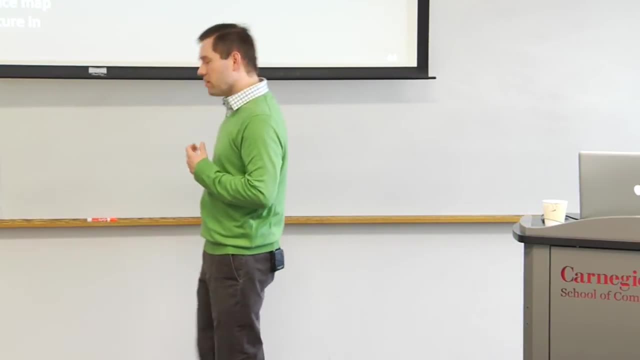 You couldn't at all use this in real time, But we can get one fixed image and let it compute and give us this high-resolution 3D surface map. Once we have this, we no longer have to do simultaneous localization and mapping. We have the map. 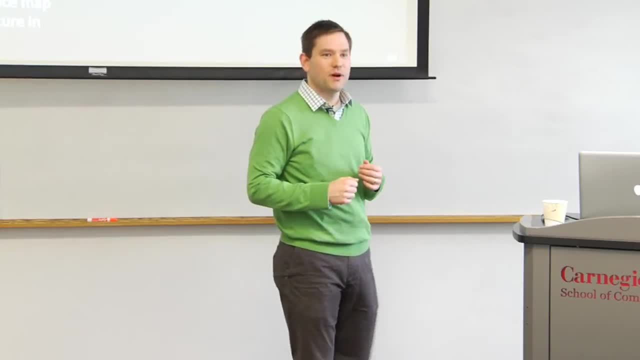 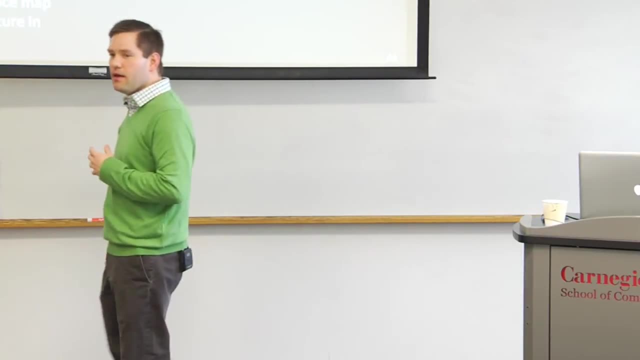 We just need to do simultaneous localization- A much easier problem. Still hard, but substantially easier. Furthermore, having the map gives us, for the first time, a meaningful way to talk about coordinates in a deformable way. As I said earlier, we need to do 3D registration. 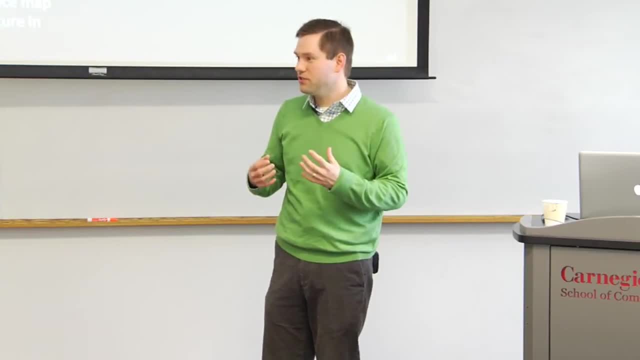 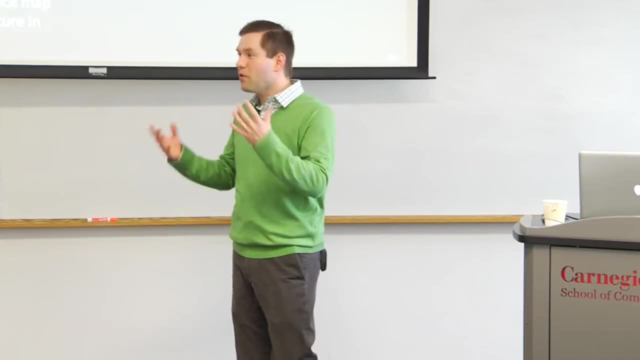 and Cartesian six degrees of freedom aren't sufficient to describe deformation, Although the probe is there. Well, is the probe there relative, you know, to their navel? Where is the probe there? relative to the operating room? Where is it? Now we can say the probe is located at this exact point. 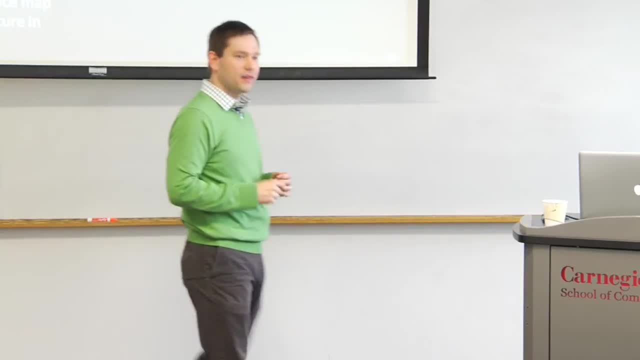 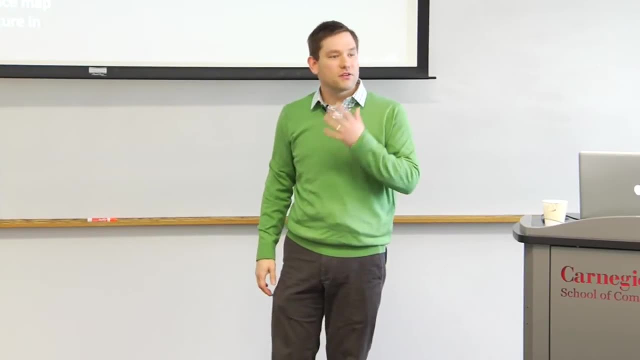 on our pre-acquired surface map with this exact orientation relative to it, And, furthermore, this image was acquired with the surface map deformed thus, And now we can describe fully what it means for that probe location. We have a full 3D deformation tool for the surface map plus. 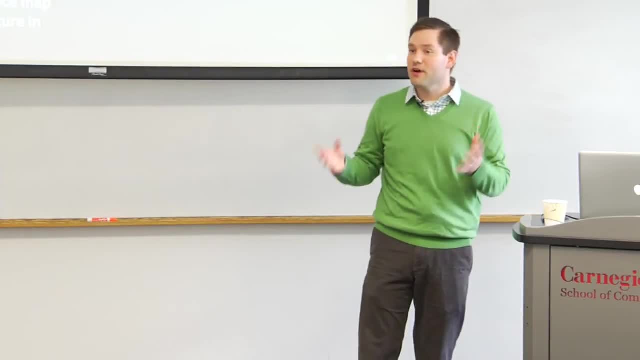 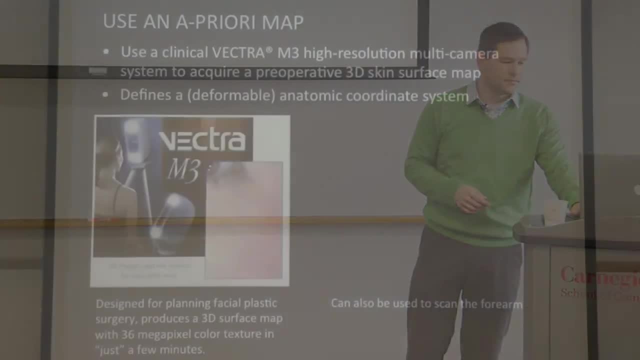 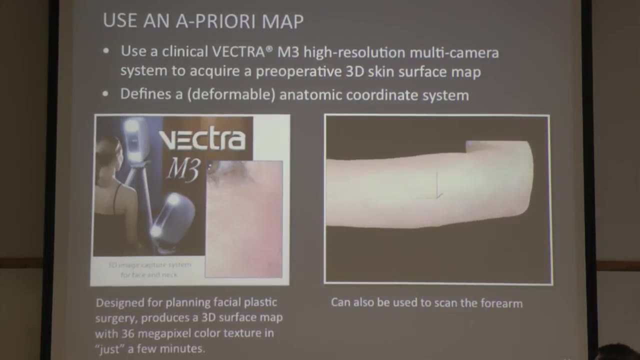 and we can take everything and relate it back to the surface map and we can deform that surface map- And we've used that scanner to also scan a forearm- and we can create the surface model. We can view it from all different directions. 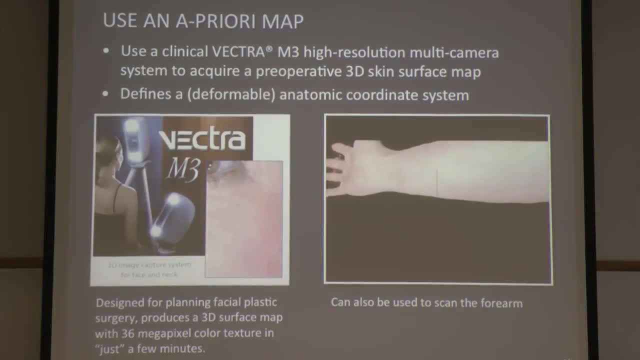 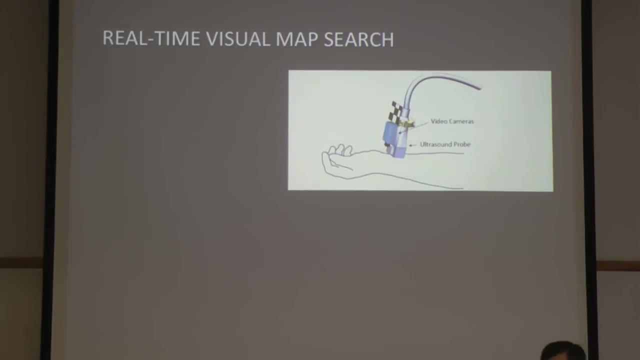 see the details in it and so on. Using this, we still have to do a real-time visual search to map what the image from the camera is currently seeing to where it is on that prior scan. If we know about where it is, and we hope to be able to do- 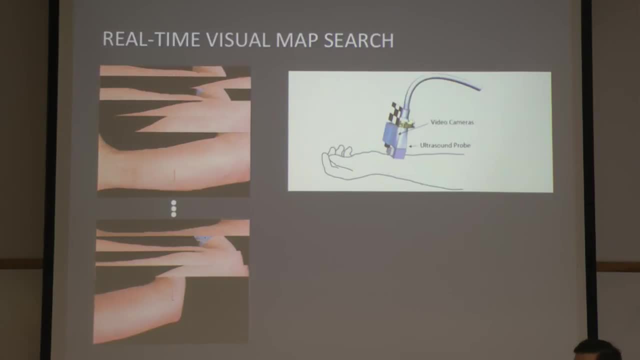 that, for reasons I'll discuss shortly, we can then generate a whole bunch of renderings of that 3D surface model from the possible viewpoints of the camera. Well, the camera was about here relative to the patient, but maybe it was here, maybe here, maybe here. 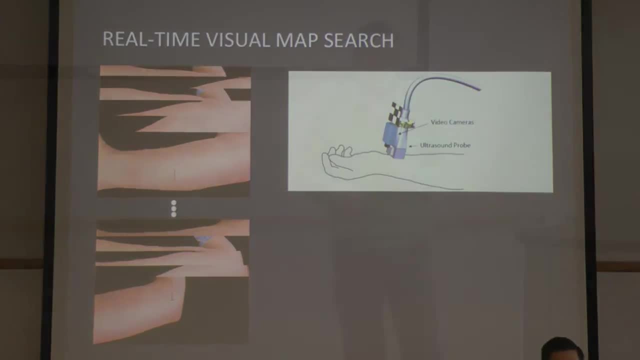 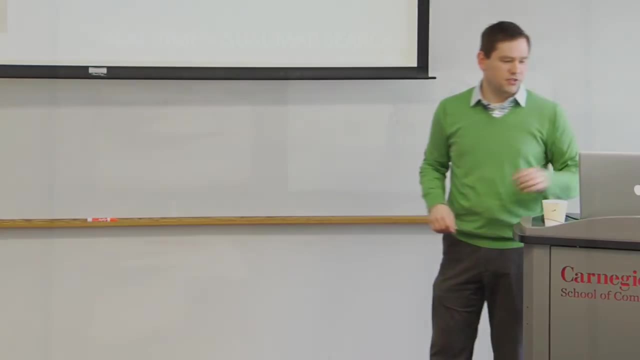 maybe here, so on and so forth- Generate a bank of these images and we basically have a visual search about this search space for which one of these images best matches the actual image we're seeing from the camera right now. Once we know which image best matches, 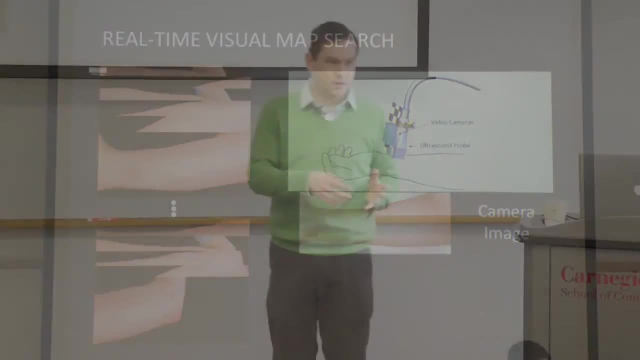 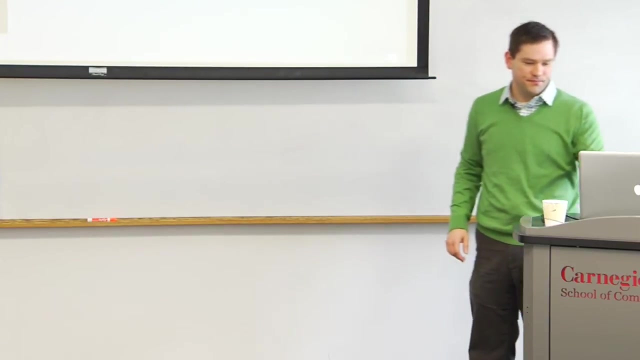 we know what simulated viewpoint was used for the camera to generate that image, and so now we know where the camera actually is relative to that 3D surface map, and we've thus localized it, And so we're looking for the best match out of there. 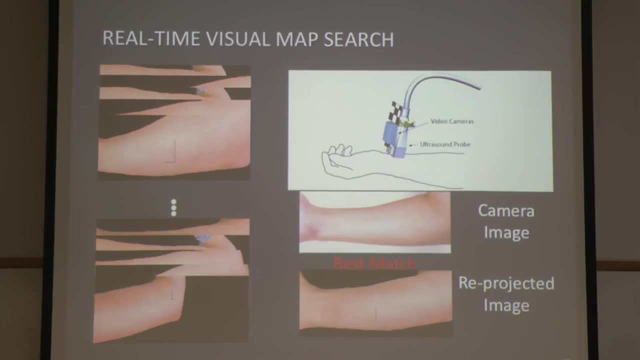 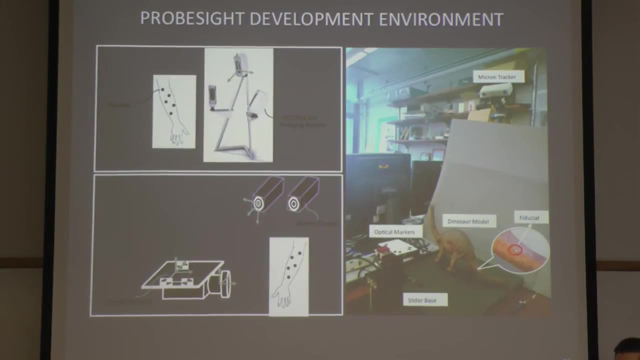 It's a visual match image search that we're trying to do very rapidly across a large number of images in real-time frame rates. Our experimental setup, which is what can be called a 3D model, is pretty much all about the 3D model. 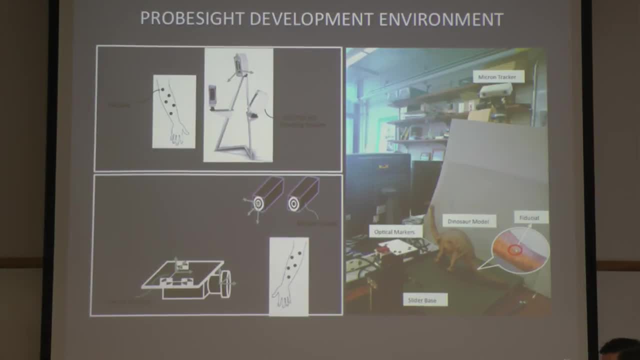 It's also a 3D model that's clearly able to cache and Hammersmith and a lot of other things. Also, we have a camera, so that's really great, And so we're looking at that to see what are the best matchings and what's best with the model. 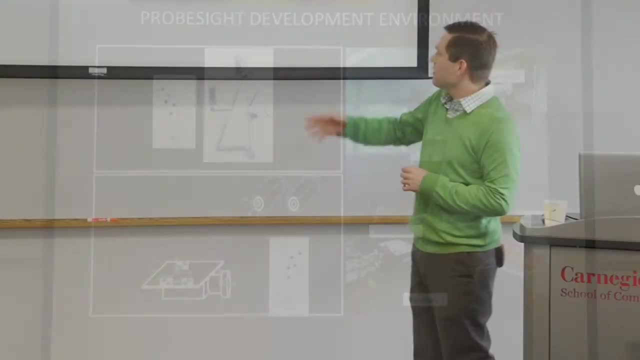 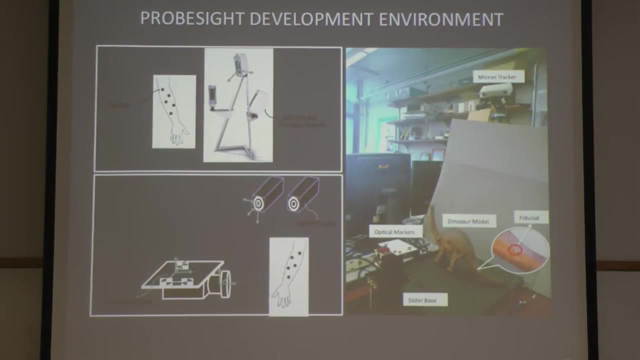 And so we've done some deeper analysis, so now we can see what the model is going to look like. We've got a few things that we haven't really looked at yet, So one of the things that might interest you as we talk about this is: we're looking at, how do we look. 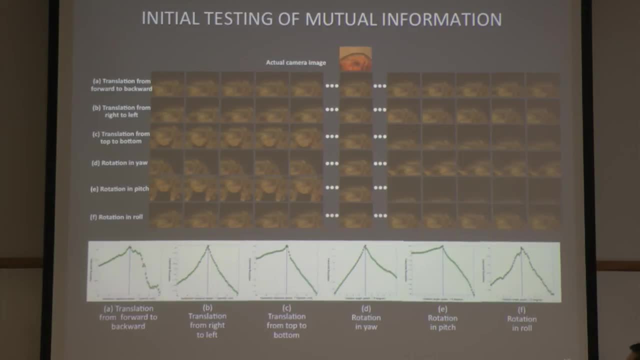 at tracking on a camera, took a bank of images over all these different search spaces and used something simple like mutual information that we do in fact get the best match at the exact correct location, The metrics fall off everywhere else. So if we get the best matching image, 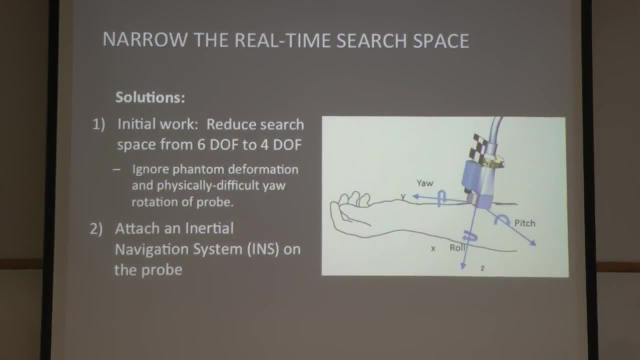 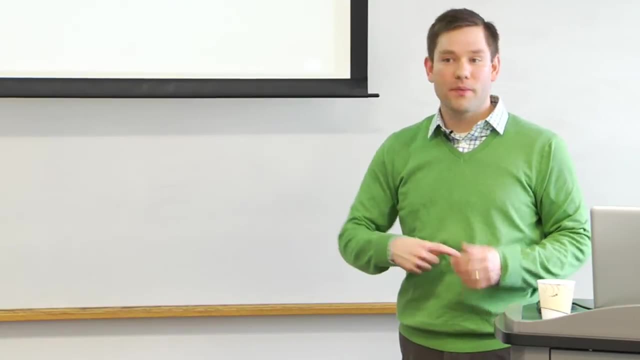 it will be the correct location of the camera, And we're working to address the real-time nature of this, initially by reducing our search space to ignore yaw of the probe, because probes have a rectangular cross-section so it's hard to rotate them in one dimension. 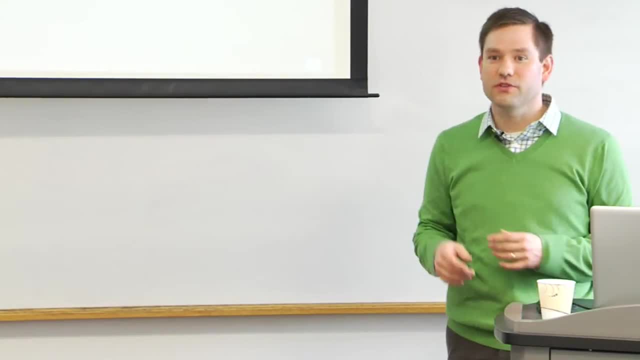 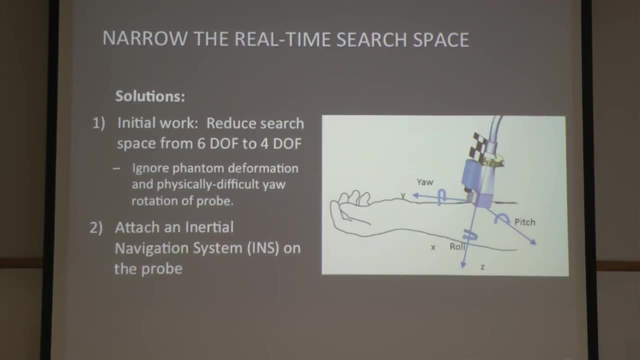 And initially to ignore deformation as well, because as computational resources improve, that will naturally take care of itself. if we can get it working for the others, We can do that at not real-time but real-time. we're ignoring that And, most importantly, we're attaching the inertial 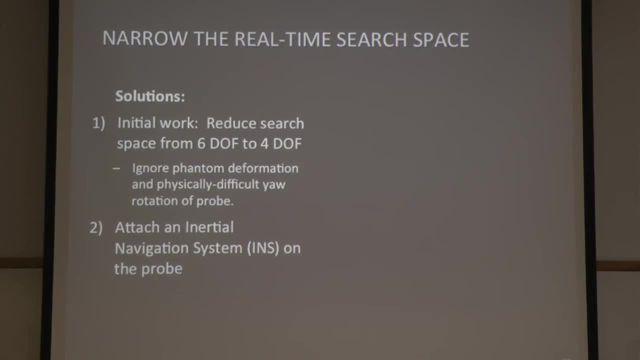 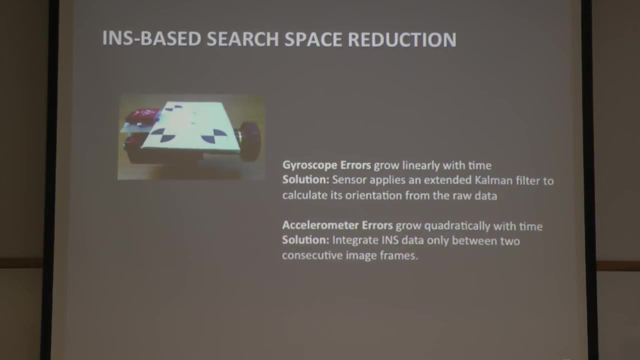 navigation system to the probe as well, And we do this to get an approximate answer for how the camera's moved to have a nice narrow search space. Now the system- as I'm sure you're aware, inertial navigation systems- suffer from drift. 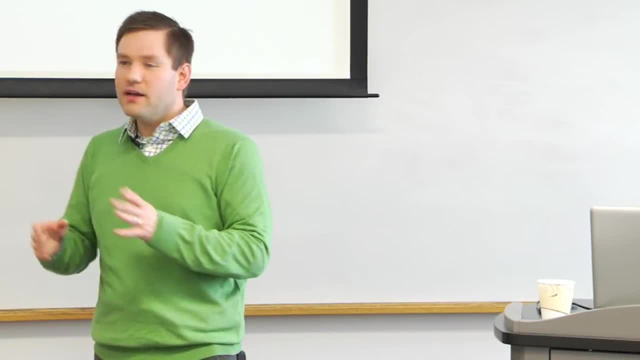 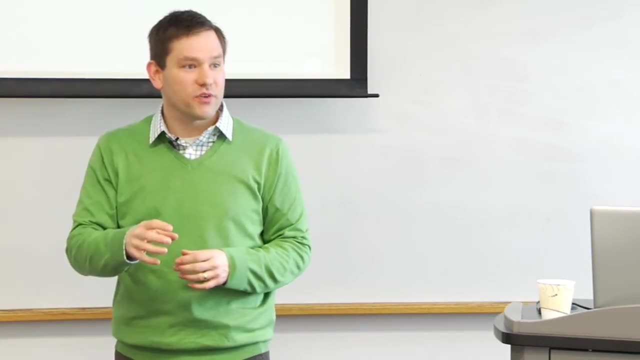 The air accumulates in a nasty way. However, because we only need to use the INS to get an estimate of where the camera is and after that we do a visual search to find out exactly where the camera is, we don't integrate this error over any meaningful period. 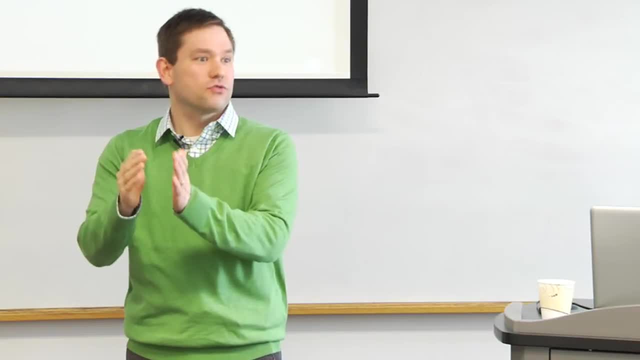 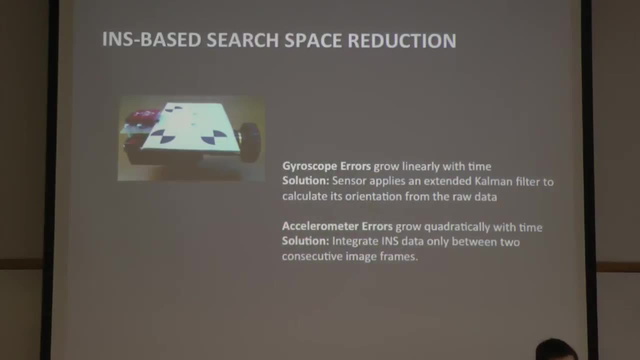 of time. We have a very small amount of drift, but we can still do a tight visual search. We find exactly where we are and reinitialize our INS system to now be doing a visual search from scratch again or integrating from scratch again. 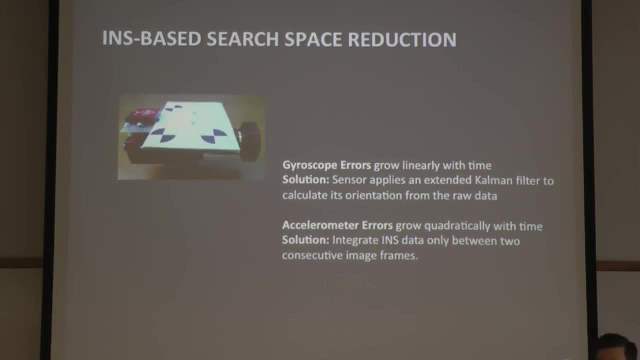 And so we never let the error build up. We're using the best of both worlds: INS for its short-term accuracy And the visual match for its exact accuracy, but over a narrow search space. The INS system we're using was recommended to us. 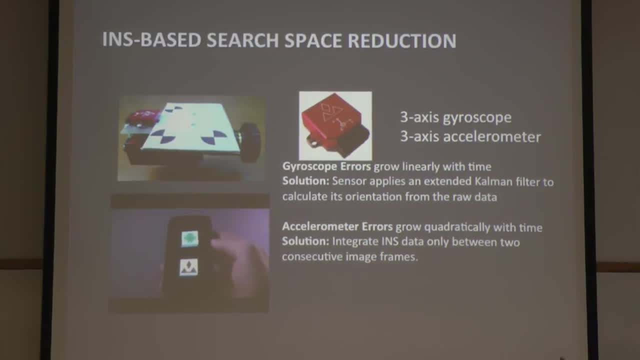 by Ralph Hollis. He uses it on BallBot, I believe, And you can see that its rotational accuracy is much more stable attached to this phone than the built-in system of the phone. Of course it costs more than the entire phone does. 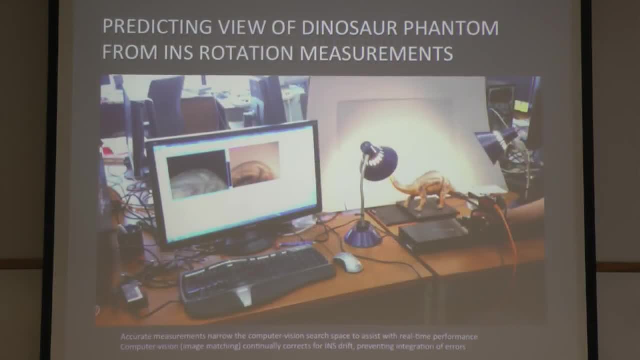 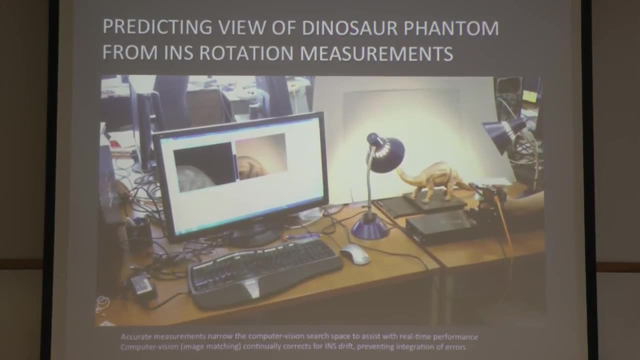 but it's much more accurate And we've demonstrated that its accuracy is sufficient to see where the image is, And we can see that we're seeing the image in the right direction relative to the model as we rotate the camera around without any other optical. 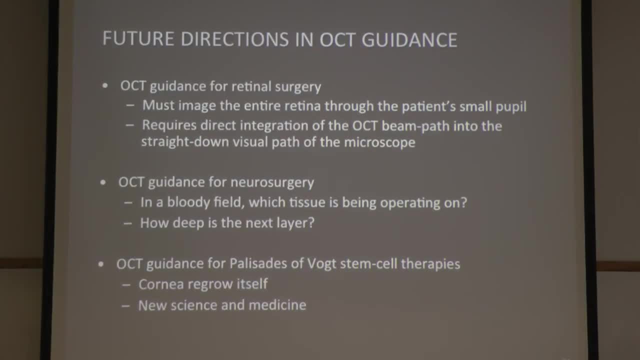 tracking going on here. So future directions for my research. There's a lot I can do with OCT guidance. I can adapt it to retinal surgery. A key difficulty there is that we need to image the retina through the small aperture of the pupil of the patient. 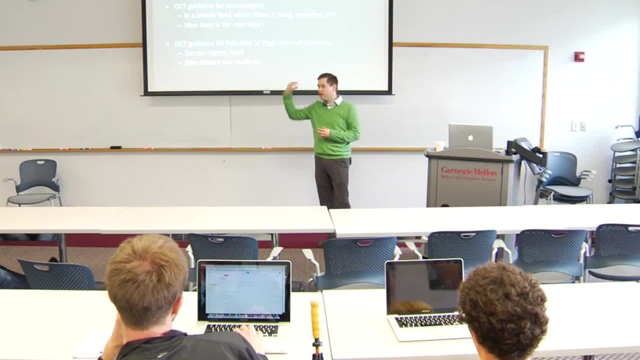 And if we had the ultrasound probe right in front of their eye, that would be easy. had the OCT scanner right in front of their eye, that would be easy. but to pull it back for the working distance, that becomes hard. We basically have to share the beam path with the microscope, which itself was going to put a tiny lens right there to get around that, so the surgeon can see through the small pupil. 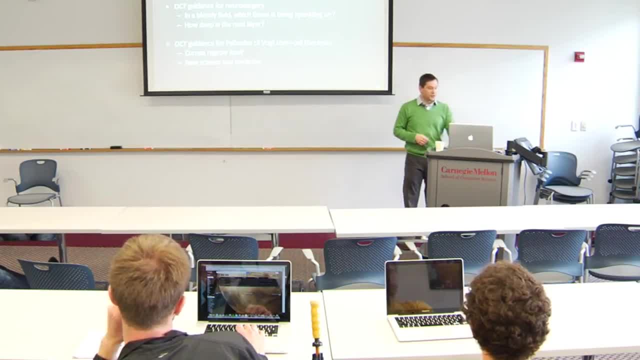 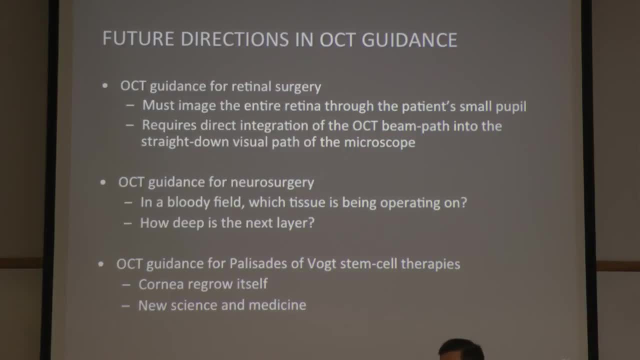 We have to integrate this much more tightly into the microscope. Several engineering issues there to address. We can also adapt the system for neurosurgery. In neurosurgery there's a bloody field. It's very hard to see what you're working on. 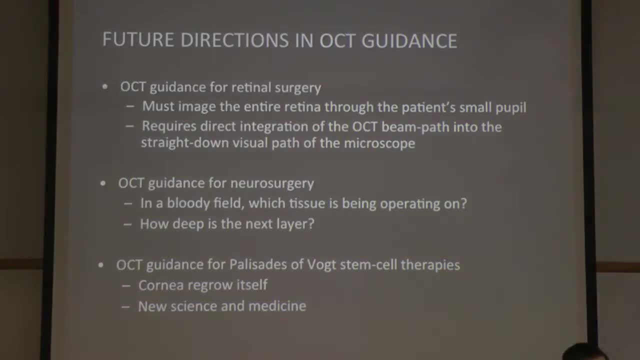 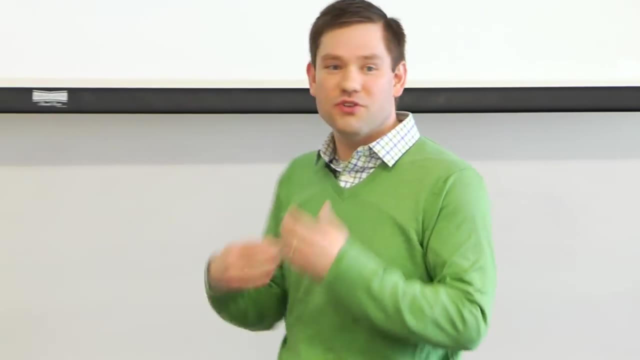 And neurosurgeons have communicated to us that it would be tremendously helpful if they could just know what tissue is there underneath this blood that I'm just about to cut into And, beyond that, if they could know how deep is it from this tissue to the next layer. that would be great as well. 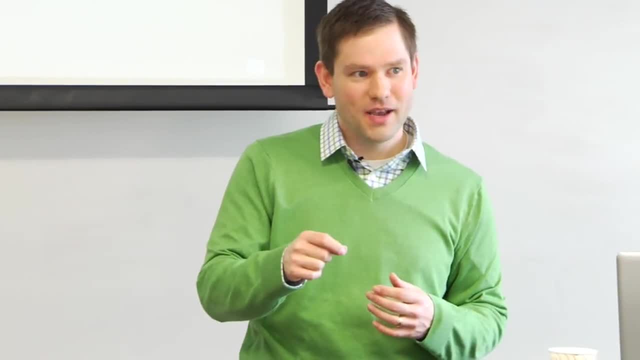 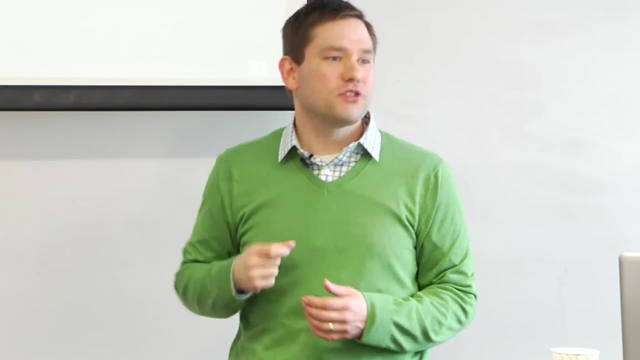 If they're trying to cut through one little piece of gray matter and they don't want to cut it all in the white matter nerve tracks that are underneath it. if they could tell: hey, I've got three millimeters here versus one millimeter, that's tremendously helpful to them. 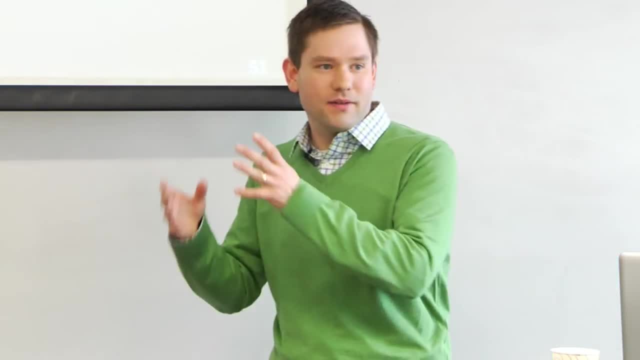 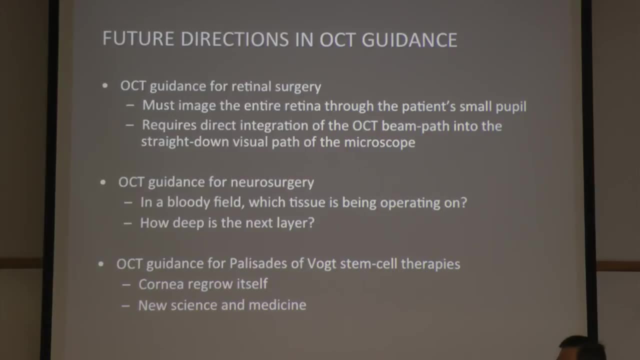 There's a system I talked about earlier for the VAT epithelial stem cell niche. a whole new application there. Likewise, there's lots of potential for collaborating with manipulators for this. There's people here- Howie, Cam and so on- and trying to take this system and combine it with manipulation tools to enable finer perception and control of what you're doing. 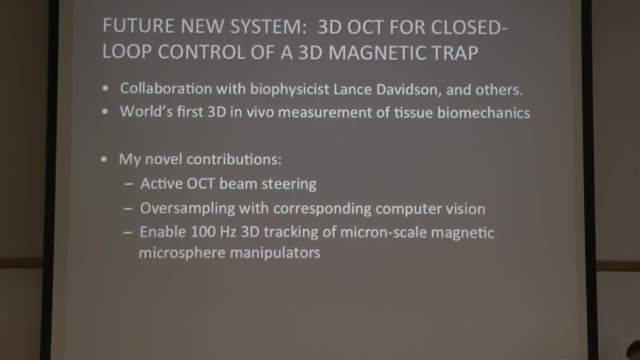 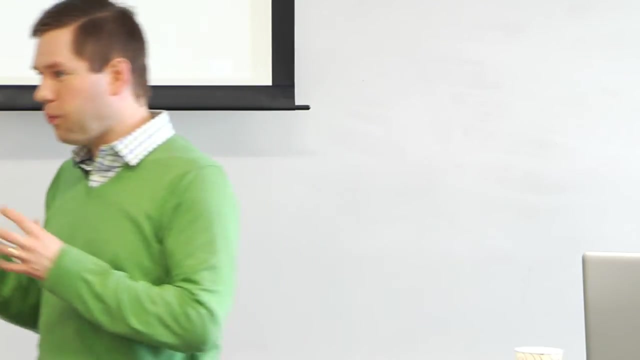 Also, I'm collaborating with a biophysicist at University of Pittsburgh to develop a new 3D magnetic trap. Basically, it uses microsphere manipulators controlled by magnetic fields, And my key contributions here are to be able to image where exactly that microsphere is in real time in 3D at 100 hertz per second. 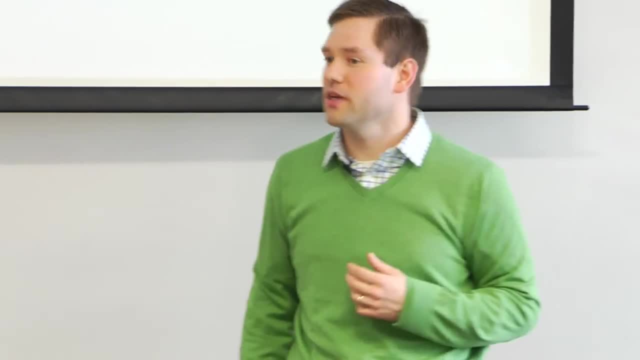 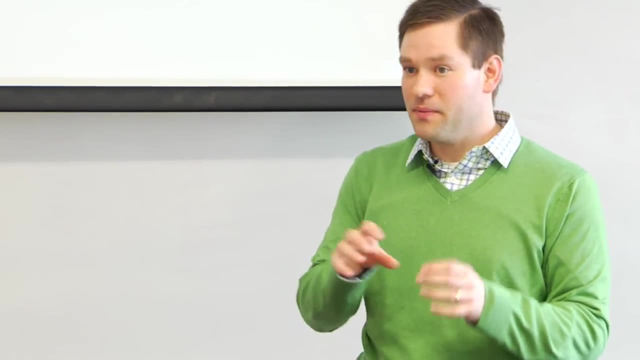 Now to do that. there's two key things that I want to do that no one's ever done before with OCT. One is to do active beam steering, so that we can image only the tiniest possible frame around the manipulator and move that in real time to track it. 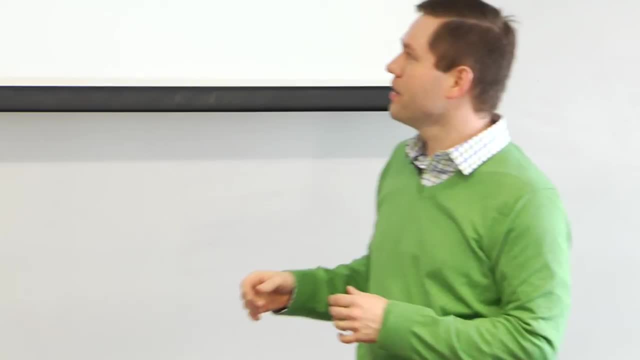 That's the only way to handle this. We have to search over a large range and we can't do that in real time otherwise. And the second is we need micron-level resolution, smaller than what the light waves of OCT will let us see. 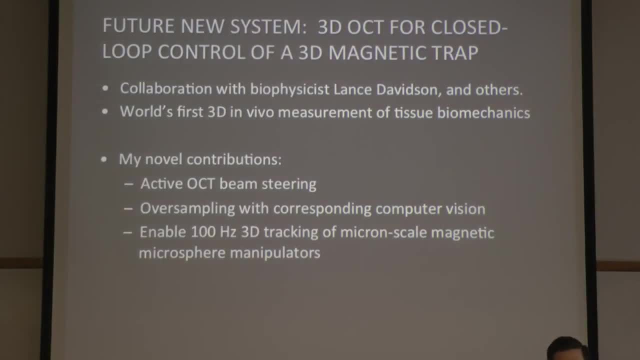 And so we're going to do some unique oversampling, taking into account prior knowledge about what that microsphere is going to look like and how we're trying to control it to be able to determine pixel resolution at spacing, even though we can't actually image it directly. 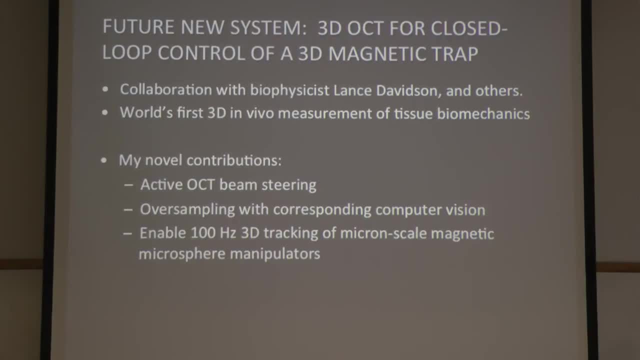 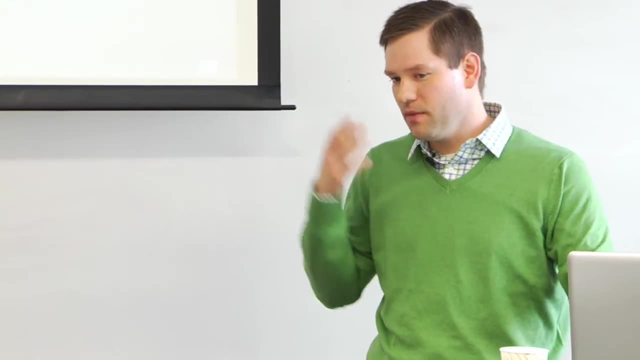 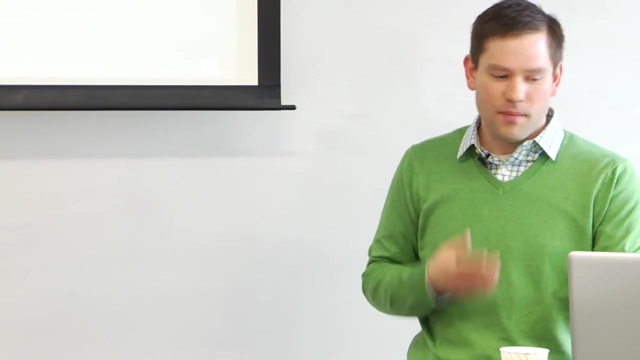 So two key contributions I'm making here to enable this entire system- And this system would allow major new contributions in a wide variety of clinical applications, ranging from detecting cancer, preventing cancer from coming back, tissue biomechanical properties, tissue engineering. a large number of collaborators lined up that would want to use this system. 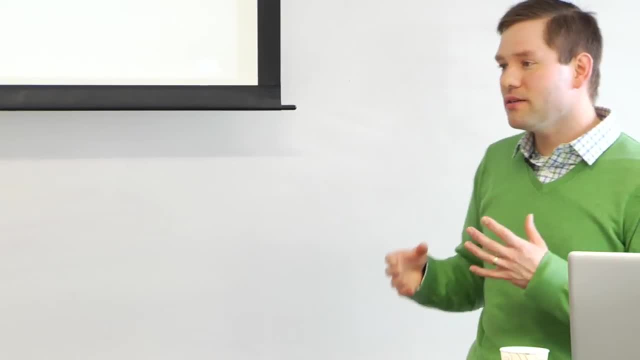 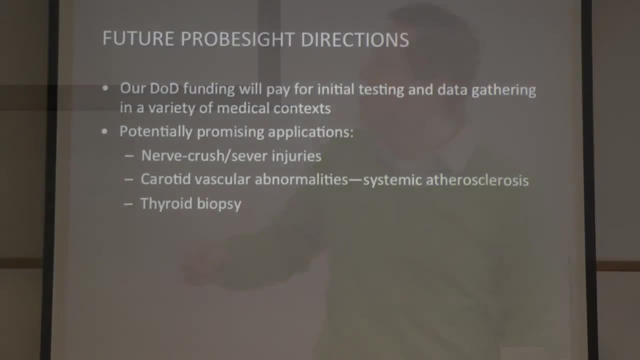 Finally, probe side. I have the DoD funding now And we're going to use that not only for the purposes there, but to gather preliminary data that would enable us to write following proposals for compelling broad-spectrum cases of nerve crush: sever injuries. 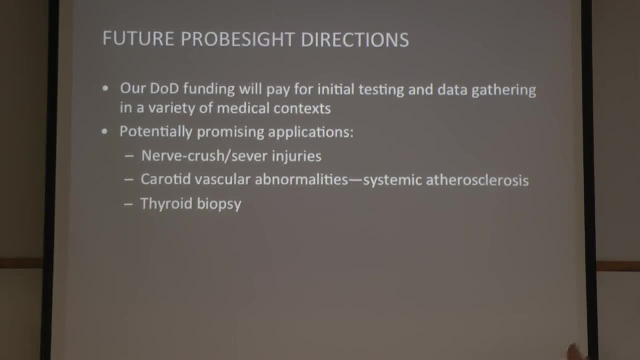 everything from carpal tunnel syndrome to paraplegics. Monitoring blood vessels could enable us to monitor systemic apheliosclerosis for a wide variety of patients that have heart disease. trying to image the neck and figure out again as the plaque is thickening, where exactly are those measurements taking? similar to the entomol thickness. 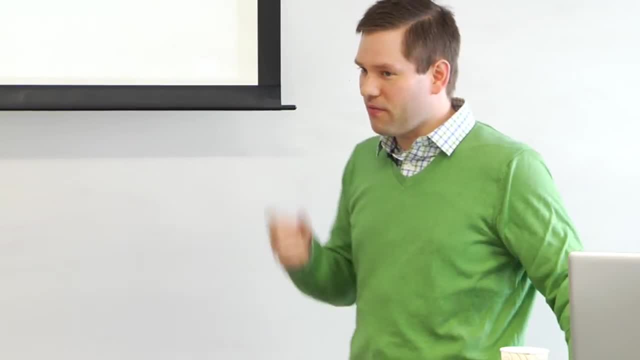 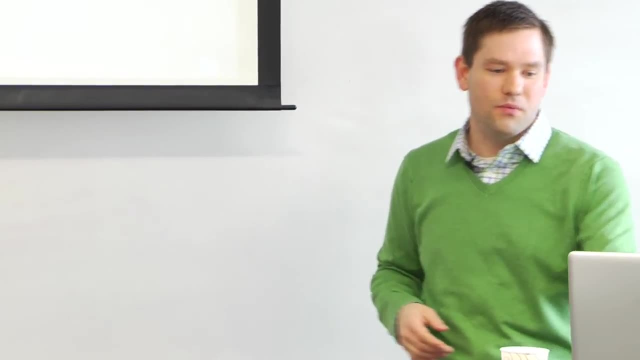 but at a much larger scale. And thyroid biopsy, where you have lots of tiny structures you need to avoid that are integral to and right beside the thyroid and others that we need to hit. And those are just three examples of a great many we could do. 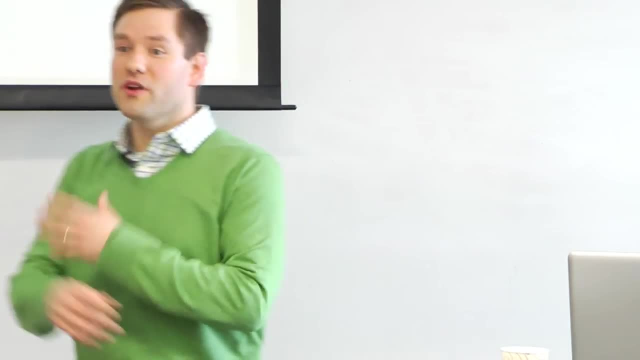 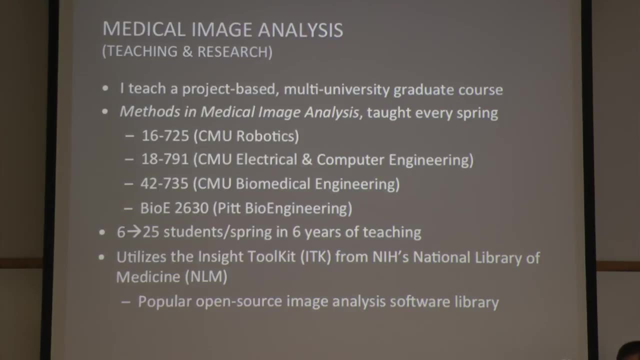 I also teach a course in medical robotics. It's cross-listed in four different departments across two universities. The course has grown from about six students when I first started teaching it about six years ago to 25 students each semester now, and I always have a waiting list of about 15 students trying to get in. 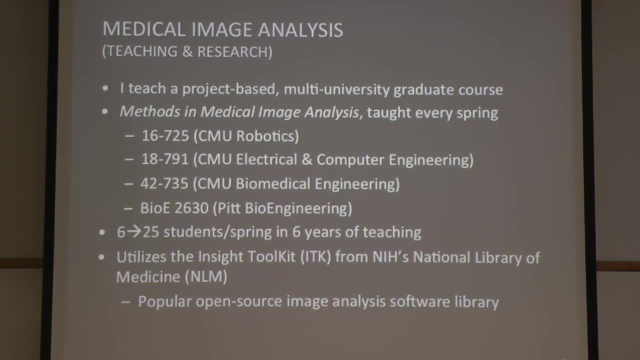 But I can't handle many more because it's project-based and I try to put substantial time into helping them all with their projects, which has been very useful for me. It's given me inroads into other faculty's labs and what they're doing. 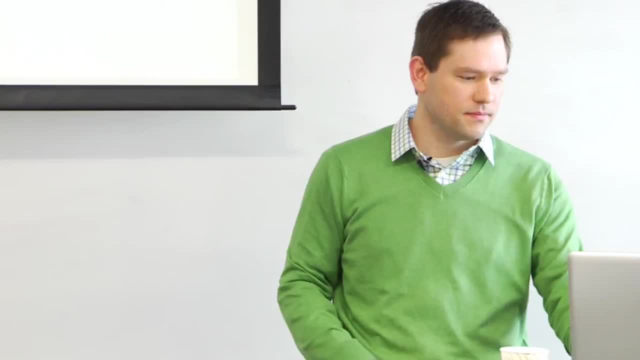 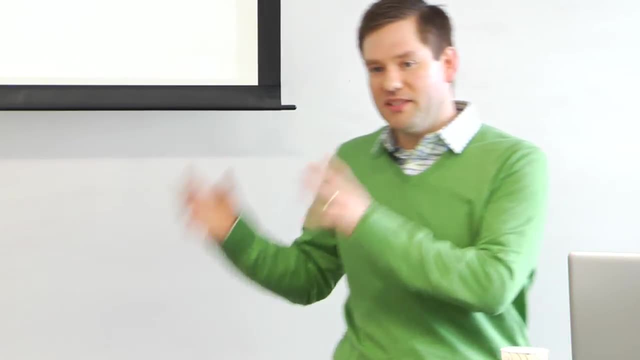 and put me in touch with clinicians and new work that they're doing as well. I've also received funding from the National Library of Medicine to further develop my course materials and to integrate ITK, the image analysis library I work with, which I've also had funding to help develop. 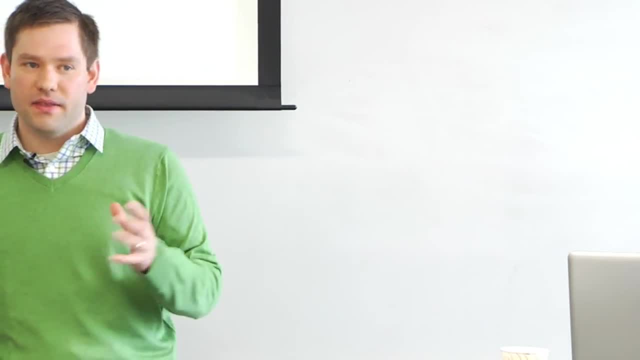 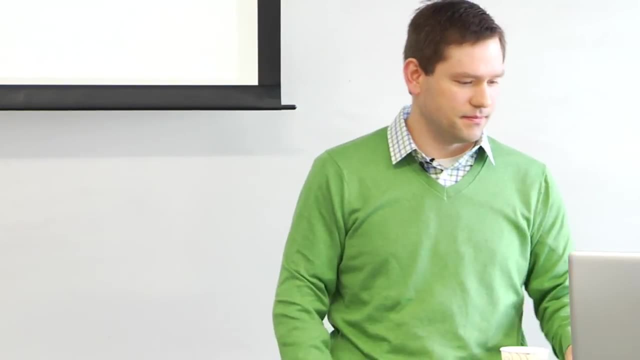 with OpenCV, the traditional computer vision library, And this work of integrating traditional computer vision with traditional medical image analysis in a real-time context has laid an excellent foundation for my work with ProbeSight. I also get funding from ECE to help pay for teaching that. 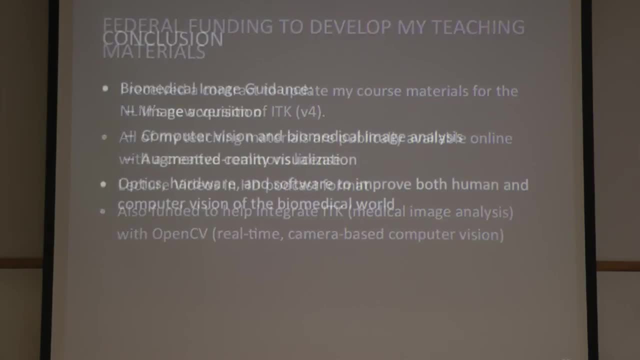 So yes, said that. So, in conclusion, I do my biomedical image guidance. This includes image acquisition, this includes the augmented reality, visualization of it and the computer vision and image analysis that happens in the middle to make all of this a reality. 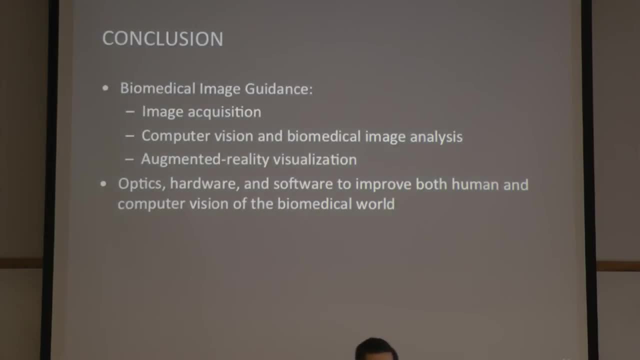 I work with hardware, optics, software and so on to build these systems so that in the end, I'm making fundamental improvements to the vision of both humans and of machines as they try to understand, analyze and see the biomedical world. Thank you. 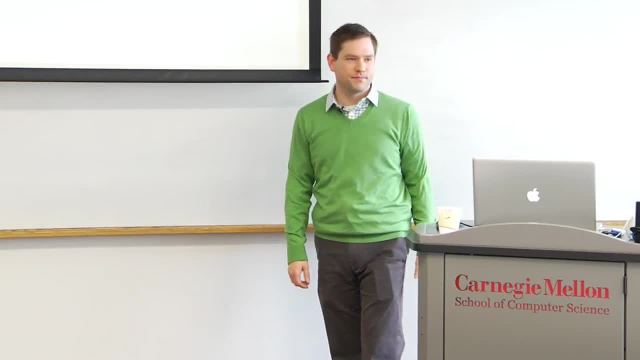 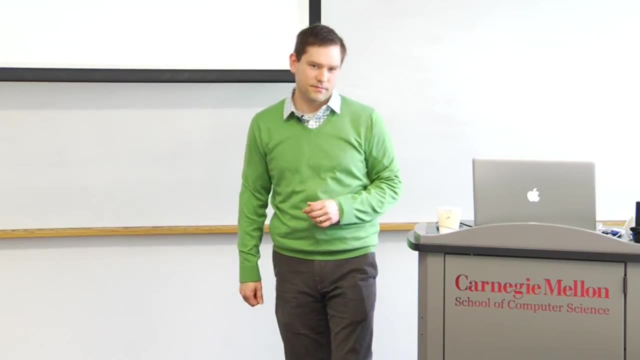 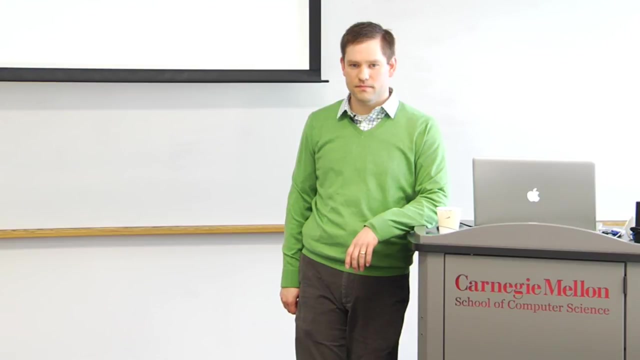 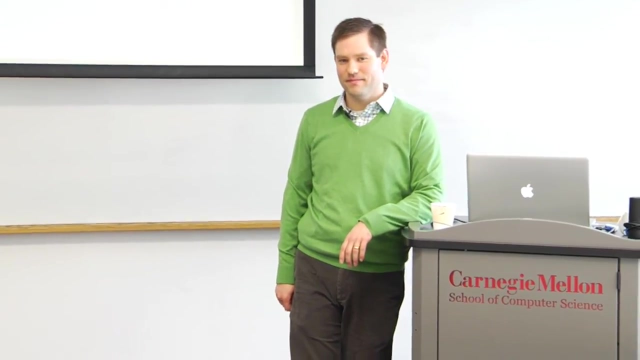 Are there any questions? Yes, Yeah, so I thought your system of visual registration on patients was interesting, but, as you pointed out, patients are squishy and they move and change, So one thing that you would have to account for is obviously the positioning of the arm. 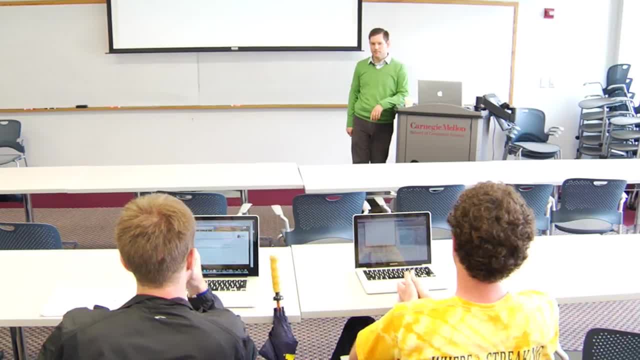 or whatever you're looking at, But also over time patients will change And oftentimes when they're on these drugs, they have a large change in body mass. So how can you account for stuff like that? That's a very good question. 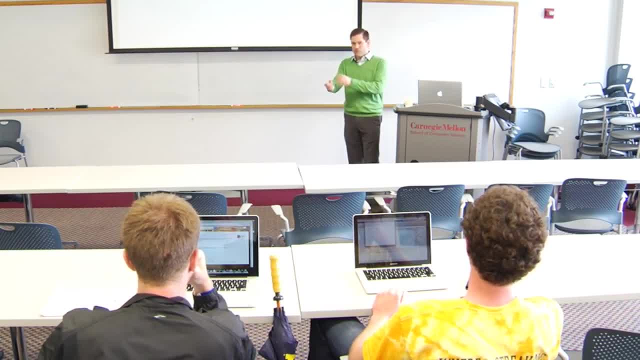 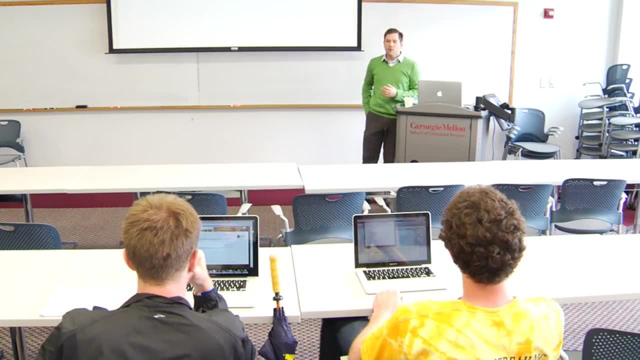 And, in fact, our application of hand transplants. when they initially do the surgery, you have tremendous swelling all around it and that slowly heals over months. So, yes, it is a hard problem And the only way to properly account for that is to be able to take the vision of the exterior. 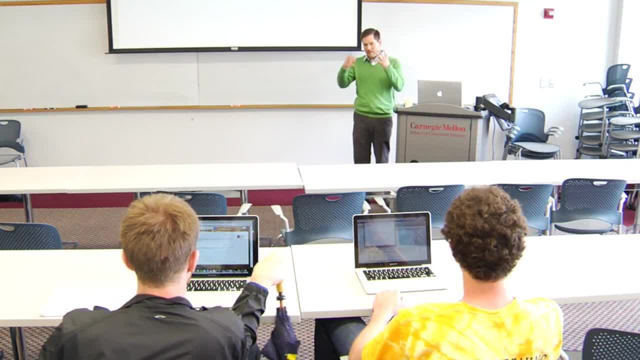 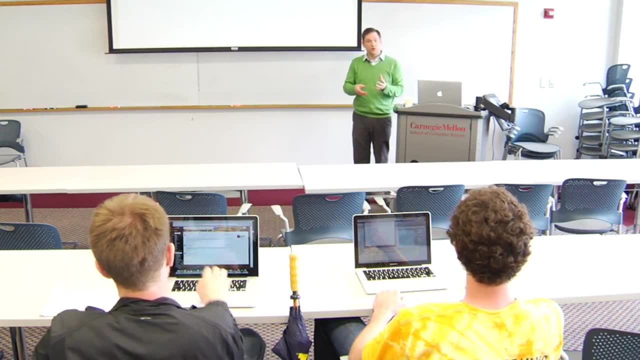 of where the probe is and the ultrasound data itself, and we actually have to analyze both of them in our 3D reconstruction. So we're seeing the exterior and the interior. Doing the 3D reconstruction as the internal anatomy is changing is an open problem. 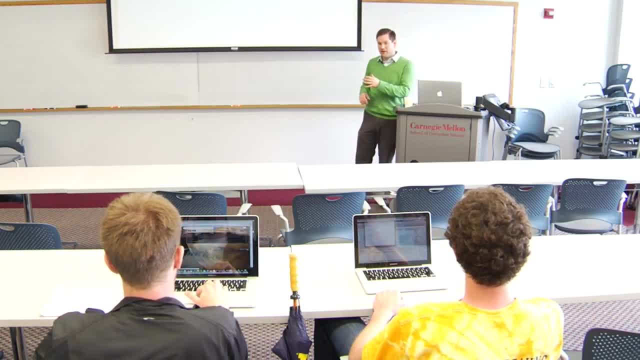 There's another PhD student I'm working with- I didn't talk about here who's working on some of the nuances of that- And we have some great ideas that I didn't want to put up in a lecture that's going to be published on YouTube. 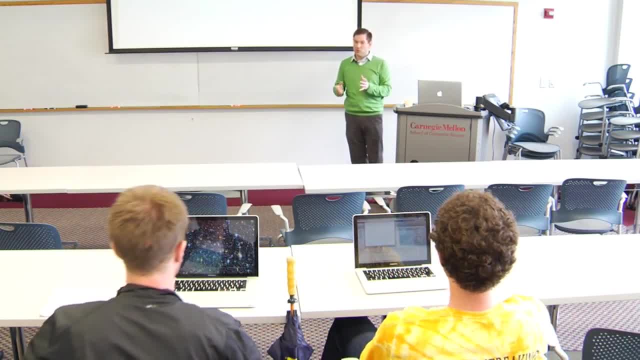 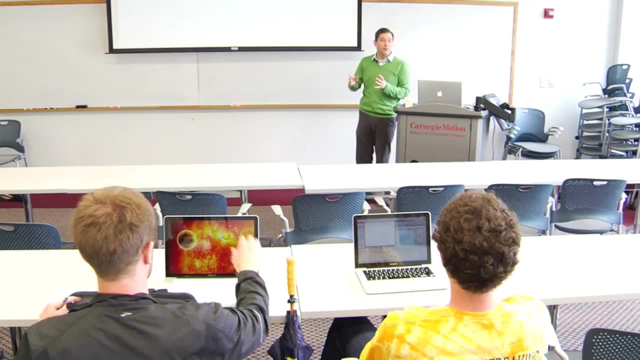 We have ideas, They're not fully proven. The degree to which they work remains to be seen. Once we get past about three to six months, I think there will be a lot less variability. We can still make major contributions if all else fails. 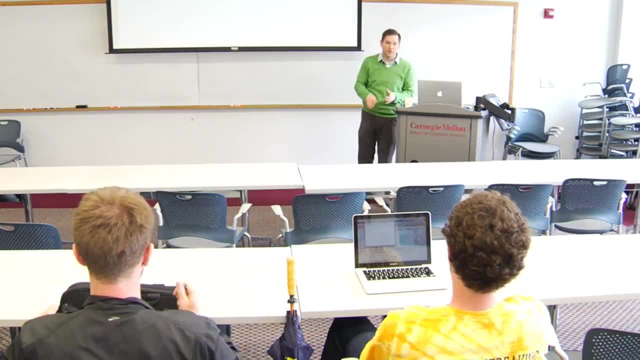 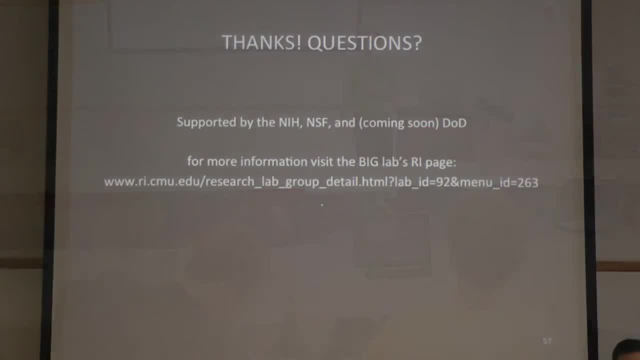 But we do have a plan in place to try to handle the severe deformation cases well, And I hope, a year from now, to be able to stand up and give a seminar about how great and wonderful all of that was. Excellent question, though Others. 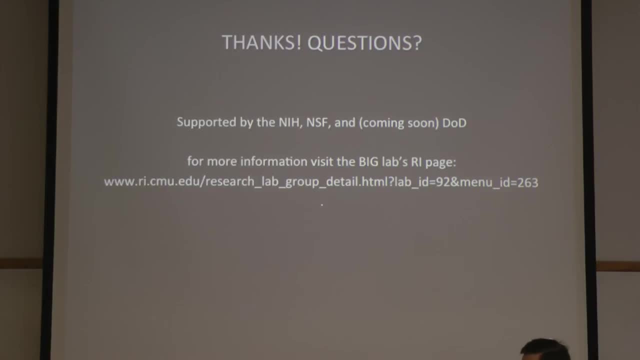 Yes, So when you showed the picture of the tilted thing, The image patch, You said there was stereopsis. that was necessary to infer that it was really tilted. In other words, we looked at it with our own eyes. However, that surprised me a little bit. 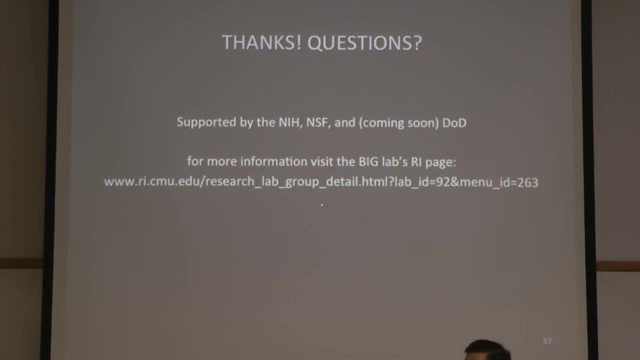 Because we hear in school that no two eyes- stereo vision- are the same thing. The truth is, one-eyed people walk around all the time with a 3D which leads you to think it's a map of eye movements or something like that. 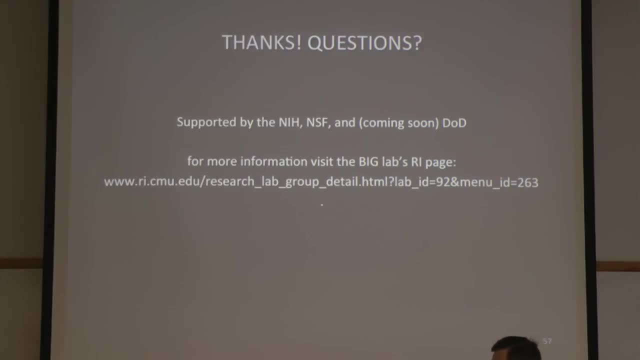 that's giving you 3D view. So what's happening there? So stereopsis is actually not the strongest depth cue. The strongest depth cue is when you see object occlusion. If I look at my hands here and I move over here. 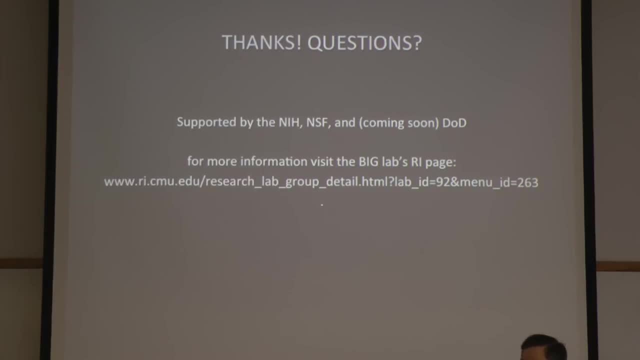 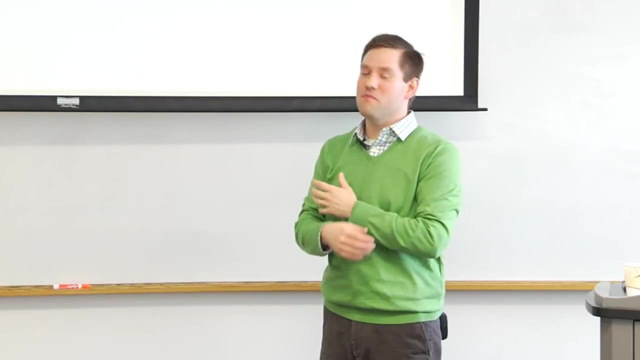 and suddenly my back hand comes in and out of field of view. that always wins. If you see that happening, your brain will absolutely infer that this one object is in front of the other one because it occludes it Right If you have other depth cues at conflict. 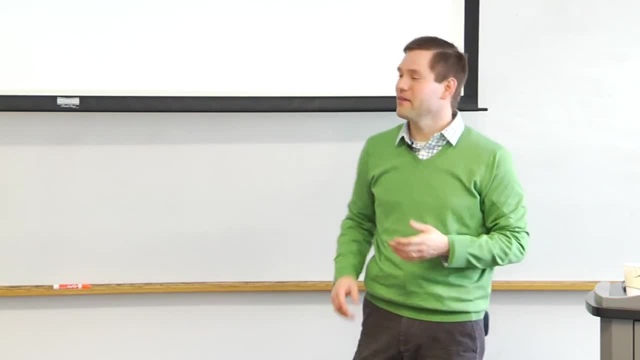 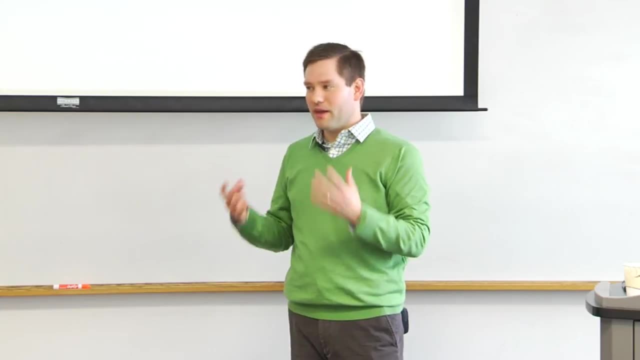 you can get tremendous headaches as your brain tries to make sense of what it's saying if you deliberately distort reality. But that's the number one cue. Secondary cues, motion is always tremendously important And then, going from that, lesser things, The pectoral cues, are important. 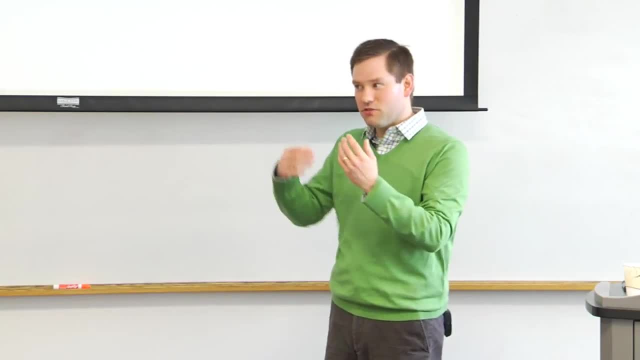 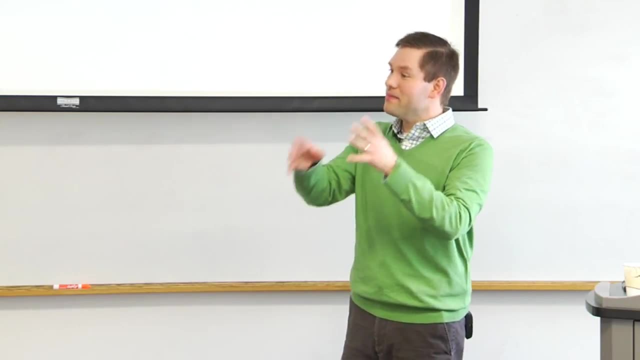 Focal distance is important In life. focal distance isn't usually as important under a microscope It's much more important, And so on. So the key is that some of the cues that are really important but misleading under the microscope, we can try to suppress those so that the stereopsis